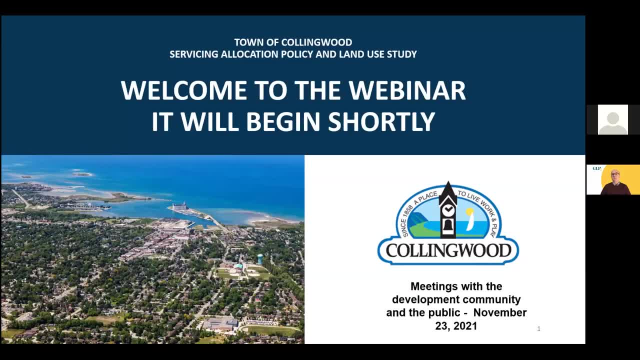 Lives to contribute constructively to matters of civic and community interest are always deserving of our gratitude and respect. So thank you again for joining us and I look forward to a very constructive and productive and informative session, and I'm sure you do as well. Let me 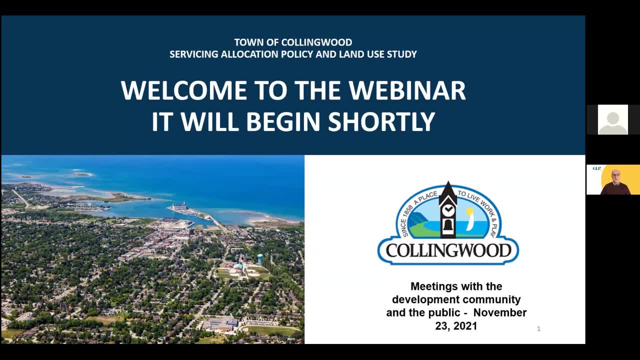 introduce myself For those of you whom I've not yet met. my name is Glenn Pace. I'm the head of a firm called GLPI and it's my pleasure to serve as the independent facilitator for the meeting. So again, it might be important for you to know that I am not a Town of Collingwood staff person. 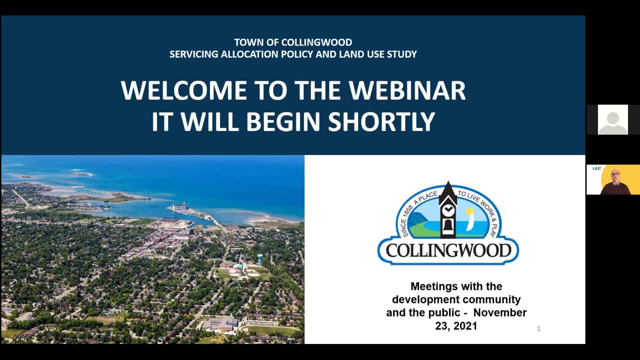 I am not an employee of any planning or engineering firms that have been retained to work on this initiative. My role is simply to moderate the meeting, and the only bias I bring to the meeting- if I can call it a bias- is toward achieving the best result for us all. 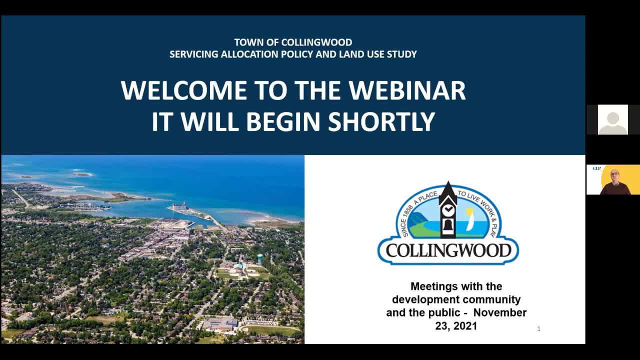 And that's what I will set out to do Now. as you may know, there are two sessions being held today. One is ostensibly for developers, and that's this one, the one starting at three o'clock, and there'll be another that's more designed for the general public and that will be taking 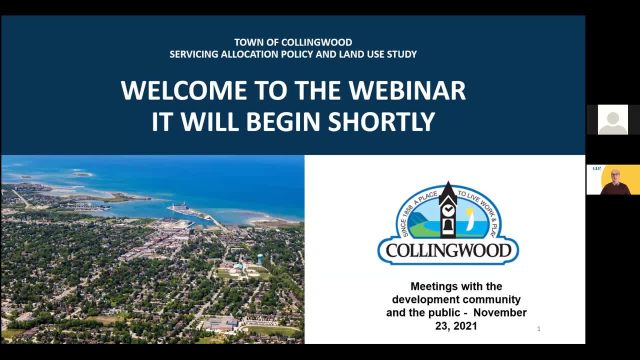 place this evening. I will note, though, that the Town, in the interest of openness and transparency, has made the links for both meetings available to everyone, So there may be some members of the public at this meeting and, of course, some developers, and 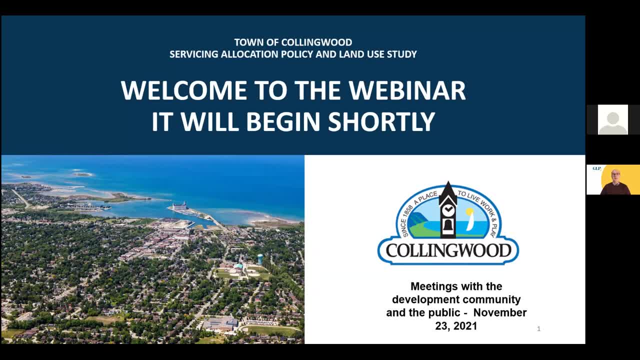 or their representatives may be at tonight's meeting, And I'll just note, though, to any members of the general public, that, again, this session will be primarily focused on the development community. Now, before we go any further, let me share a respectful land acknowledgement. 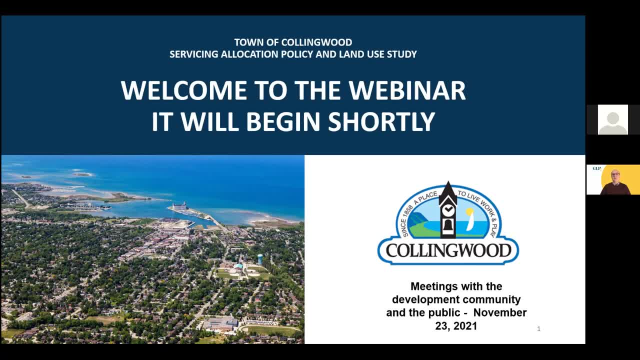 For more than 15,000 years, the First Nations walked upon and cared for the lands we now call home: Anishinabek, Haudenosaunee, Ojibwe and many others who were families, friends and communities the way we are today. The Town of Collingwood acknowledges. 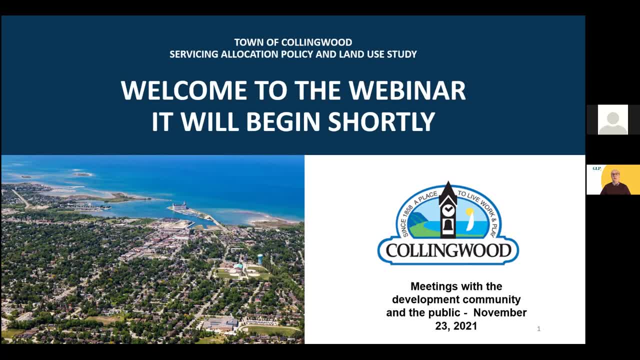 the Lake Simcoe-Nadawasaga Treaty of 1818 and the relationship it establishes with the original inhabitants of Turtle Island. We acknowledge the reality of our shared history and the current contributions of Indigenous people within our community. We seek to continue empowering. 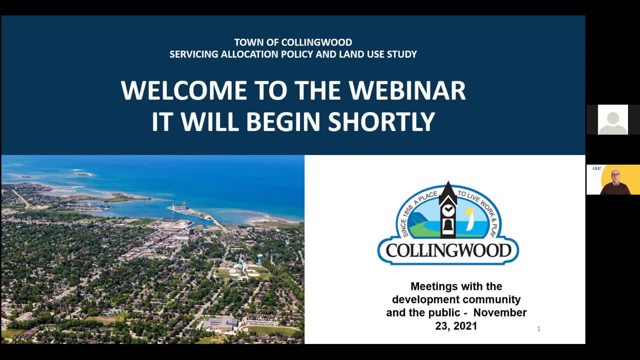 expressions of pride amongst all of the diverse stakeholders in this area, And we seek to do better and to continue to recognize, learn and grow in friendship and community nation to nation. OK, so let's talk a little bit about what it is that we are up to today. You'll hear more. 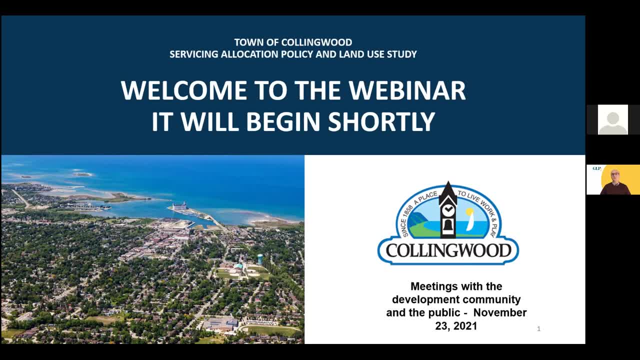 about this in a few minutes, but, as I think every everyone knows, the town passed an interim control bylaw that put a pause on certain development pending the creation of a framework for allocating water and wastewater capacity, and this session is really about sharing that draft framework and related recommendations, and, of course, it's also 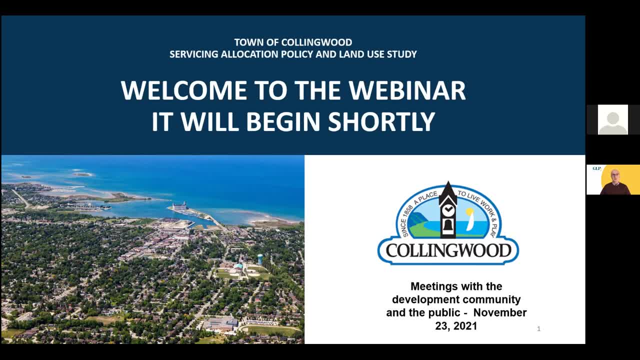 about getting your feedback, and there'll be an opportunity to ask questions of fact and clarification. In essence, the session is really focused on information sharing of one kind or another. Now, more specifically, let me walk you through the session agenda. First, we will hear from Town of Collingwood staff, who will provide a few words of welcome and some additional context. 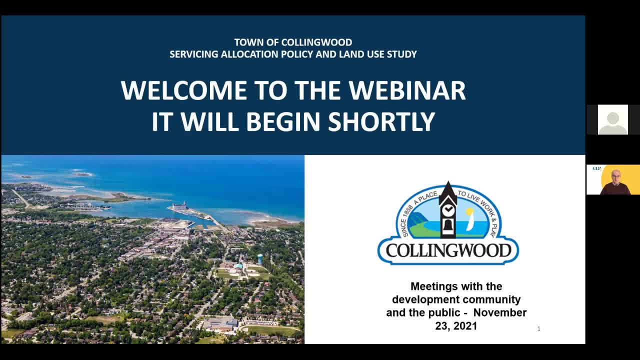 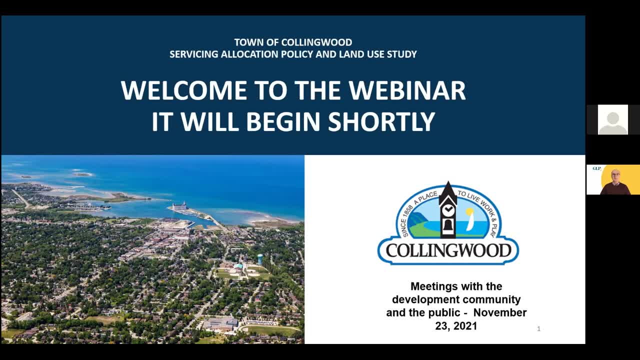 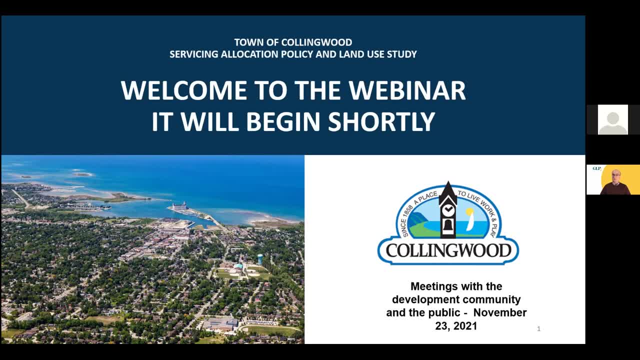 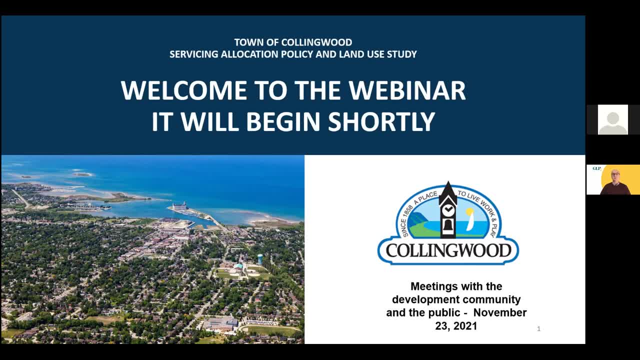 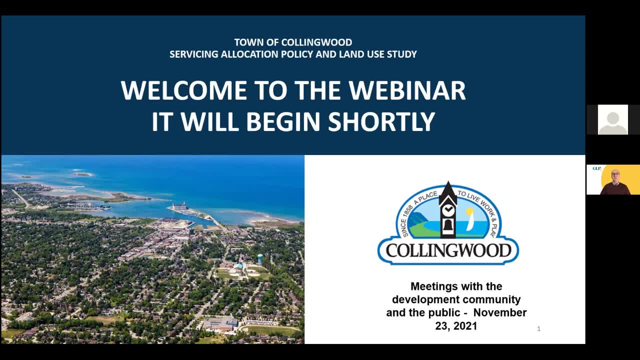 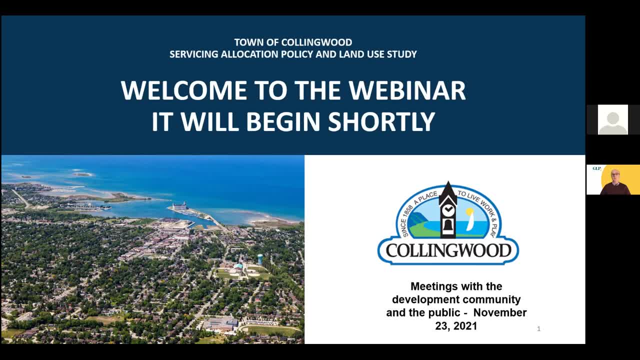 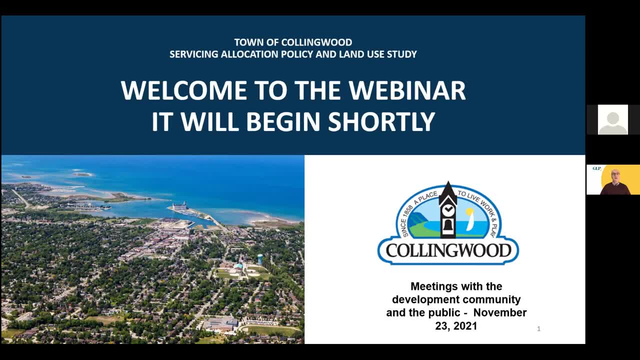 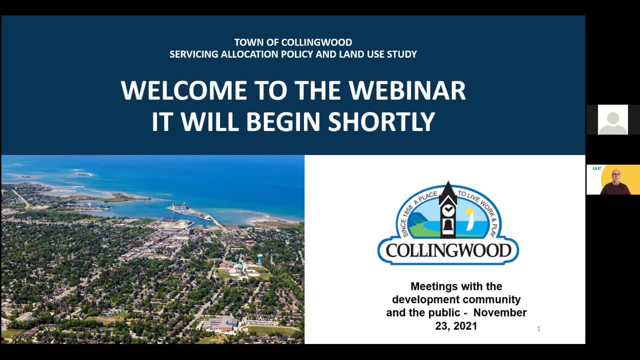 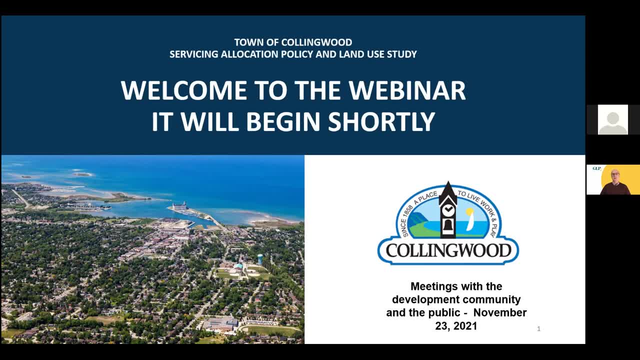 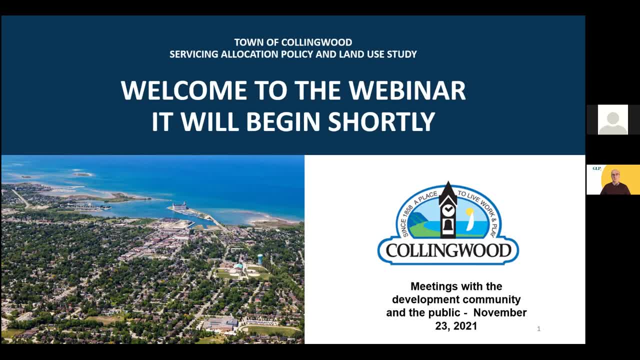 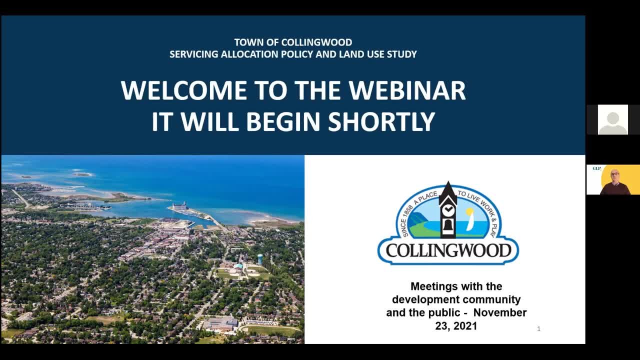 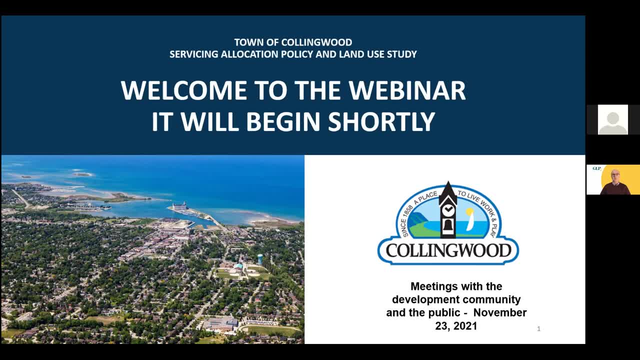 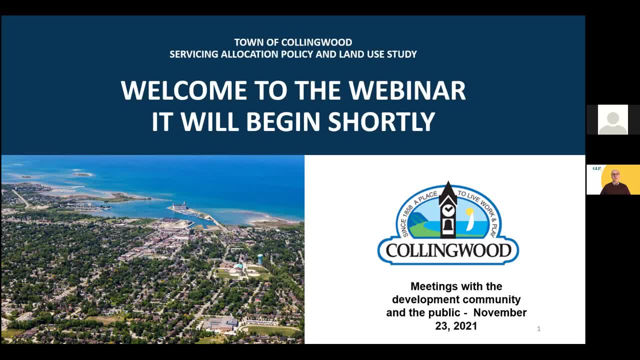 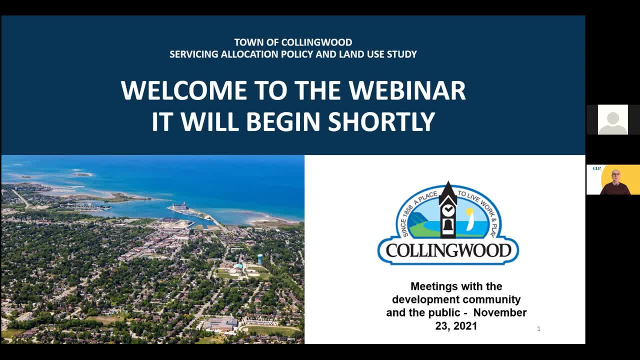 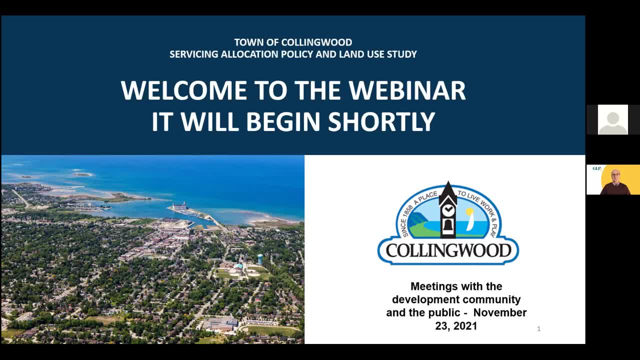 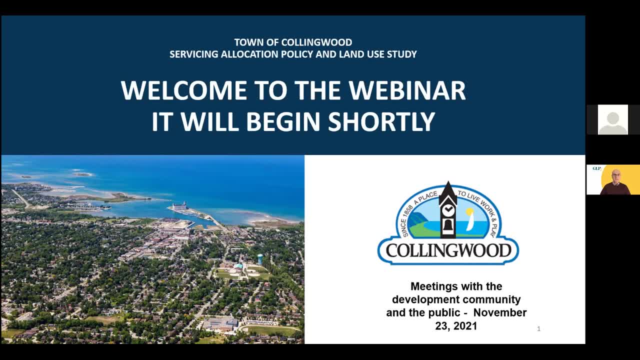 Meridian Planning Consultants- the lead firm assisting the town with the study. Meridian Planning Consultants- the lead firm assisting the town with the study. done so to potentially make the session content available to those unable to join us today, but also to have a record of the proceedings. We will occasionally make use of some electronic. 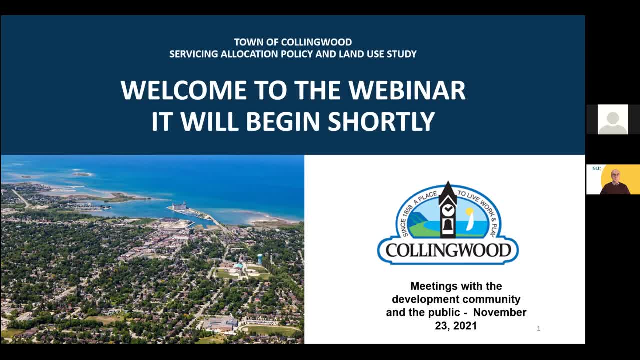 polling questions to which you are invited to respond if you have a web-enabled device. If you're joining us today using a simple, non-web-enabled phone, you will not be able to participate in the polling portion of the session. Now, I mentioned that we're looking to hear from 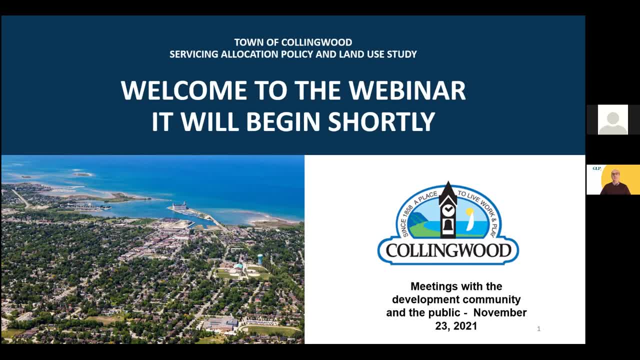 participants later in the meeting. Depending on the number of people who are interested in sharing comments and answers to the questions and posing their own questions and so forth, we may not get to everyone. Please be assured that there are other avenues for sharing your valued thoughts. 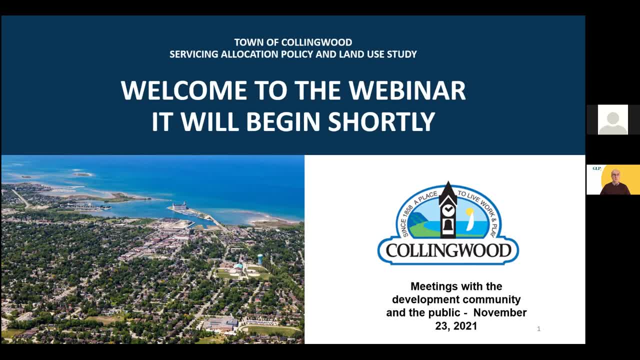 both online and otherwise. For example, you can visit engagecollingwoodca. At that site, you can access study-related information, You can share comments and so forth. You can also send them by email to planning at collingwoodca Again. 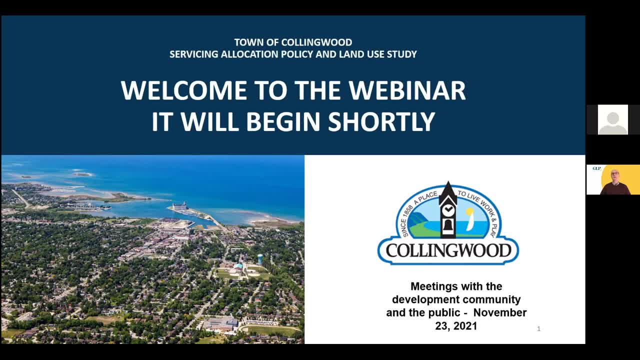 that's planning at collingwoodca. Some of this information will be on some slides later, so don't worry if you just missed what I just said. And again, comments, written comments and so forth are being accepted up until December 3rd. Now I know that the good people of Collingwood 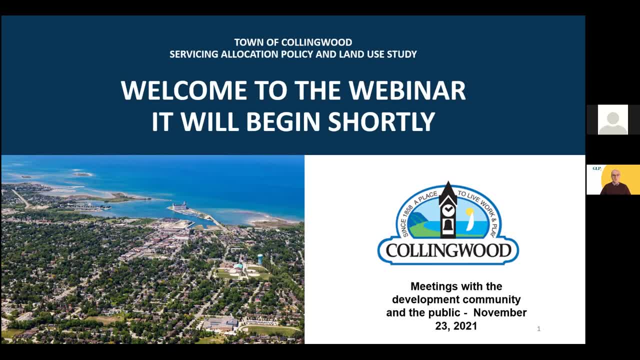 share this next sentiment, but I will just note that the mayor and council feel very strongly, as do I, about the importance of civility and respectful dialogue. So you know, to that end, of course, there'll be no tolerance for profanity or inappropriate language, And I know all of you. 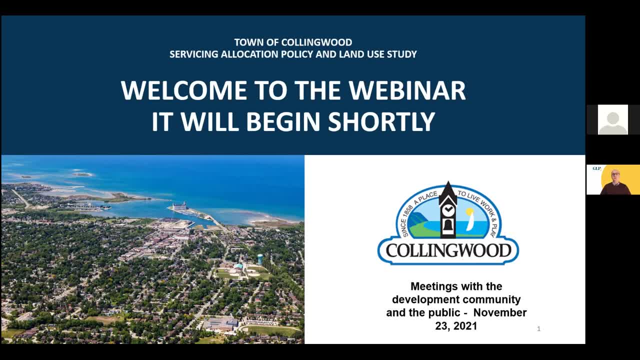 share that feeling as well, but I just needed to make mention of it so that we're all able to absolutely all on the same page about that. And, by the way, I understand that we have a number of our esteemed elected officials joining us. I'm in some senior town staff as well who are observing. 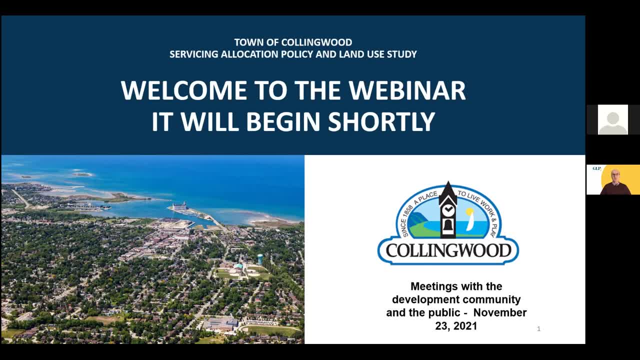 the session today. We are very pleased to have them join us. I know they will be keen listeners to the conversation and welcome to all and thank you for your interest in the initiative. So I'll say a little more about the nature of this Zoom webinar and how you can participate. 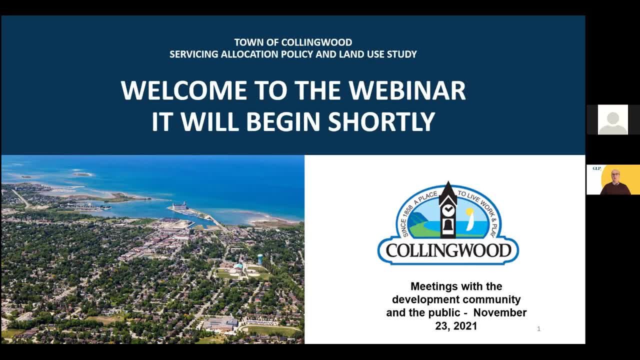 a bit later in the session when we look to open things up to your questions and comments. But, as mentioned, we'll begin by hearing from town staff who will share a few words of welcome and a little bit of additional context And to that end, it's my pleasure to hand things over to. 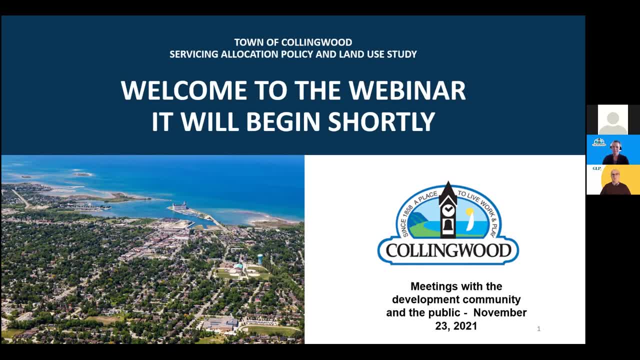 Summer Valentine, who is the Town of Collingwood's Director of Planning, Building and Economic Development. Again, welcome everybody, And Summer over to you. Thank you so much, Glen, and good afternoon to everyone joining us today. I'm relatively new at the town. I do recognize a number of names on our participant list today And welcome to those I've met and to those that I haven't met. I look forward to meeting you in the very near future. 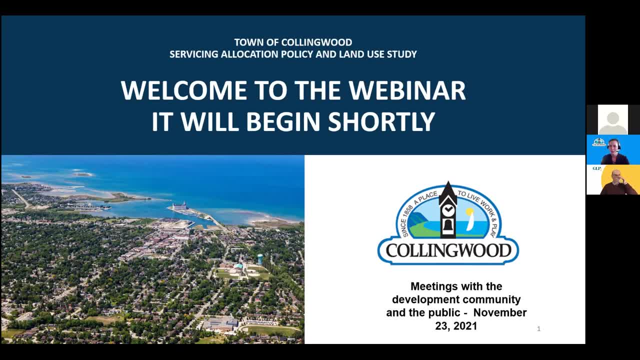 I'd certainly like to take the opportunity to express words of welcome and gratitude to everyone joining this session, and thank you for taking the time to do so. In terms of some additional context, as you all know, the City of Collingwood is a very important, very important, important part of our community, And so I'm going to turn it over to you, Glen, to what you have to say about the Town of Collingwood. 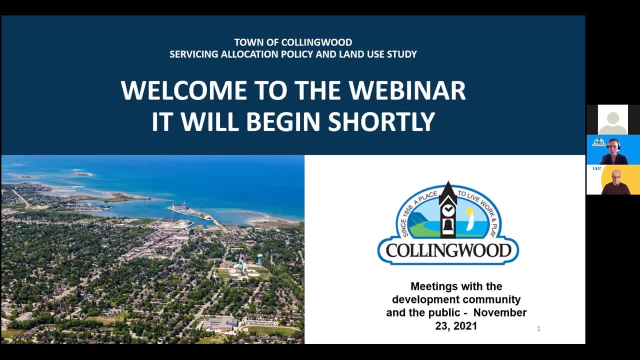 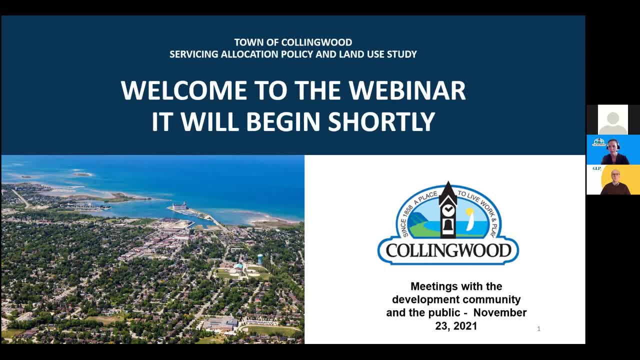 though several exemptions have been approved for shovel ready projects in 2021 and early 2022.. the bylaw is set to expire in april of next year and the town moved quickly to address issues from a land use planning perspective staff and the town's consultant, meridian planning, who's? 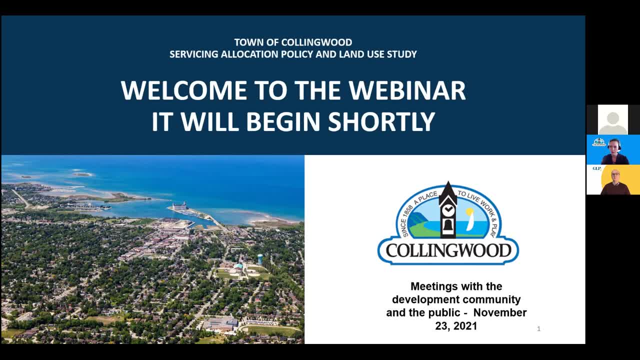 here today are working hard to complete the land use planning policy study by the end of this year to allow us time to set up an appropriate implementation framework. the study is intended to provide a fair and transparent framework for the allocation of water and wastewater capacity in a way that would achieve the community's vision and also be in line with good planning principles. 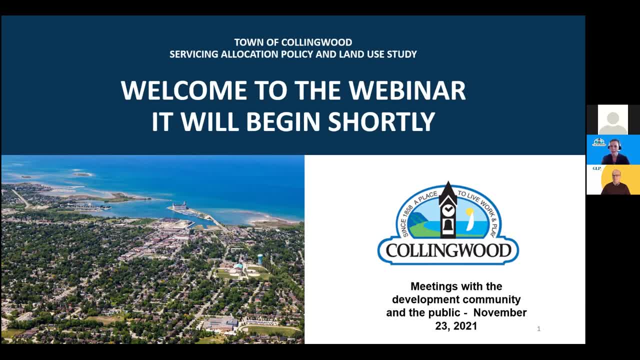 in our research meridian planning's reviewed best practices from across ontario. we'll be presenting to you today a preliminary multi-pronged policy and regulatory based framework for service and capacity allocation in the town of collingwood. i would suggest at this point it's important to 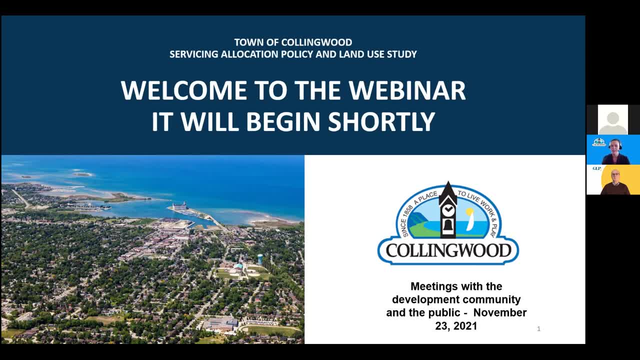 note that the combined effect of the framework which will be presented is a transition away from a first-come, first-serve approach and towards a mainstream and merit-based model of committing capacity. as glenn mentioned, this is a major project for the town and it's critical that we collectively get it right so that we can achieve a balance between: 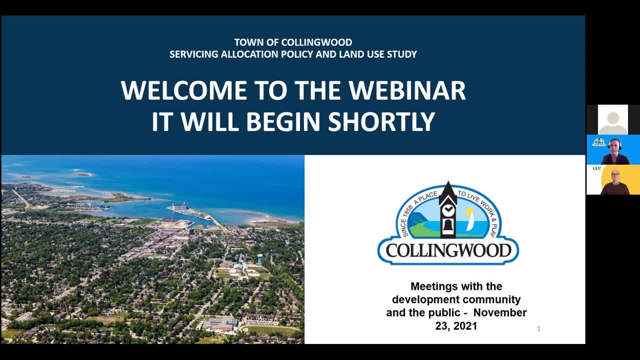 supporting appropriate growth and protecting the town's interests in ensuring that there's sufficient water and wastewater capacity available to new development and redevelopment projects in a way that fosters a complete and healthy community. so, that being said, your input on these preliminary documents and the recommendations that are going to be presented today will be provided to us in the next few days. 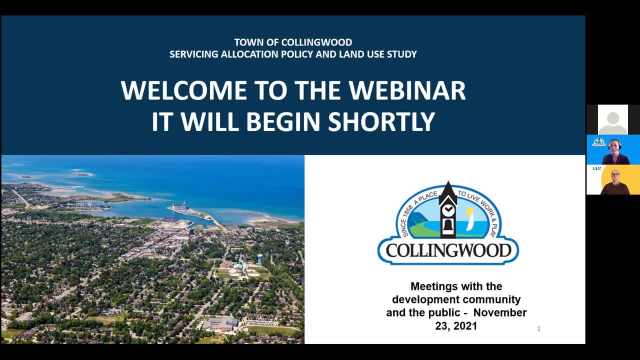 thank you, gwen. great thanks, summer. and for those of you who've just joined us in progress- and i know some people have: my name is glenn pache. i'm the head of the firm called glpi. i have the pleasure of serving as the independent facilitator for today's session. you've just been listening to summer valentine's. 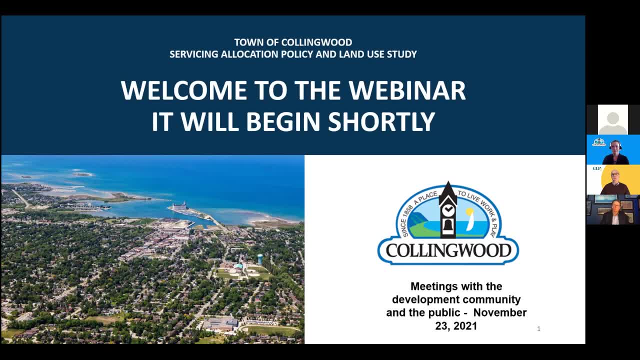 who is the town's director of planning, building and economic development. so now, as mentioned, we'll share an overview presentation covering all of the topics i mentioned earlier: background to the initiative, purpose and content of the allocation policy and what's covered and not covered by it, all of that sort of stuff. and it's my pleasure now to hand things over to nick mcdonald, who is 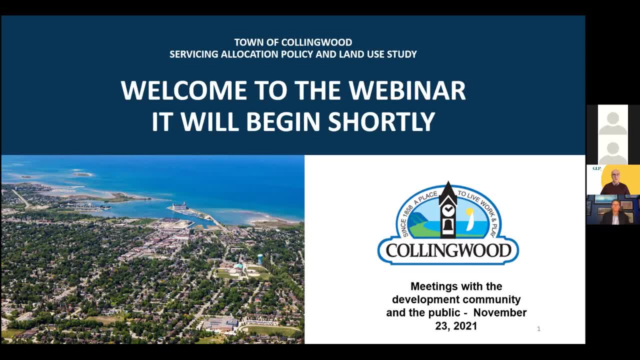 the president of meridian planning consultants, one of the firms that is assisting the town with the study. nick has some interactive polling questions that have been integrated into his presentation. he will be asking you those as well. again, they will come up throughout the presentation. however, as i mentioned earlier, those connecting through a simple non-smart phone. 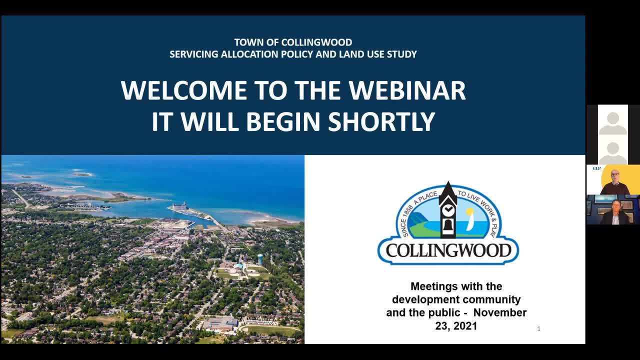 will not be able to participate in the polls part of this meeting, but you will have other opportunities later on and we'll get to those in a bit nick over to you, sir. great. thank you very much, glenn, for that introduction, and thanks very much to summer for those words of welcome as well. perhaps we can advance the slideshow. 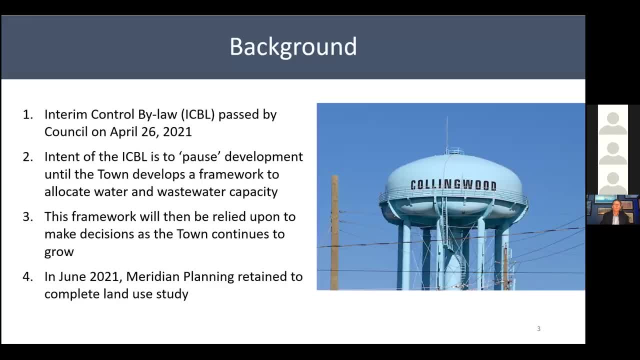 to slide three. i believe it is great. so good afternoon. so my name is nick mcdonald. i'm the president of meridian planning consultants. i'm a land use planner and a registered professional planner, and i've been working at meridian planning for over 30 years. the purpose of the session today is to present our preliminary 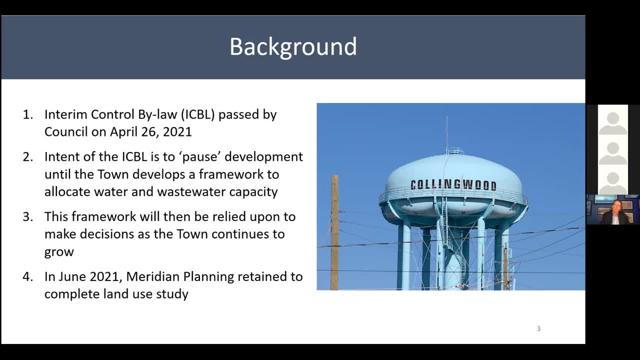 recommendations on a go forward water and wastewater allocation policy framework for the town of collingwood. our recommendations on needed changes to the zoning bylaw and optional changes to the official plan will be presented as well. i very much look forward to your comments on our preliminary recommendations. 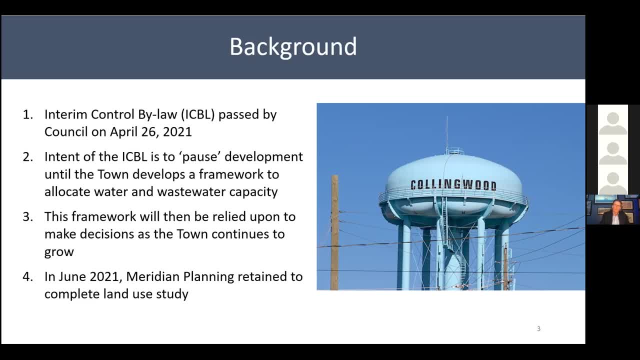 as many in this session are aware, and as mentioned by summer, valentine town council did pass an interim control bylaw on april 26th of 2021 and the intent of that interim control bylaw is to pause development until the town develops a framework to allocate water and wastewater capacity given. 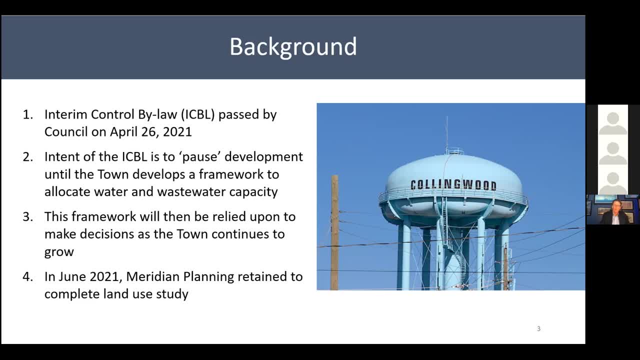 that the planning act only allows interim control bylaws to last for a one-year period. it will expire on april 27th 2022.. once the allocation framework is finalized, it will then be relied upon to make decisions. as the town continues to grow and, as many on this call are aware, considerable growth is expected in. 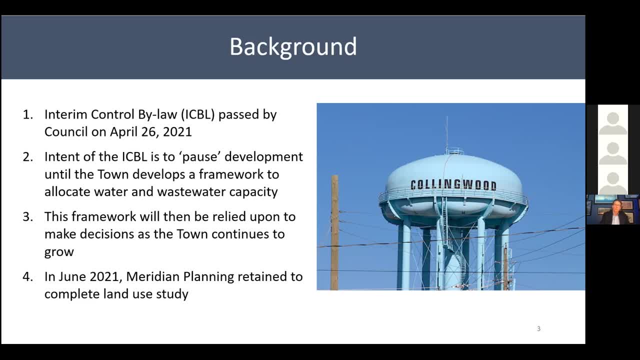 the town of collingwood to 2051.. so, in order to provide advice on the strategy itself and with other aspects of the work to be completed, my firm was retained in june 2021 to complete the plan for the next 15 years. i'm going to talk about the project's future and the potential. 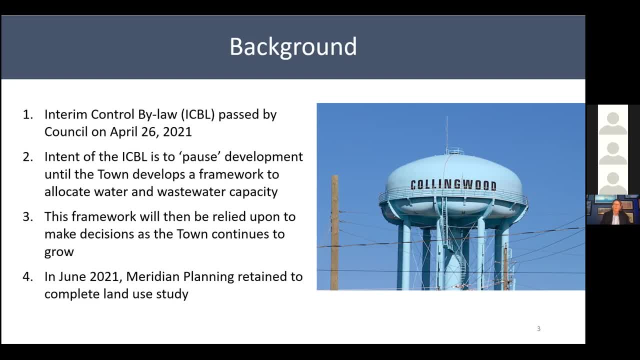 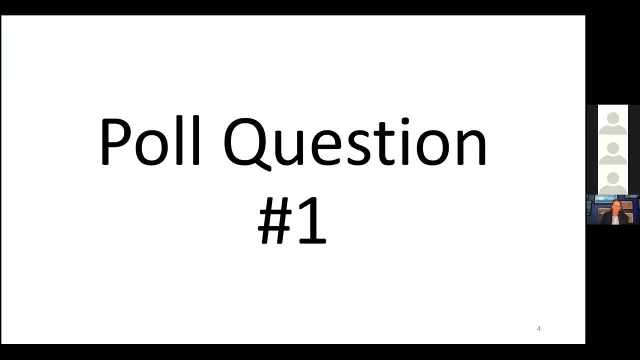 benefits of this plan to the town of collingwood in the future, as well as what the planning act will do and what the goals are for this project. the plan is set to be a very broad and comprehensive work and, as you will see in this presentation, we have made quite a bit of headway, however. so to get 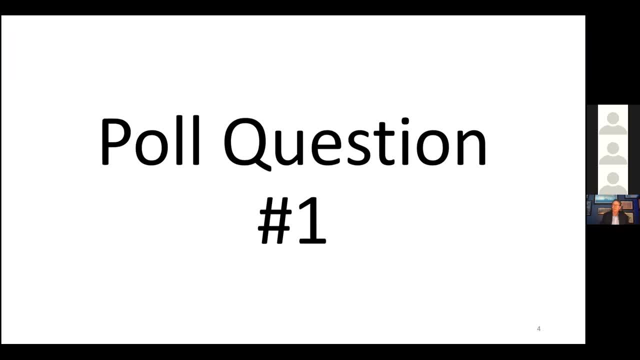 us started today and to find out who's joining us on the call. we do have a number of polling questions, with this one being the first, which i will read in the context of the town of collingwood: are you and realtor? Are you a business owner resident, a member of a stakeholder group such as the? 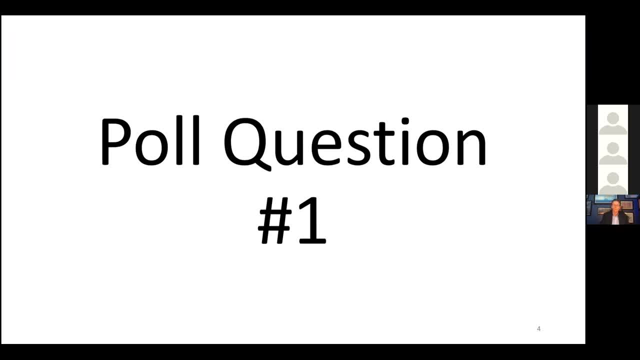 Climate Action Team or other. We always put other in these things in case there is another circumstance, And I'll wait for a few moments for folks to put in their answers. So we've got half of the people have already put their answers in, which is great. 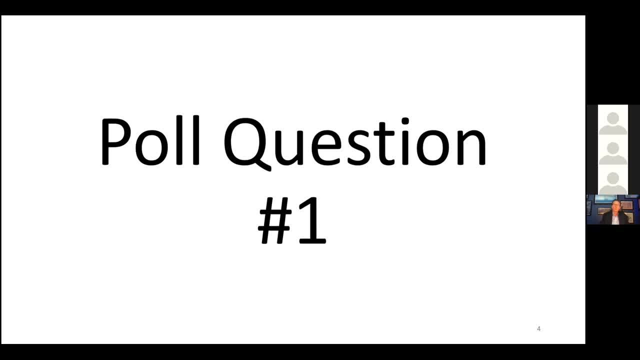 When we get close to 90,, 95%- we'll close it out. That's great. So it looks like- unless something changes at the end- that most of the participants on the call today are from the development community- 43%- or are agents or working with developers. 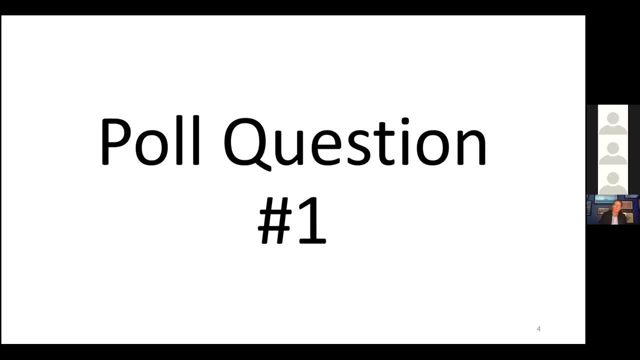 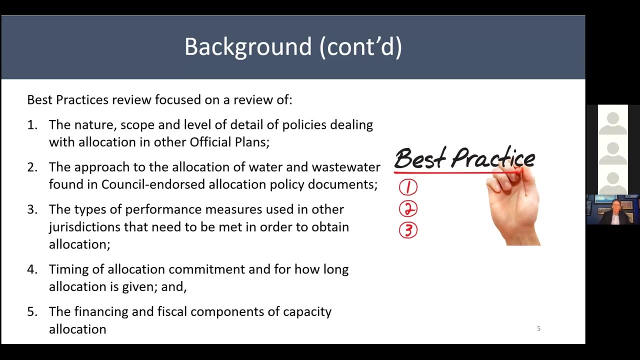 that are in the development community, So we'll close it out Another 52%. Okay, that's great. Thank you very much for joining this session today. We'll move on with the slideshow. Next slide, please. So in carrying out our work as Summer indicated, we did carry out a best practices review that. 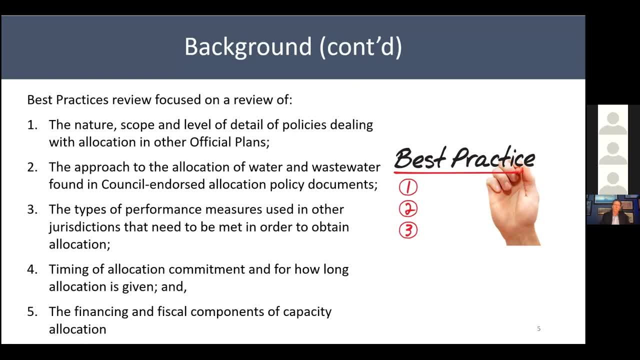 looked at how other municipalities in Ontario deal with this particular issue And in particular, we looked at the nature, scope and level of detail of policies dealing with allocation in other official plans in Ontario. We also looked at the approach to the allocation of water and 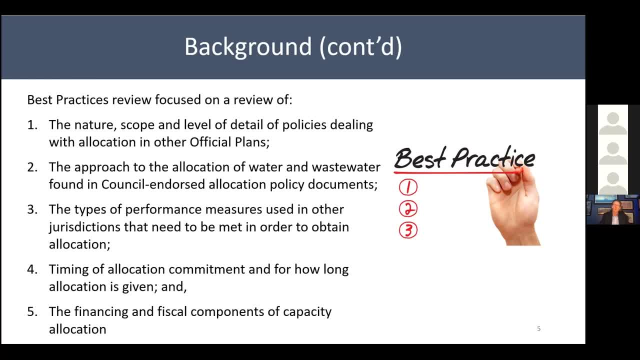 wastewater in council-endorsed allocation policy documents. And, to be clear, these policy documents sit outside of official plans and are endorsed by council, So therefore they're non-statutory. We also looked at the types of performance measures used in other jurisdictions that need to be met in order to obtain allocation. And when I say 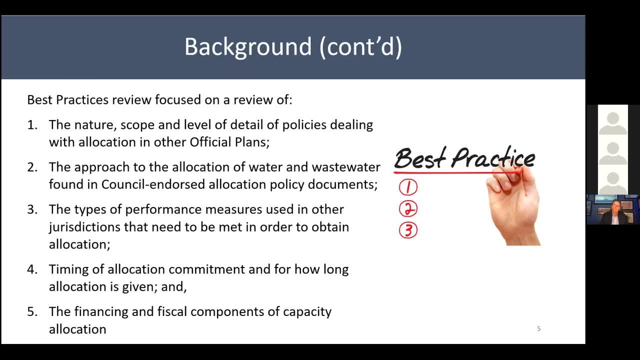 performance measures. that means what criteria need to be satisfied to obtain allocation. We also looked at the timing of allocation commitment and for how long allocation is to be given, And this is important, particularly when services are finite, as is the case in Collingwood, at least in the short term. And of course, we looked at the financing and fiscal 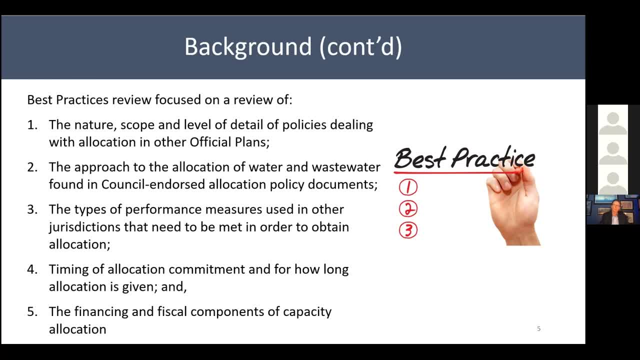 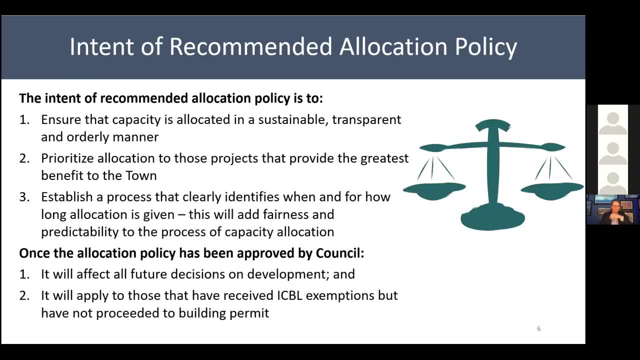 components of capacity allocation as well. Next slide, Next slide, please Thank you. So, in terms of the intent of the recommended allocation policy, it is to ensure that capacity is allocated in a sustainable, transparent and orderly manner. And when I say sustainable, 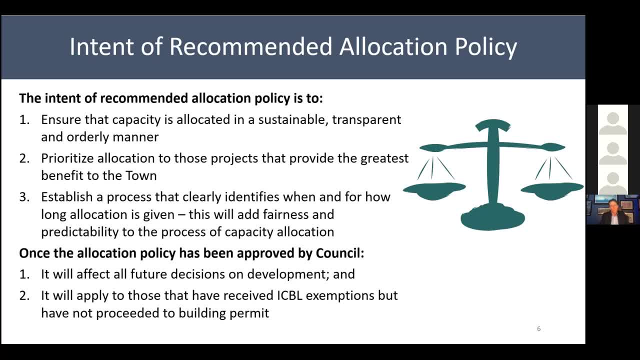 that means that resources are used widely- sorry- wisely. And when I say transparent, that means the process is known up front and applied equally to all. and when I say orderly, this means that since development has to occur in an orderly manner, so should the allocation of 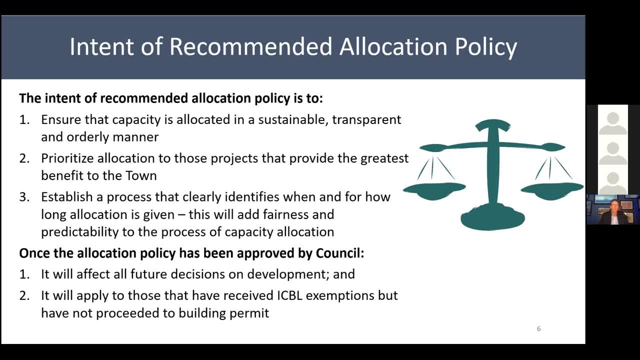 capacity. A further intent of the recommended allocation policy is to prioritize allocation to those projects that provide the greatest benefit to the town, and you will hear later in this presentation how this is proposed to occur through a merit-based system. And lastly, a further intent is to establish a process that clearly identifies when and for how long. 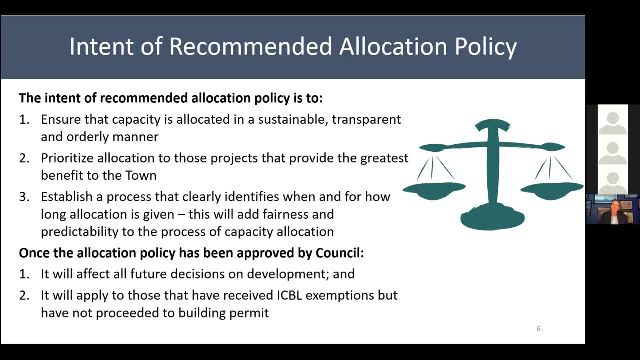 allocation is given with the goal being the addition of fairness and predictability to the process of capacity allocation and, given the finite nature of the resource, at least in the short term, this is obviously very important. Once the allocation policy has been approved by council, it will affect all future decisions on development, and I will explain what development will be. 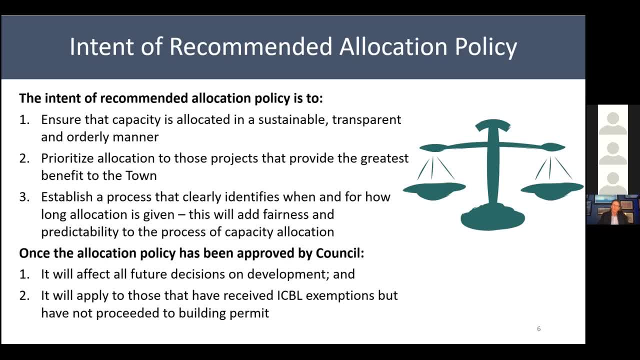 seen. The first is that the allocation policy will be subject to the policy in a moment and, secondly, it will apply to those that have received ICBL exemptions that have not proceeded to building permit. This means that those who have already received exemptions will be subject to the policy. 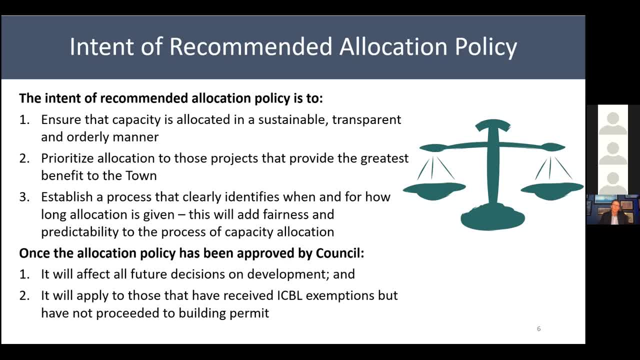 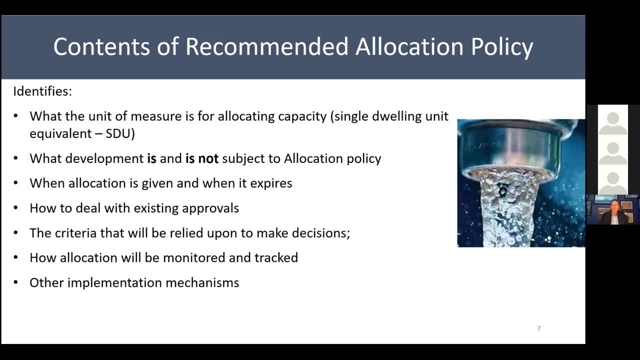 if they have not applied for and obtained a building permit when the allocation policy is adopted by council. Next slide. So this is a recommendation allocation policy. It identifies what the unit of measure is for allocating capacity and in the town of Collingwood it is an SDU, which stands for single dwelling unit. 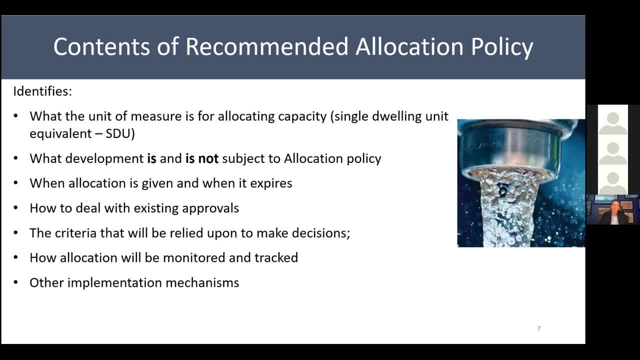 equivalent. It also indicates what development is and is not subject to the allocation policy, and this is obviously key to understanding what development can proceed without having to apply the policy. Next slide, It deals with when allocation is given and when it expires. In other words, at what point in the planning process, which often involves many decision points, should allocation be given. 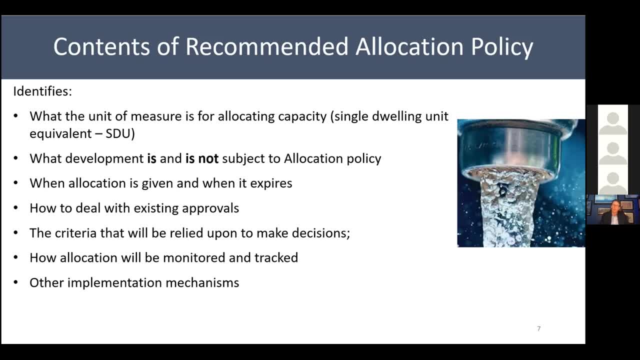 It deals with how to deal with existing approvals, Always a consideration, since existing approvals may potentially require additional municipal water and sewer services. It includes criteria that will be relied upon to make decisions, with this being a key element of the policy: How allocation will be monitored and tracked to make sure that allocation is being used wisely. 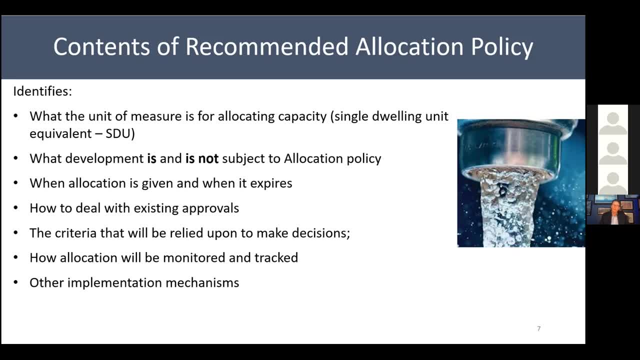 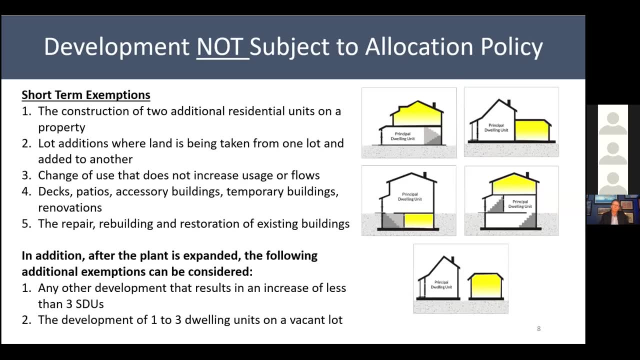 and it also deals with other implementation mechanisms that will need to be considered, such as updates to the zoning bylaw, for example. Next slide: So this slide identifies proposed short-term and long-term exemptions to the draft policy framework. So the short-term exemptions are the construction of two. 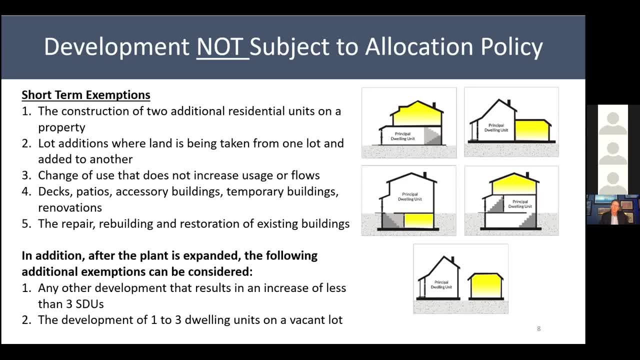 additional residential units on a property, and additional residential units is the term the province uses to describe what others may know as basement apartments or secondary suites. It would not apply to lot additions, where land is being taken from one lot and added to another. While this rarely occurs, it does happen and we want to make sure we think. 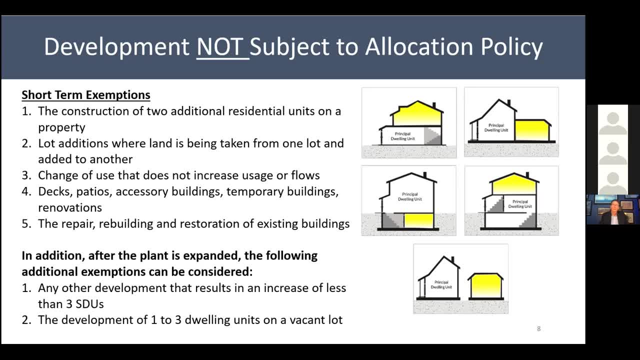 about every type of application going forward. It will not apply to to changes of use that do not increase usage or flows, and examples, of course, may include going from an office to a retail store, but it would not include, for example, and office going to a restaurant, for obvious reasons. 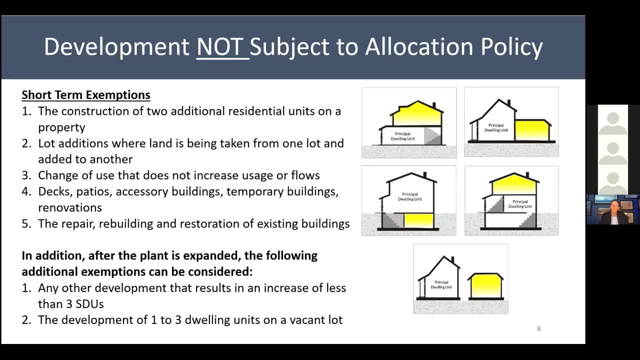 Decks, patios, accessory buildings, temporary buildings or renovations would also be exempt, which they are currently in the an interim control bylaw. and, of course, the repair, rebuilding and restoration of existing buildings would also be exempt, which is also again already exempted by. 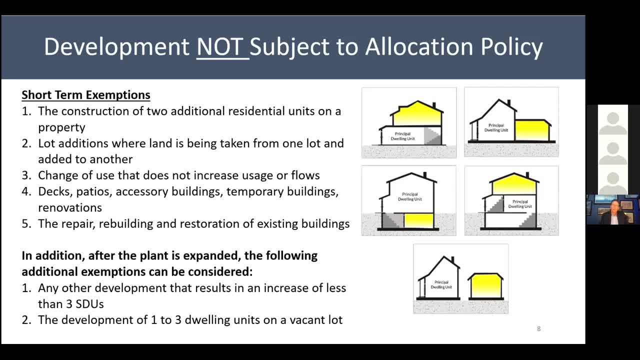 the interim control bylaw as well. In addition, after the plant is expanded- and when I say the plant, it's the water plant itself- the following additional exemptions could be considered, and they include any other development that results in an increase of less than three SDUs and or the: 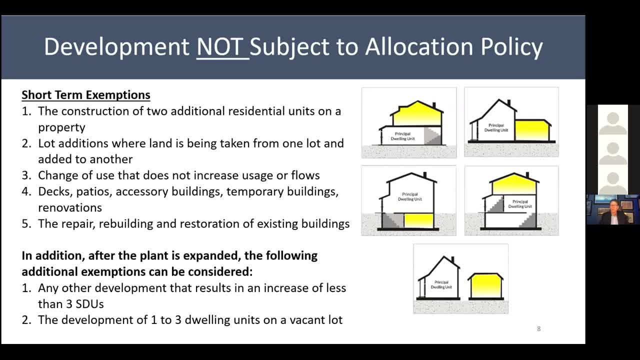 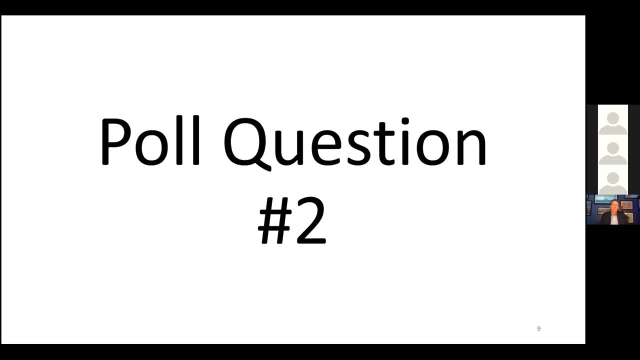 development of one to three dwelling units on a vacant lot. Other exemptions could also be identified. So this brings us to our second polling question, question two, which I will read: To what extent do you agree that an exemption should apply for up to two secondary residential? 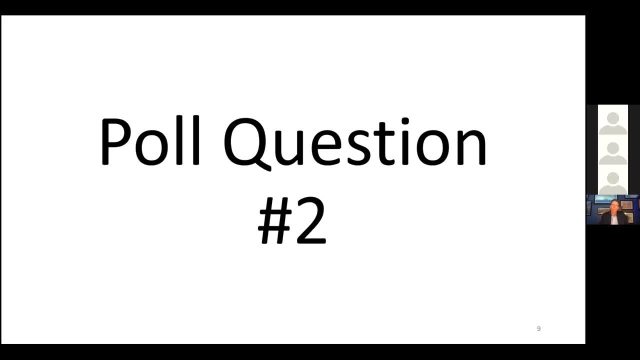 units and, for example, accessory apartment, coach house, accessory dwelling unit on a property, And then the choices are strongly agreed, Agree, agree, neutral, disagree, strongly agree and don't know. And I'll wait a couple of seconds for folks to put in their answers. 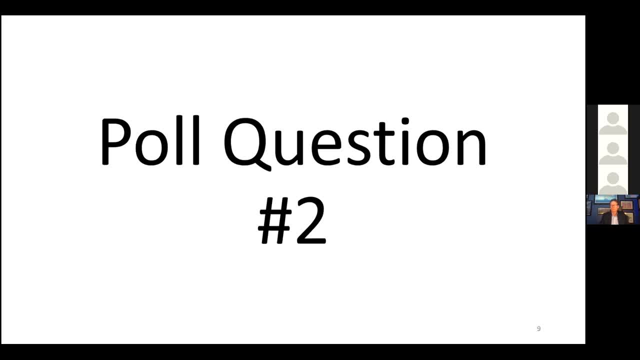 And just to let everybody know, Nick inadvertently said at the end: strongly agree, That should be disagree and strongly disagree, and then don't know everyone. Thank you Great. Thanks very much, Glenn. Always good to have backup. We've got about 70% of the folks online putting in an answer. 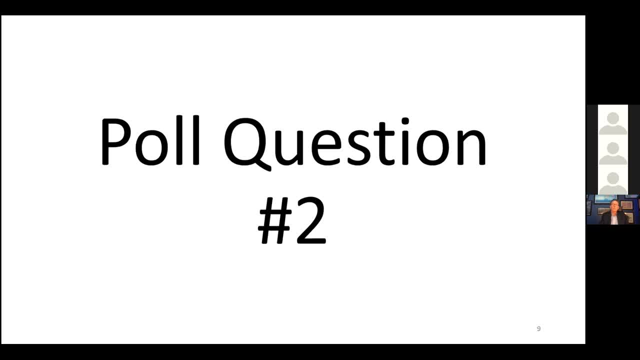 Looks like we're stopping at that point. So it looks like 30% strongly agree and 25% agree, and then the rest are neutral or disagree with some not knowing. Great Good to know. That certainly helps, And then if there are any more questions or any need, I would so then. so we'll move on to. 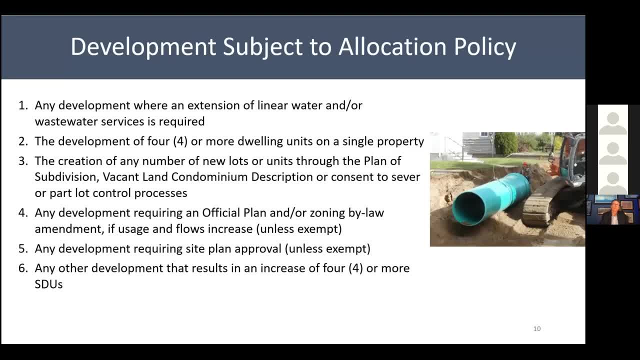 the next slide. Okay, Great, Let's see here. Um, we're next slide here to dé interess. Well, what I can say is that the majority agree there are. there are some things that can be said with this: the claim that the status of the mortgage law would be an exemption. why? very? 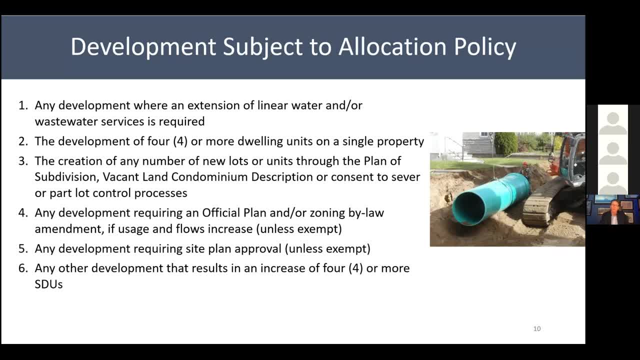 matters from that perspective, especially given that the leniency Could be inserted. UL buffer- Oh okay, would be the subject of the policy. And this is simply because additional water usage and sewage flows will occur as a result. It's a new land use and services are being extended to it. 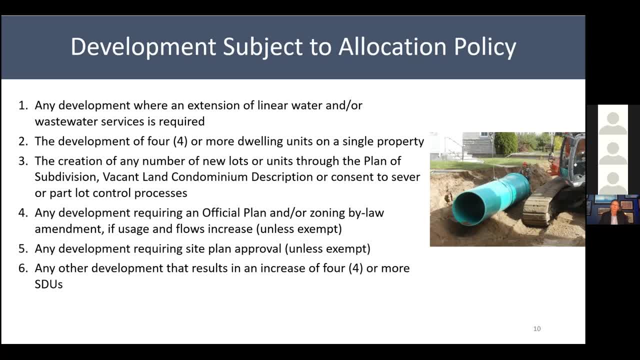 Secondly, the development of four or more dwelling units on a single property would be the subject of the policy, And this would be the case when the long-term exemption I mentioned comes into effect. However, until then, the development of additional dwelling units, except secondary suites. 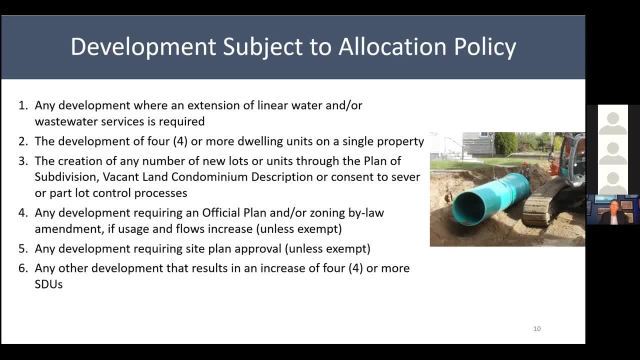 would be subject to the policy. Thirdly, the creation of any number of new lots or units through the plan of subdivision, vacant land, condominium description or consent to sever or part lock control processes. This is straightforward for those on the call, but for those who do not know what part lock control is, 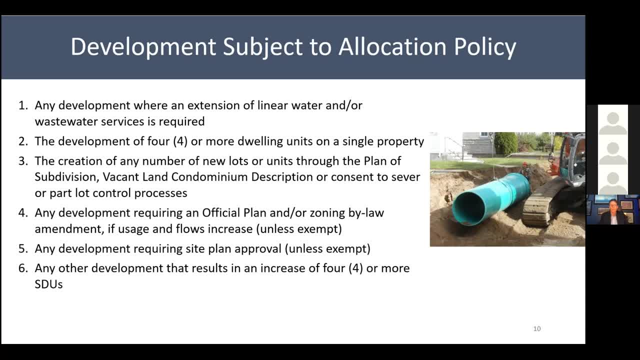 for example, that's the creation of lots from blocks in the plan of subdivision And, as often, the process relied upon when freehold street townhouses are being built, for example. Fourthly, any development requiring an official plan and or zoning bylaw amendment. 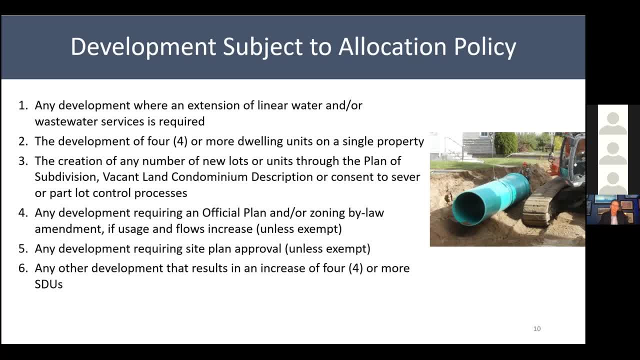 if the usage and flows increase, unless, of course, they're exempt as per the previous slide, such as a residence changing into a residence that requires a rezoning. Any development requiring site plan approval would be subject unless they're exempt, And then any other development that results in an increase. 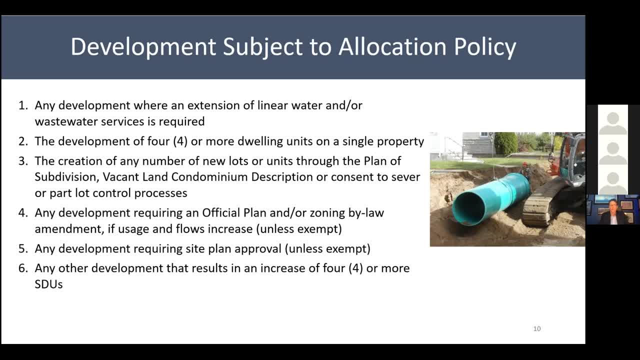 of four or more SDUs, And this is essentially to cover off anything that's not already listed and covered off in. and this is essentially to cover off anything that's not already listed and covered off in in the previous categories. Next slide: 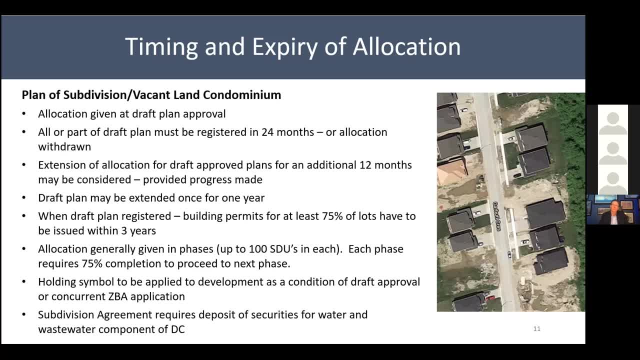 So in terms of timing and expiry of the allocation itself, and this is for plans of subdivision, vacant land, condominium. So we're suggesting that allocation will be given at draft plan approval And in our view, this provides a developer with the commitment that services are available. 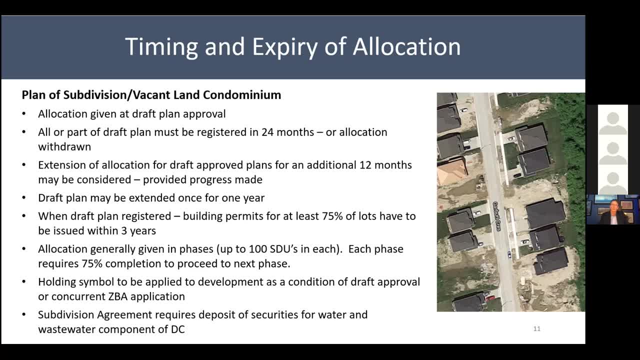 and obviously allows the developer to begin work clearing conditions knowing that that's the case. All or part of a draft plan must be registered in 24 months or the allocation will be withdrawn. The extension of allocation for draft approved plans could be considered for an additional 12 months. 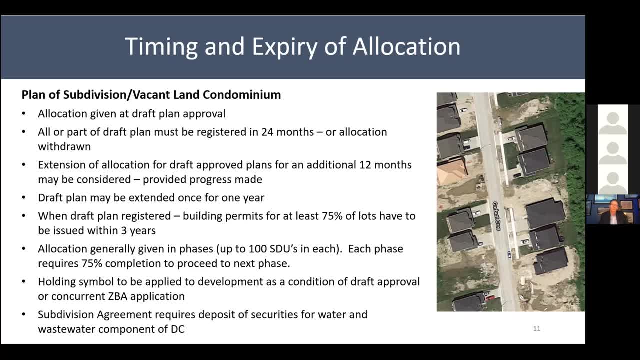 provided progress has made on clearing conditions such as completion and acceptance of servicing and grading plans, And these are just. these are just examples. The draft plan approval itself may be extended once for one year. We recommend that the plan may be extended once for one year. 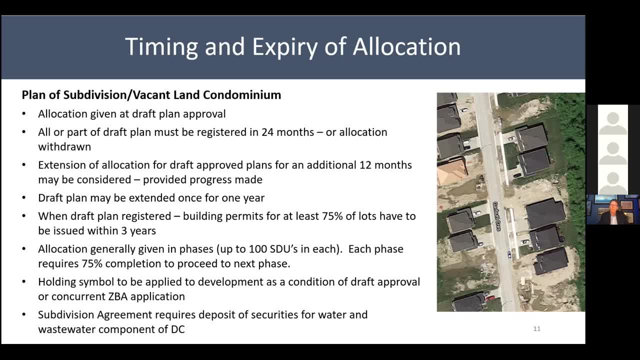 We recommend that the plan be extended once for one year, recognize that this needs to be further considered as changes to the official plan may be required to implement this, but we're suggesting this at this point and we will be looking for your comments. 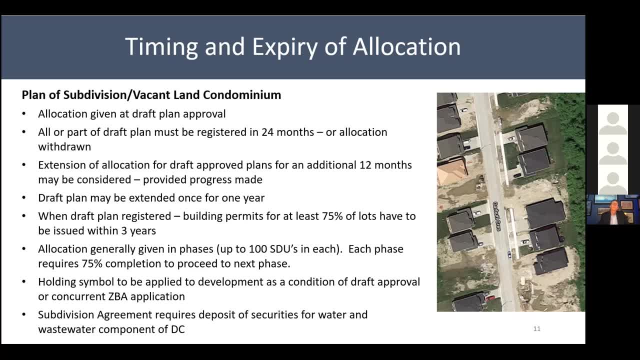 I do have two phones in my office and the other one is ringing, So when the draft plan is registered, building permits for at least 75% of the lots have to be issued within three years. Allocation would generally be given in phases and that would be up to 100 SDUs in each. 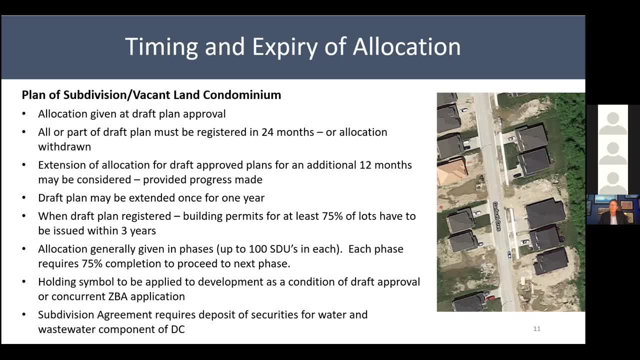 and each phase would require 75% completion to proceed to the next phase. In order to implement all of this, there would be a holding symbol applied to the development as a condition of draft plan approval or concurrent with the zoning by-law application and decision process. 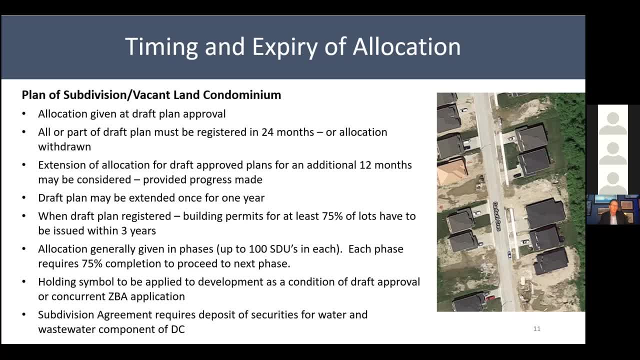 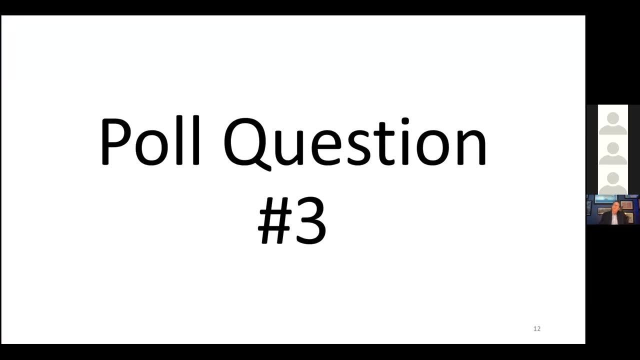 And then the subdivision agreement itself would require the positive securities for water and wastewater component of the development charge. So this brings us to our next poll in question, question three, which I will read. So, in your view, should capacity for plans of subdivision? 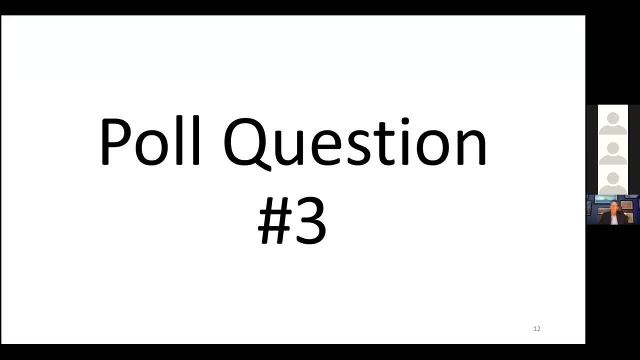 or vacant land condominium be allocated when draft plan approval is given, which is what we're recommending, or should it be given at agreement registration stage? Neither or don't know. Really happy to see everybody, I would like to say I think we've got a lot of questions. 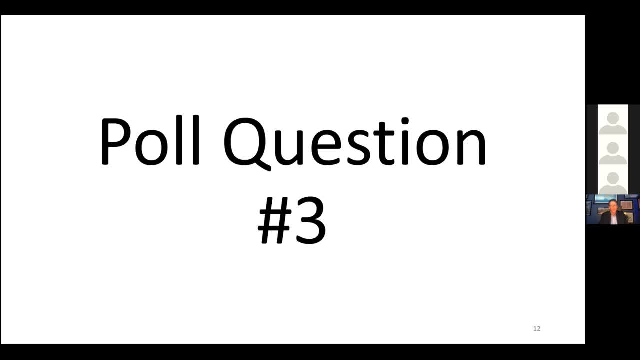 and I don't know if anybody is answering these question. These are these questions will really help us. the answer to these questions will really help us in formulating a final policy. And I'll just note Nick, in talking to the town, of course, 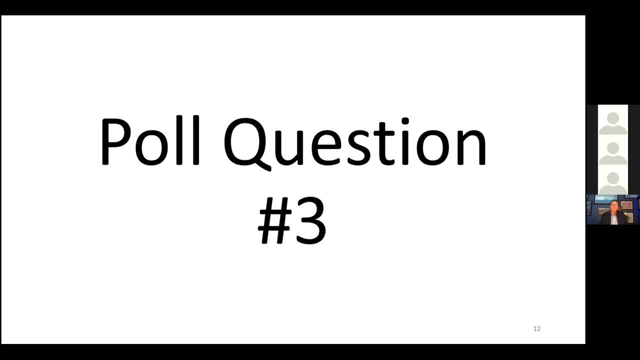 these polling questions are designed to be indicative only. they are not statistically generalizable to the broader population. So the team will be using the polling questions and the question that comes from the county is not available. so that's why we're working with the county werden. 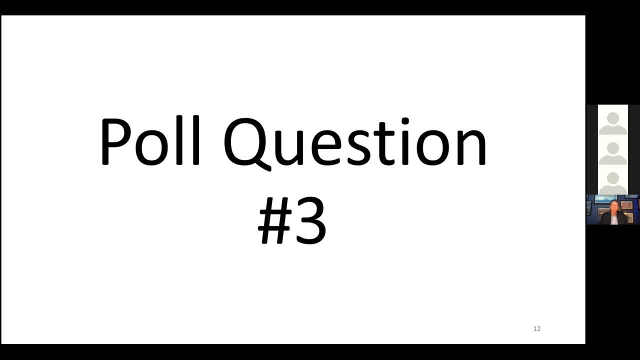 and who, again, who is the person, who is the scientist on the house using them from that perspective? But back to you, Nick, to summarize the results. Great thanks, Glenn. That's how I certainly saw it as well. 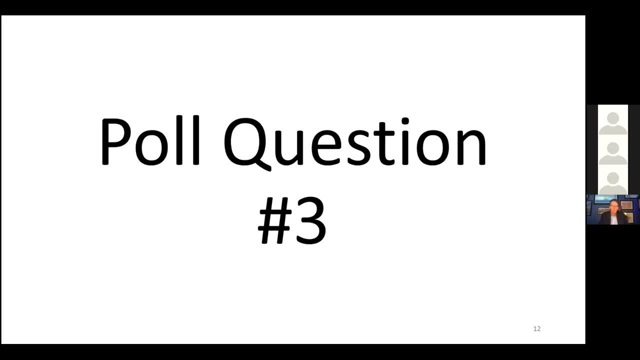 So, looking at the answers, it looks like 55% of those on the call today agree with the current recommendation, that is, to grant allocation of time of draft plan approval. but we do have a sizable number- 32%- who think it should be at the agreement registration stage. 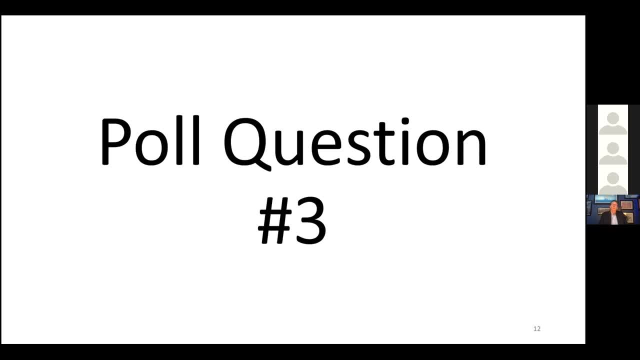 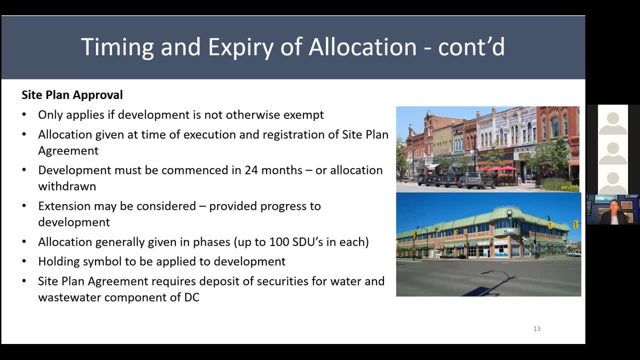 Okay, that's great Good to know. Thank you, We'll move on to the next slide. So, with respect to site plan approval, which is another type of planning approval, it would obviously the policy would only apply if the development is not otherwise exempt. 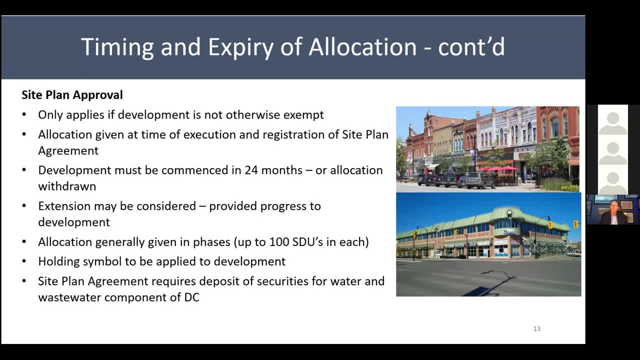 as I've already discussed, The allocation would be given at the time of execution and registration of the site plan agreement. The development must be commenced in 24 months or allocation withdrawn. While we do recognize the Planning, Act does not specifically allow for servicing to be a component of the site plan approval process. 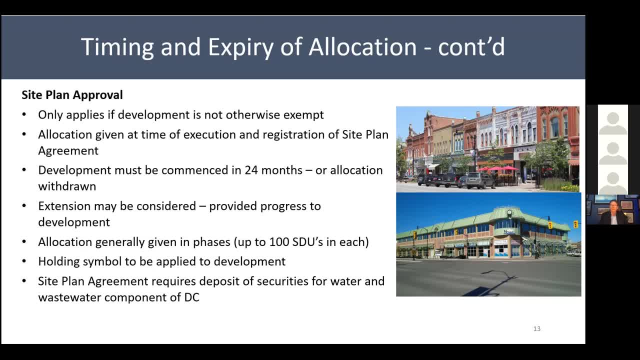 the agreement itself can be prepared in a manner such that it expires after a period of time, so we get at that issue in a different way. The extension and an extension to the allocation may be considered Again, provided that there's some progress. 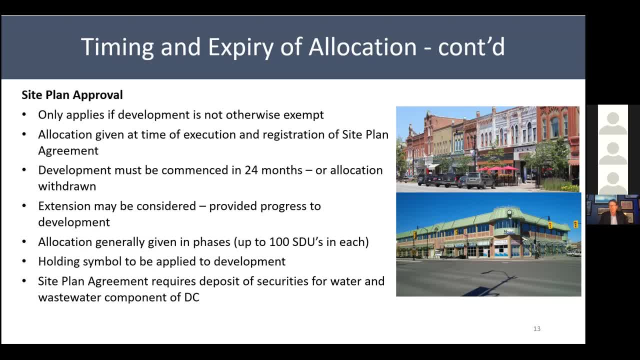 to the development on the site. The allocation would generally be given in phases, again up to a 100 SDU's in each, and of course a holding symbol would be applied to the development as necessary, and then the site plan agreement would require a deposit of securities for water and wastewater component. 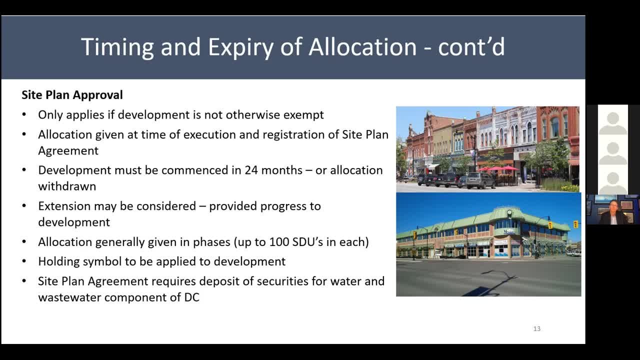 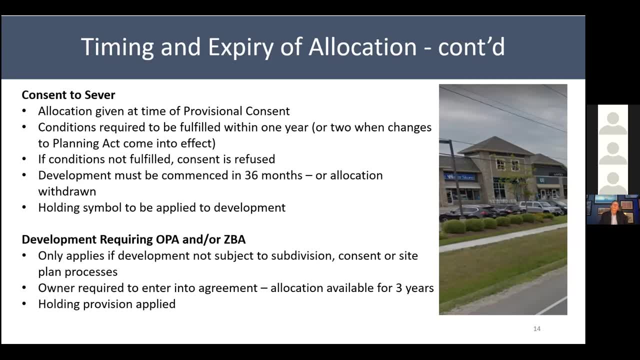 of the development charge as well. The other types of applications that are dealt with in the strategy are consent to sever, and the allocation would be given at the time of provisional consent. Conditions would be required to be fulfilled within one year. That's currently the way it is according to the Planning Act, but there are changes proposed to the Act that would 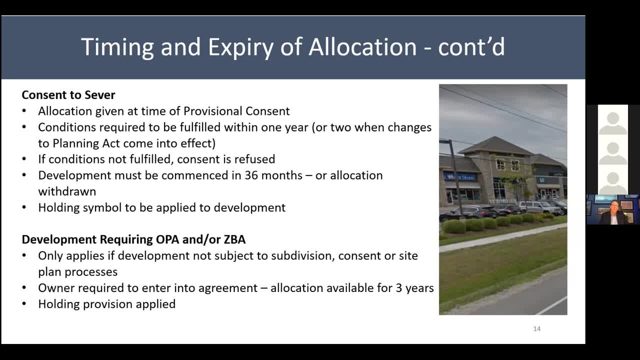 allow conditions to be fulfilled within two years. If conditions are not fulfilled, a consent is deemed to be refused. If the conditions are fulfilled and the lot is created, the development must be commenced in 36 months or the allocation withdrawn and then a holding symbol would. 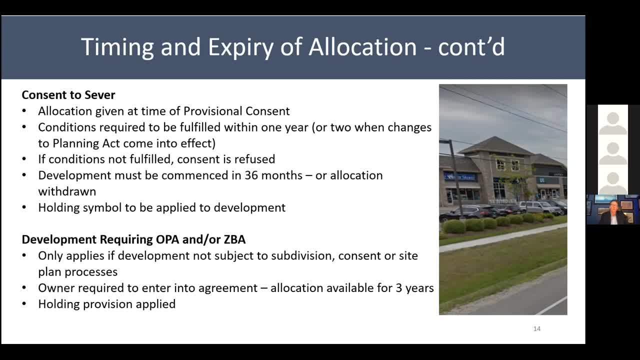 also be applied to the development, just to make sure that development occurs in accordance with these provisions. In the last circumstance- and this would be for developments requiring only an official plan amendment or a zoning bylaw amendment and not site plan approval or subdivision approval or some other type of approval, and these are rare but they do occur- the owner would be. 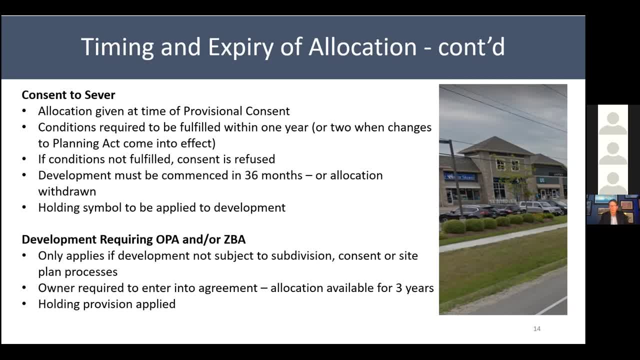 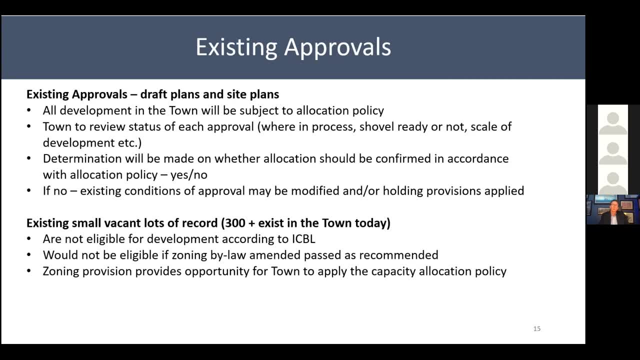 required to enter into an agreement and then the allocation would again be available for three years and a holding provision would also be applied. Next slide, please. So existing approvals- and there are a number of them in the Town to consider- and with respect to draft plans and site plans, as I mentioned, all development in the Town will be 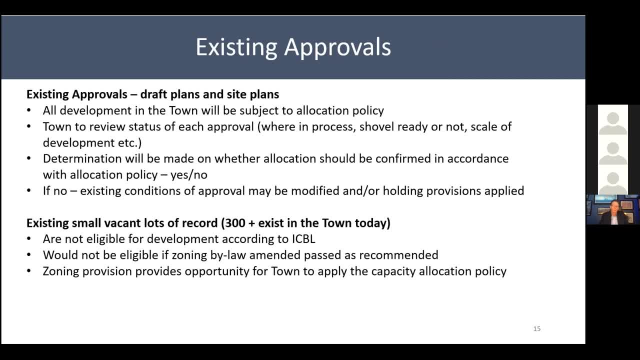 subject to the allocation policy going forward- and when I say going forward, that is after Council endorses the document- The Town is planning on reviewing the status of each approval in terms of where they are in the application process, and the status of each approval in terms of where they are. 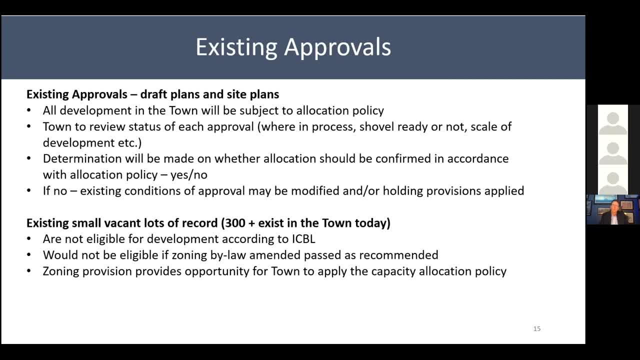 in the process. are they shovel ready or not? the scale of development: is it minor, is it major, etc. A determination will be made on whether allocation should be confirmed in accordance with the allocation policy- and that's a yes, no- and if no existing conditions of approval may be. 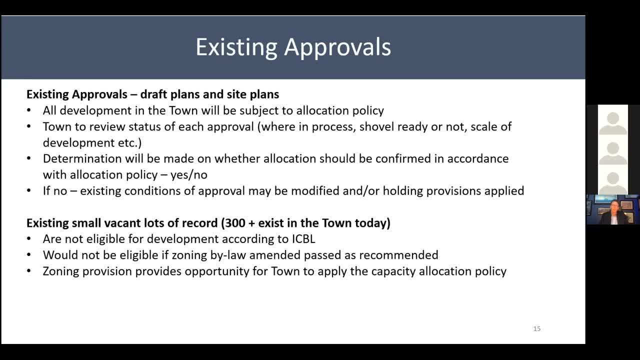 modified and or holding provisions applied as necessary. This is going to take the Town some time to figure this out. There are a few approvals out there to consider. There are a few approvals out there to consider And this is going to be initiated in the short. 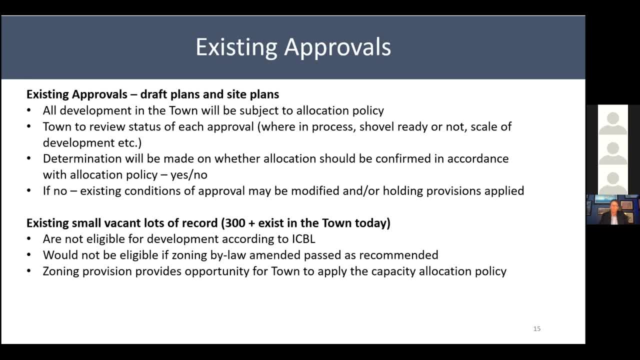 term once we have direction from Council on a direction to take with respect to the policy approach. There are also 300 existing vacant lots of record in the Town. Currently they are not eligible for building permits according to the interim control bylaw and they would not be eligible for building permits if a zoning bylaw amendment is passed as 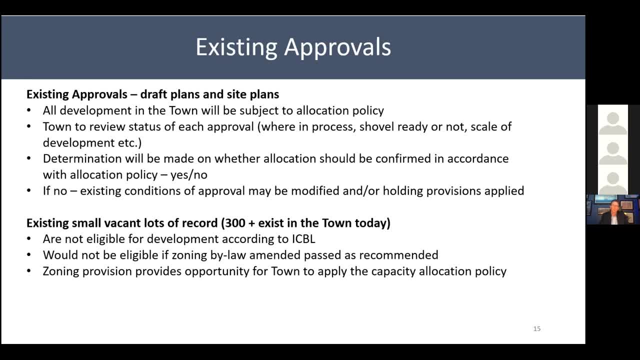 recommended- and I'll talk about this a little later in the presentation- and, of course, if the bylaw is amended, it would provide the Town with the opportunity to apply the capacity allocation policy, Because there are so many vacant lots in the Town we have come up with. 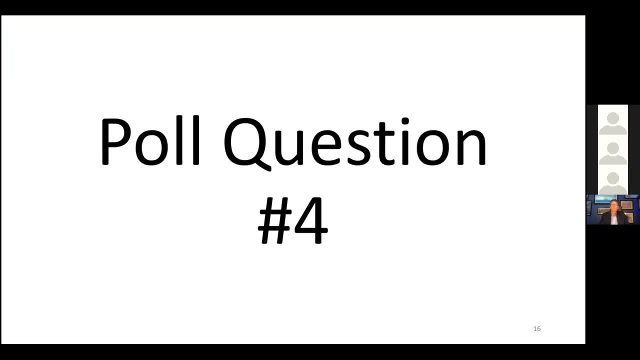 the next polling question, which I will read. So which of the following would be your preferred approach to allocate capacity to existing small vacant lots and, as I mentioned, there are 300 of them in the town? So, firstly, by evaluating proposals against the full merit-based criteria and the capacity allocation policy which we're 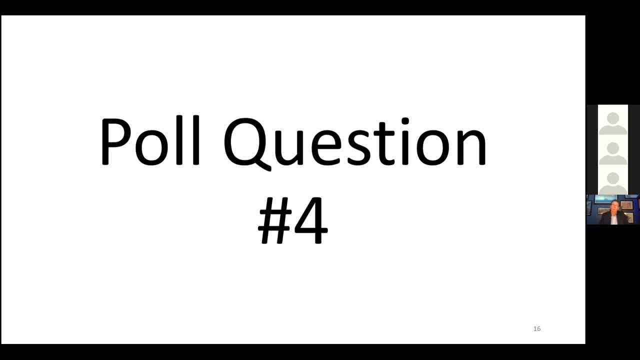 recommending or by evaluating proposals against a shortened version of the merit-based criteria. Thirdly, by setting aside a certain percentage of capacity each year and allocating it on a first come, first serve basis, and this may involve capping the number of vacant lots that could be developed in a given year. and lastly, don't know, Looks like most are participating, which is great. 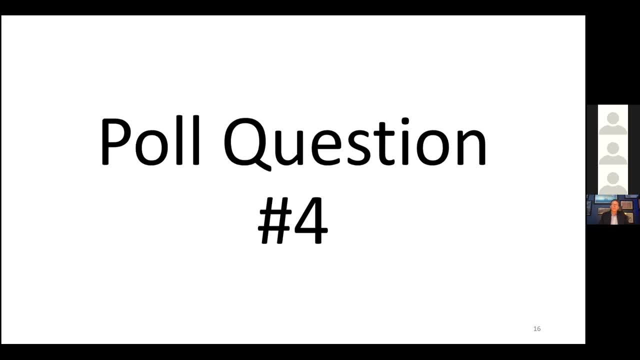 Looks like we've got answers in every category and it looks like there's some traction for setting aside a certain percentage of capacity each year and allocating it on a first come, first serve basis- Certainly a very simple approach and something we'll certainly be looking at Coming in. 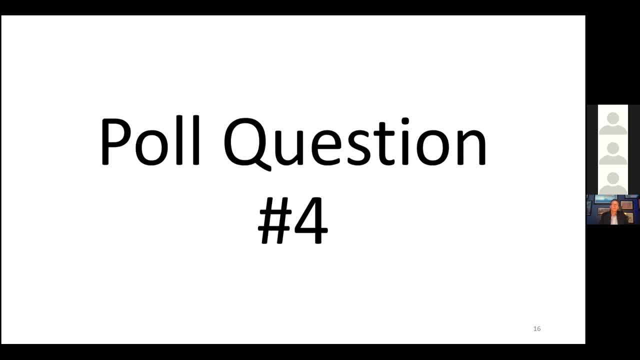 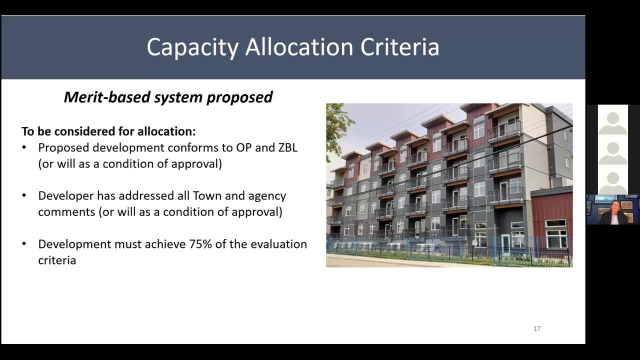 second is the evaluation of those proposals against the full merit-based criteria. Okay, so we're going to move on to the next slide. That's great, thank you. So, in terms of the capacity allocation criteria itself, obviously this is a key element of the overall approach and, in this regard, and to be considered for allocation in accordance with: 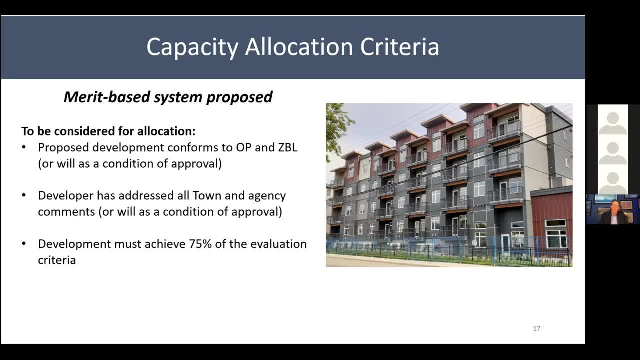 with these merit-based criteria, the proposed development must conform to the OP and zoning bylaw or will as a condition of approval. I think that's great. That goes without saying. the developers addressed all town and agency comments or will as a condition of approval. and then, lastly, development must achieve 75 percent. 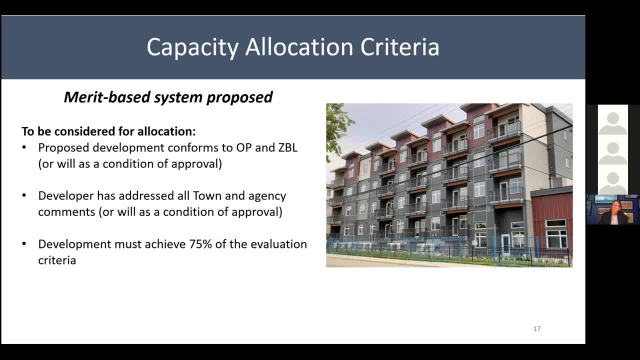 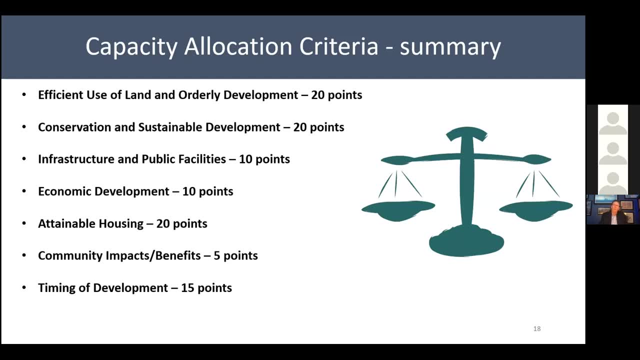 of the evaluation criteria and I'll come back to that in a moment, Next slide. So this slide identifies the categories we have come up with in the draft policy and the number of points assigned to each. and that is, efficient of use of land and orderly development: 20 points. 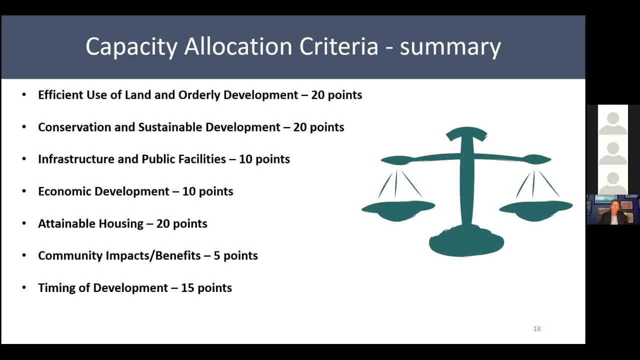 conservation and sustainable development is 20,, infrastructure and public facilities is 10,, economic development is 10, attainable housing is 20,, community impacts and benefits are 5, and timing of development is 15.. You'll see that we've placed greater emphasis on the first two. 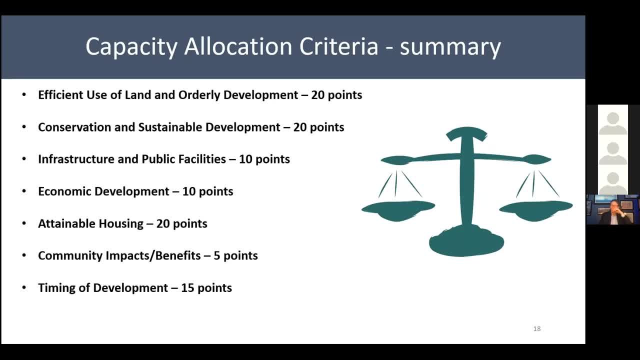 and attainable housing. So there is quite a bit of detail in the draft document, which I'm not, which is not reproduced in this slideshow but in the category. but in the category of efficient use of land and orderly development, we've come up with a number. 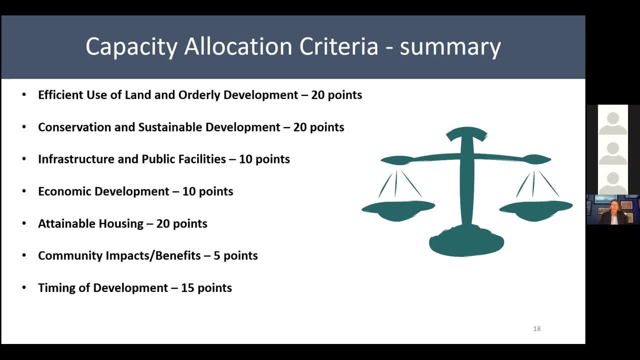 of criteria, and they include, for example: are the lands within the built boundary? Yes, no, because there's a focus on intensification both at the provincial level and at the town. Does the development include a mix of land uses, especially those that provide for live work? 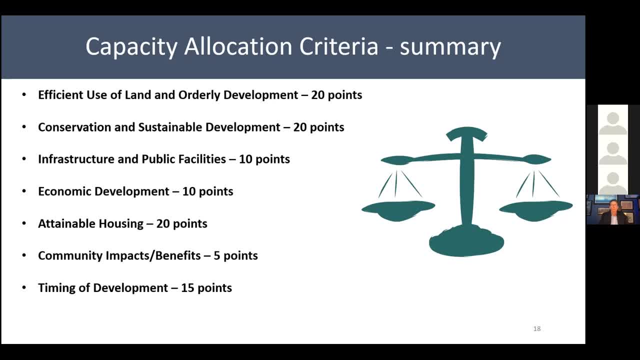 arrangements. Does the development represent an orderly and sequential expansion of the community outward from the existing built-up area? Does the development represent transit supportive development based on density and proximity to transit use routes? And does a development facilitate the development of a brownfield site? So all these 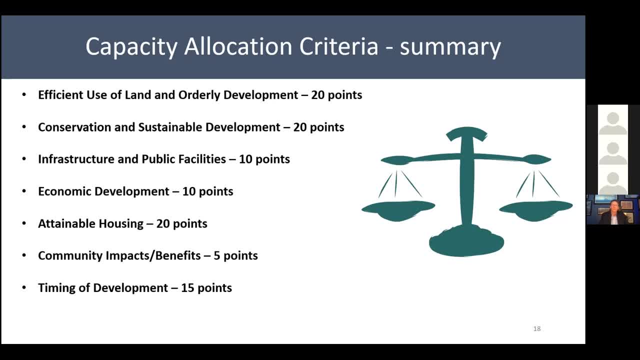 are yes or no, and points would be assigned based on whether the development was a yes. So, again, those are examples of what we've come up with in that particular category. We are certainly open to wordsmithing. This is a first draft and we will be looking for comments on. 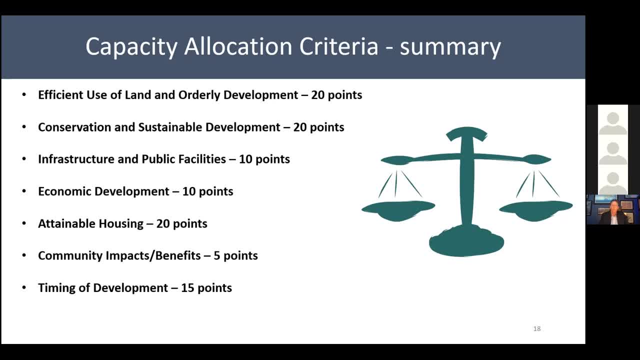 how the wording can be improved wherever possible to provide clarity. Under the category of conservation and sustainable development, we've come up with criteria that, for example, deal with: does a development incorporate low impact or sustainable development as it relates to water efficiency and reduced wastewater flow from development? 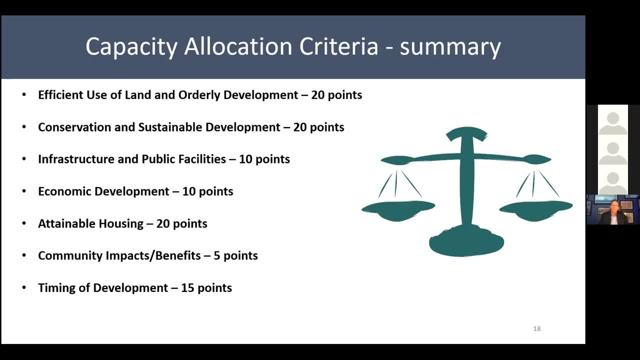 projects And then the measurement would be the degree of compliance in that particular case. Would the development achieve LEED, ENERGY STAR or other similar certification or equivalent? Will the development incorporate green development standards or methods that contribute to sustainability of the development, such as passive solar design, climate change resilient buildings? 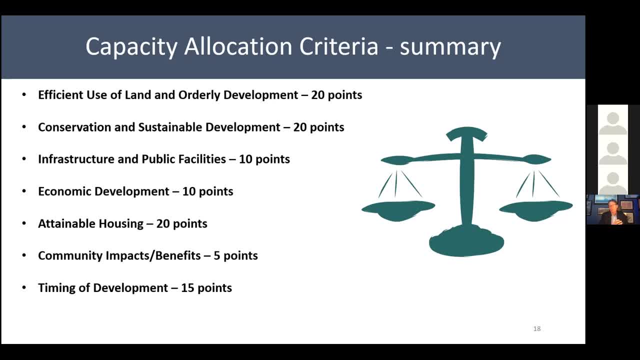 and infrastructure and so on? And would the development facilitate the transfer of natural heritage lands into public ownership or land trust? So again, those are examples of criteria under the conservation and sustainable development bucket. In the infrastructure and public facilities category we've come up with a few criteria, or two actually. One indicates: does the development? 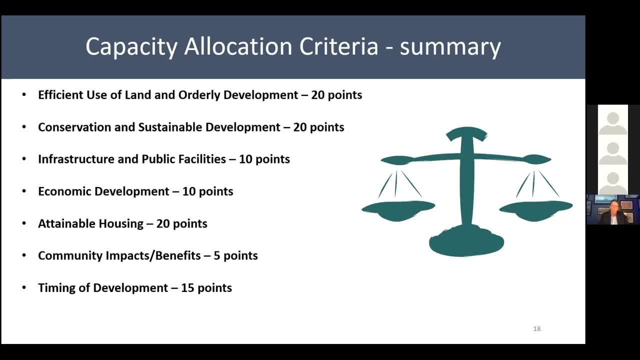 include the completion of required key infrastructure, such as road connections between development areas and or water and sewage infrastructure. Again, degree of compliance would be the measure. And then the second one we've come up with is: does the development enable the provision of public facilities beyond those that are required? 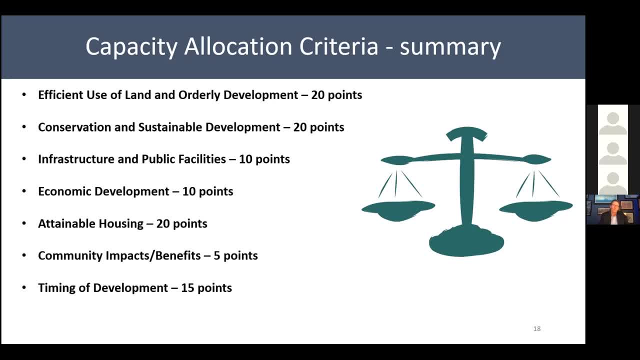 to be provided by legislation. And again, degree of compliance is the measure Under the economic development category. does the development add new jobs to the local economy? Does the development enhance the downtown or main street as a focal point of activity and commerce? 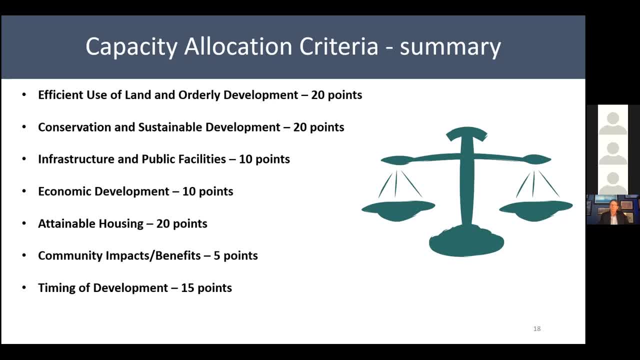 Under the category of attainable housing, which is incredibly important. we've come up with a few criteria. One: does the development include affordable housing units, for example? Does the development propose innovative housing solutions that contribute to attainability and affordability? Does the development actually include rental housing units? 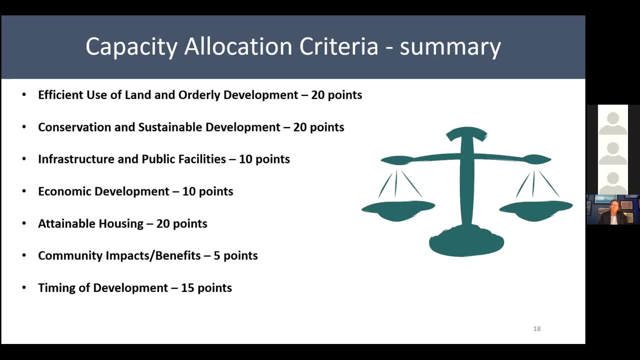 Does the development include seniors, community or special needs housing And does the development include a mix of housing types, with one housing type comprising no less than 10% of the total units? Community impacts and benefits is another category. Does the application preserve? 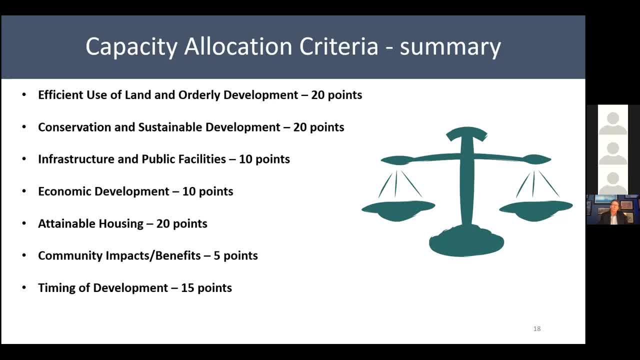 sites, buildings of historical interest? Will the development facilitate the removal or improvement of a land use complex And the measure there would be? degree of compliance And then, lastly, timing of development, the extent to which development's shovel ready. Certainly, 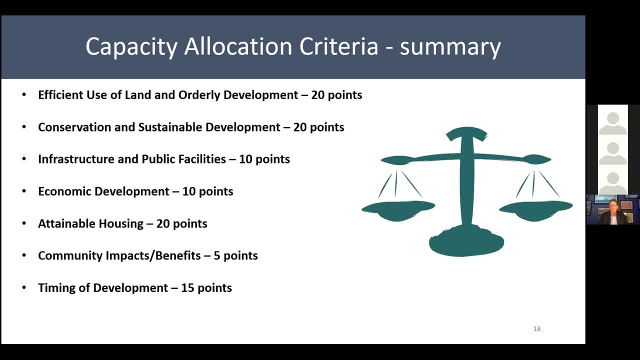 that was a big factor for the Town when they were making decisions on exemptions to the current ICBL drunk. So, at the end of the day, there is a maximum number of points available for residential and non-residential, And we're suggesting for discussion purposes that a development has to achieve 75% of the available score in order to be considered for allocation. 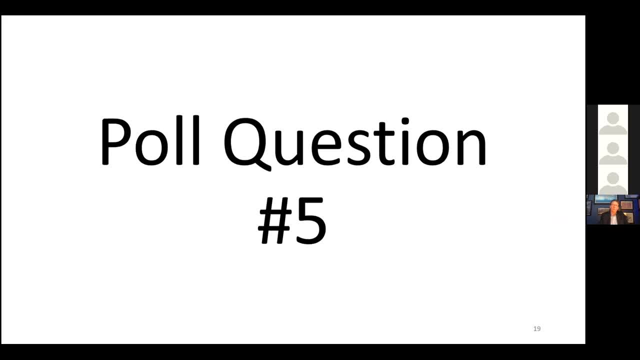 So this brings us to the next polling question, which has to do with the level of emphasis that should be placed on each of the categories identified in making a decision. So, for example, and as I mentioned in our recommendations, we have placed greater emphasis on efficient use of land and orderly development, conservation and sustainable development and attainable housing. 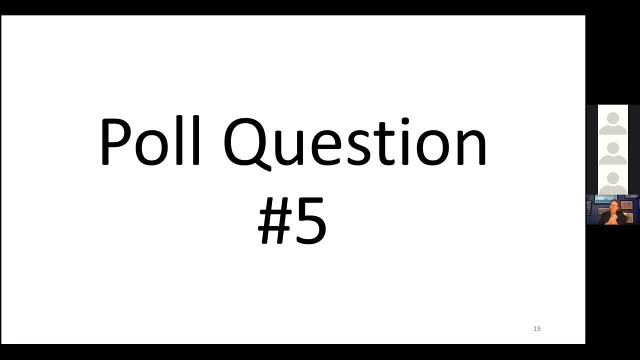 We have done this because we think, at this point, that these are the most important. However, we're looking for your views. So here is question number five, which I will read. So which three of the following would you say are the most important categories? 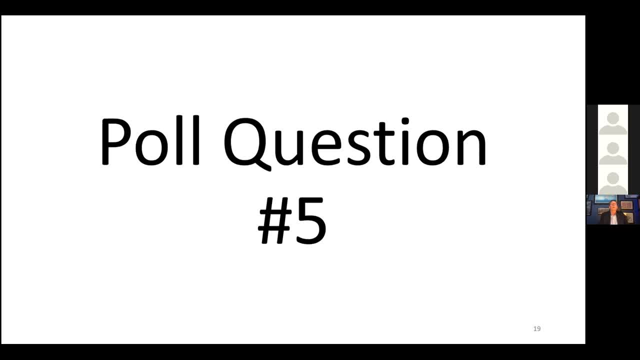 So you can pick three in this list When applying the merit-based criteria for capacity allocation, And the list is here: Efficient use of land and orderly development, conservation, sustainable development, infrastructure and public facilities. economic development, attainable housing, community impacts and benefits. 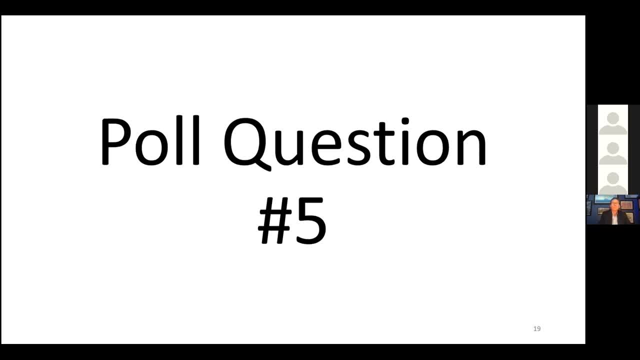 and time constraints. And just a quick note: everybody, you probably figured this out, But if you're doing it on a smartphone and you have a small screen, you can toggle to move the list up and down so that you can see all of the options. 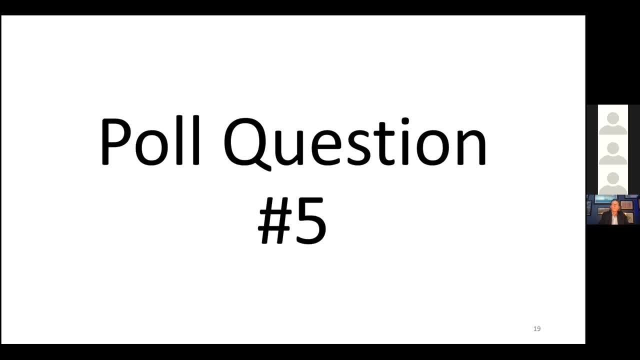 Just make sure that you aren't missing any. Thank you, Okay, I'll just wait a couple of seconds to see where we end up. So it looks like at this point that a large majority of the participants think that emphasis should be placed on efficient use of land and orderly development. 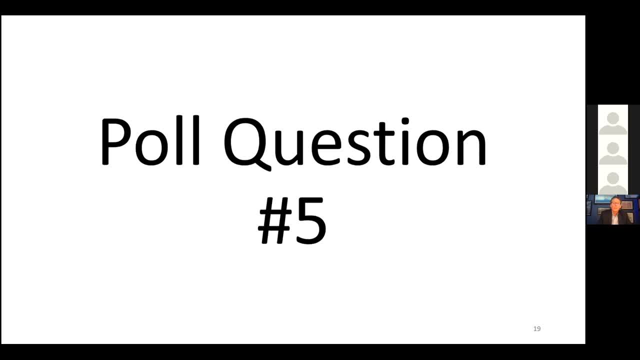 That's 76%, And coming in second is infrastructure and public facilities, And then the others are all evenly divided into 20, 26, 20 and 24.. 20%, Actually, timing of development, at the bottom of the list, is coming in at 66%. 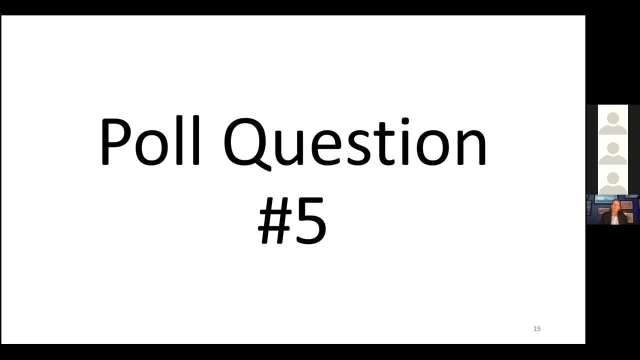 Two-thirds have put that in their top three. Thank you very much, Glenn. That didn't even show up on my screen. I should make that box a little bigger, So you're right. So timing of development came in second, And then infrastructure and public facilities came in third. 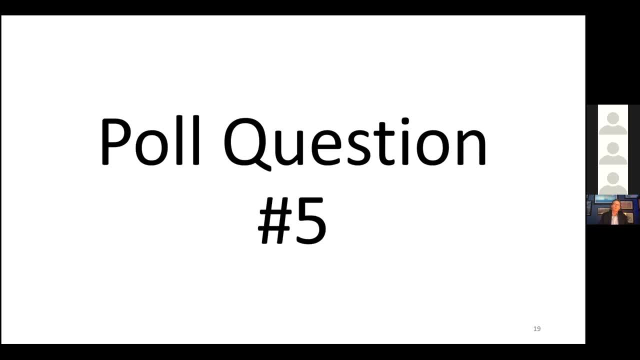 Okay, those look like the top three according to this group. Great, Thank you very much. So we also have a second question as well on this, which is question number six- I believe Maybe it's number five- And at present we are suggesting that a minimum overall score be attained to be considered for allocation. 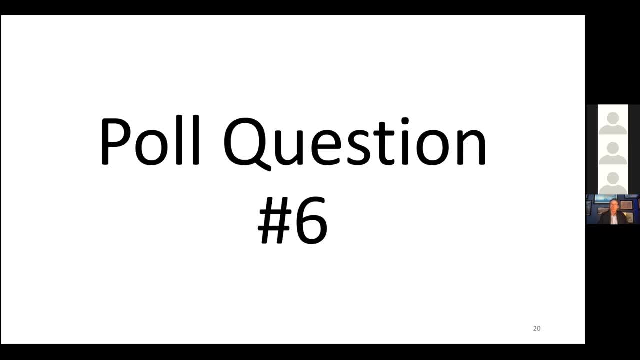 And this recognizes that not all development, in our view, will check the boxes, so to speak. So, in the alternative, to what extent do you agree that a minimum score should be achieved? Okay, So in the alternative, to what extent do you agree that a minimum score should be achieved? 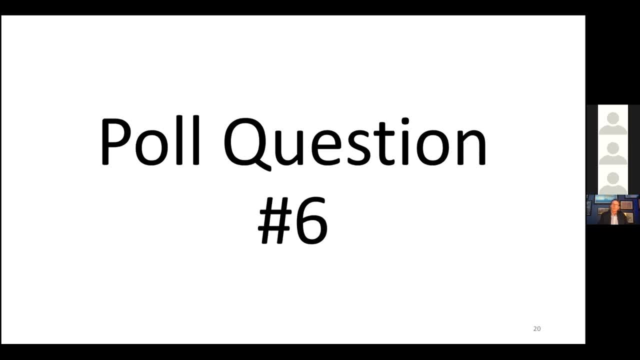 Okay. So in the alternative, to what extent do you agree that a minimum score should be achieved? Okay, We will discuss each category of the merit-based criteria: Strongly agree, agree, neutral disagree, strongly disagree or don't know. 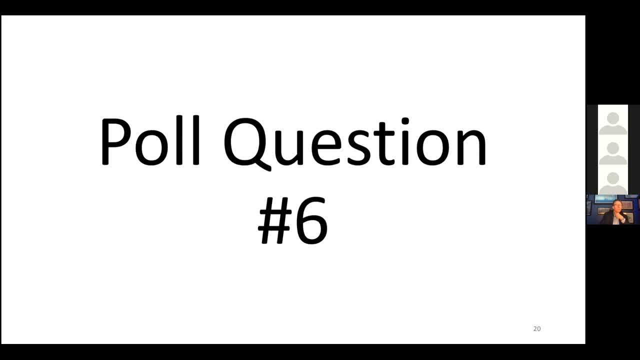 Clearly an alternative approach, and it would require a level of effort to figure that out, but it's something that we could consider as well. So it looks like Most folks are saying they strongly disagree, which is at 44%. And then there's the next component is disagree. 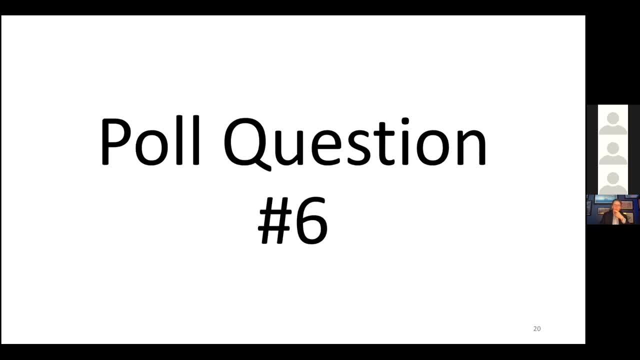 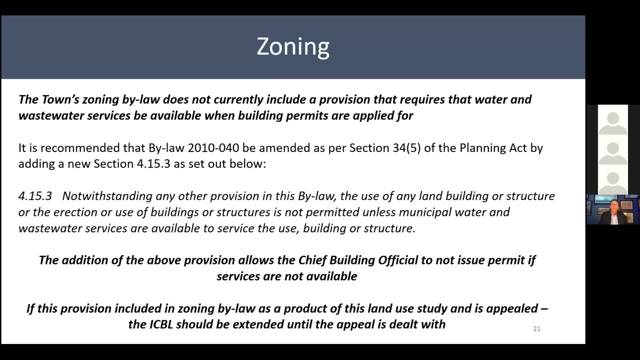 So, based on this crowd only, there isn't much support for the alternative. Great Thanks for that. We'll close that and move on. So only a couple more slides. So we also looked at. We looked at the town's zoning bylaw and it currently does not include a provision. 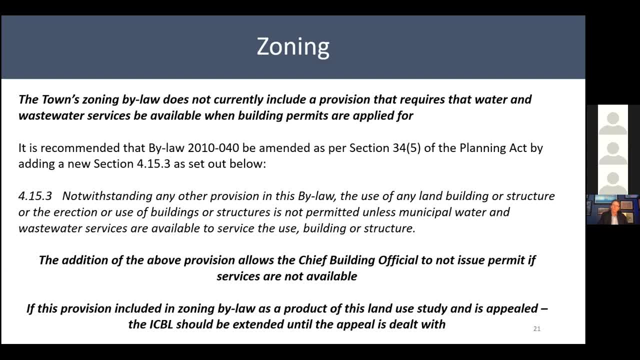 that requires that water and wastewater services be available when building permits are applied for, And this means that there is no legal way to not issue a building permit, since there is no applicable law that would prevent this from occurring. So, with that in mind, we're recommending that bylaw 2010-040 be amended. 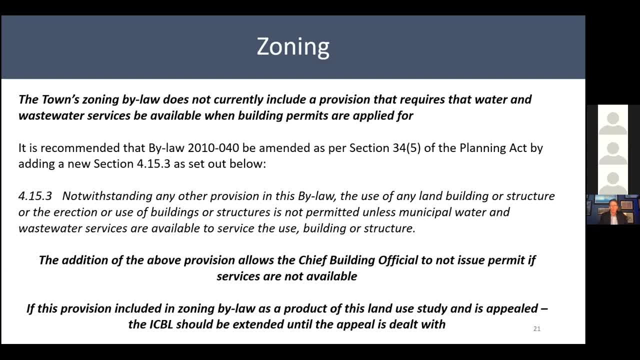 as per Section 34.5 of the Planning Act. by adding a new section, as set out on this slide, It basically acts as a notwithstanding over any other provision in the bylaw and it would say that the use of any land, building or structure. 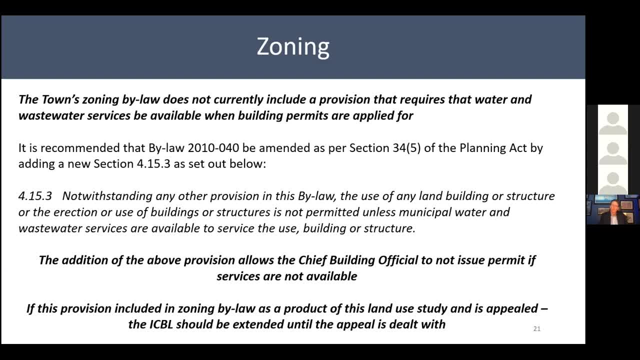 or the erection or use of buildings or structures and this is kind of Planning Act. language is not permitted unless municipal water and wastewater services are available to service the use, building or structure. The addition of this provision into the town's zoning bylaw. 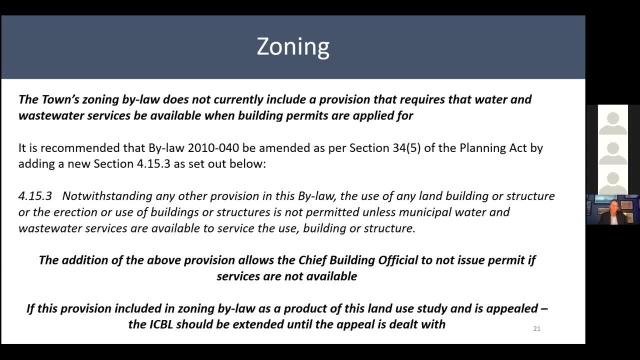 would allow the chief building official to not issue a permit if services are not available. I should also note that if this provision is included in the zoning bylaw as a product of this land use study and is appealed, the interim control bylaw would be extended until the appeal is dealt with. 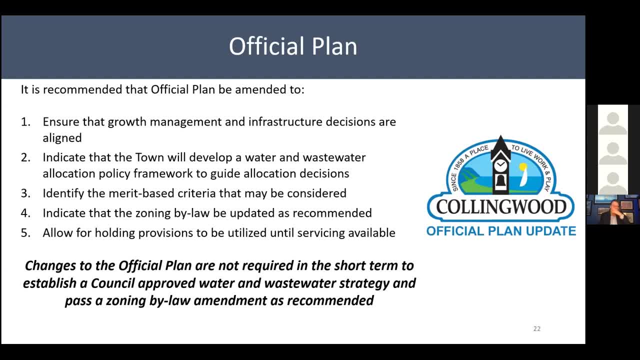 Next slide With respect to the official plan. we do also recommend that the official plan be amended to ensure that growth management and infrastructure decisions are aligned. Certainly, the town is already going through an official plan update process and is working on the development of those kinds of policies. 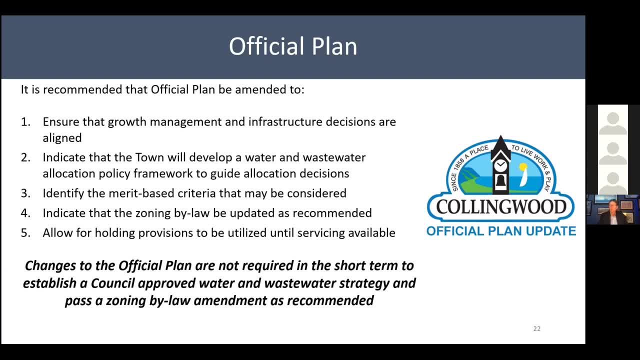 We also think the official plan should indicate that the town will actually develop a water and wastewater allocation policy framework to guide allocation decisions. It should indicate that a merit-based criteria approach may be considered, but it wouldn't get into what those criteria are and how they would be stored. 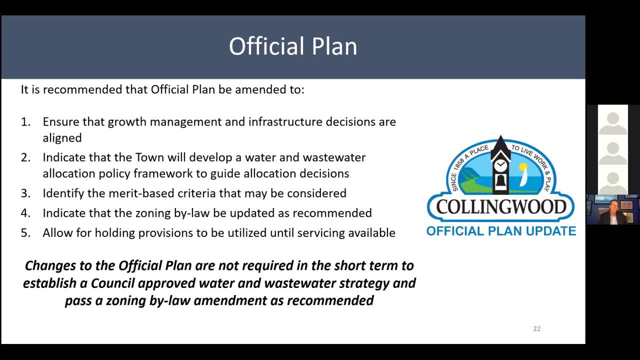 It would just be said in a general way. It could indicate, or shouldn't indicate, that the zoning bylaw be updated as recommended, and it should also allow for holding provisions to be utilized until servicing is available. However, we don't think the changes are to the official plan are required in the short term. 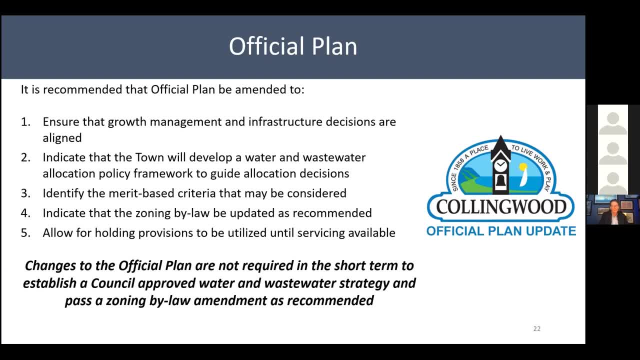 to establish the county Council approve water and wastewater strategy, because such a strategy does sit outside of the Planning Act and it is a decision of Council that involves the allocation of capacity to water and wastewater in the town, And I also don't think changes to the Official Plan. 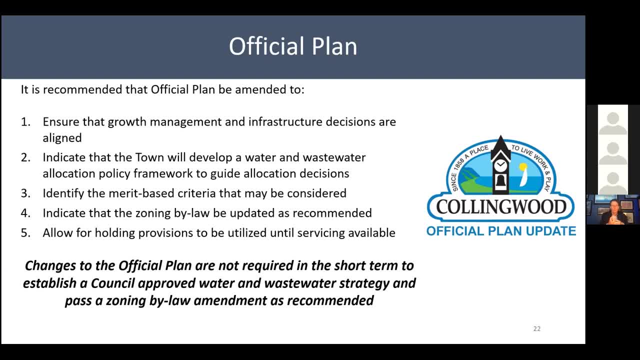 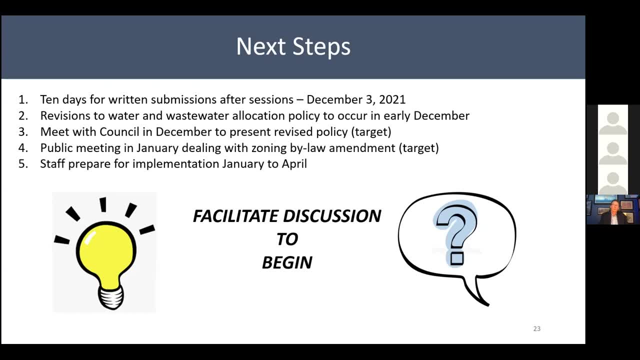 are required to pass a zoning bylaw amendment, as recommended either Next slide. So in terms of next steps, timing is tight for sure, We recognize that in a very significant way. but it is the town's wish to establish an appropriate allocation policy framework. 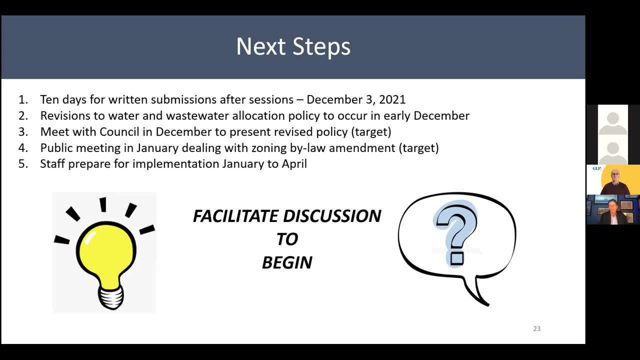 in an expeditious manner. So 10 days are set aside for written submissions after the sessions. today, That means December 3rd 2021, that's a Friday. We anticipate that revisions to the policy will occur in early December. 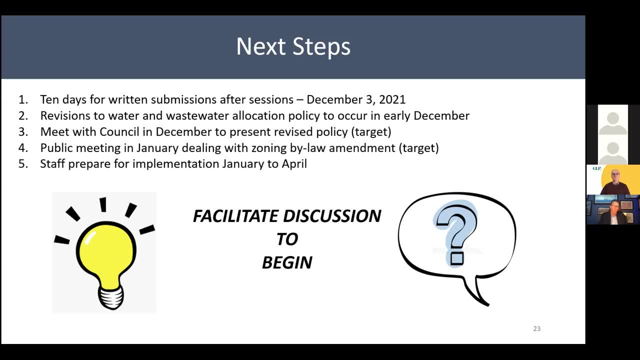 We would then meet with Council in December to present the revised policy At this point. that's a target And if it does occur, it would probably occur on December 20th. There would be a public meeting in January to deal with the zoning bylaw amendment. 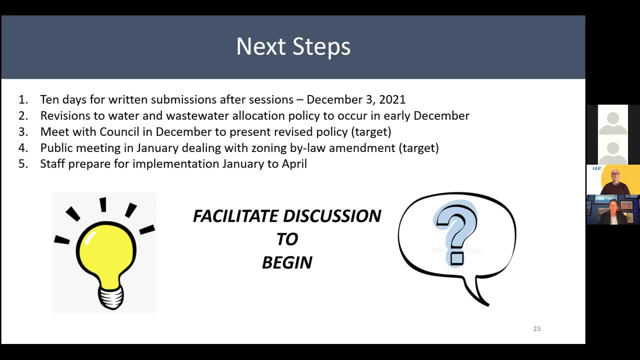 Our recommendation that we've made again. that's a target And, as I mentioned earlier, staff would be working very hard on the implementation of this in the January to April Time period, before the ICBL expires in April. So back to you, Glenn. that's it for my presentation. 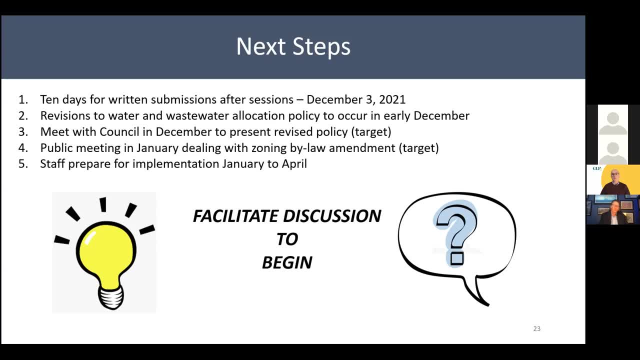 Well, thank you very much, Nick, for the overview of the framework and also all of that additional important information. Okay, so we've heard from the town and we've heard from their planning consultant. Now it's time to hear from you, our session participants. 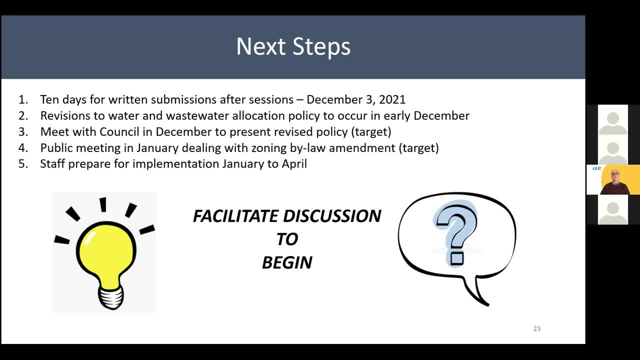 And give me just a couple of minutes to set this up for you Again. some of you are very familiar with Zoom, Others may not be as familiar, So let me just say a couple of things First. again, I will note that the town has a few questions. 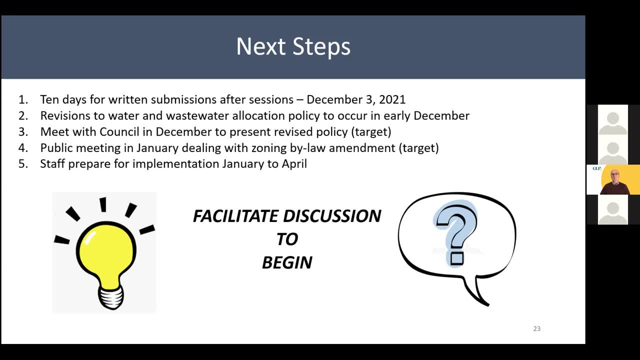 to which they would like to get your responses. We'll put them on screen in a couple of minutes And, again, your answers to those questions can help inform and shape the water and wastewater allocation policy In this portion of the meeting. again, 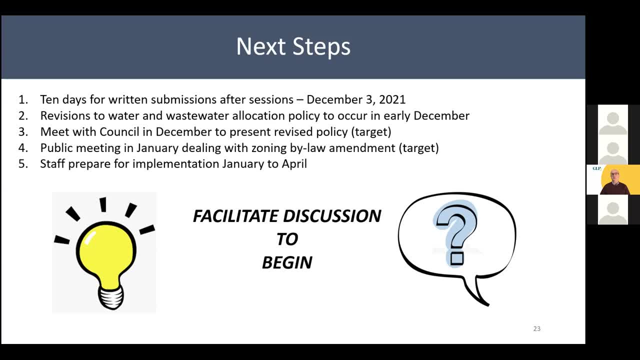 I'll be posing some of those questions and inviting your responses, But you are also invited to share any general comments or reactions you might have on the draft policy and on the framework, And, of course, you're encouraged as well to ask any questions of fact or clarification. 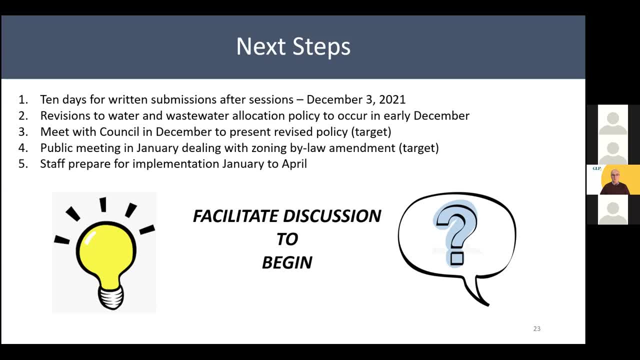 that you might have And let me quickly outline for you the options in terms of how you can do that. And again, for those who may be less familiar with the Zoom platform, I'll go into a little bit of detail So you can share your comments and questions. 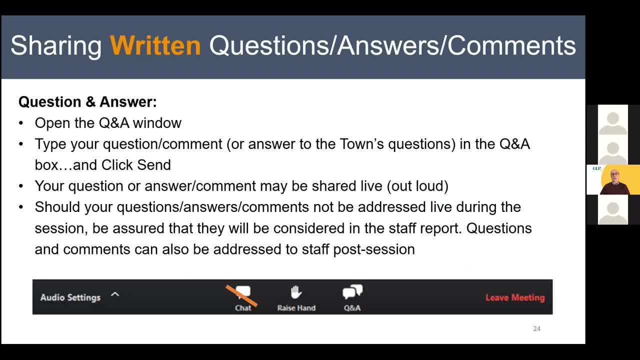 either in writing or orally, And we have up on screen right now the instructions about how to do that in writing. So if you'd like to share your thoughts that way, you can use the written Q&A function, And to do so, please open the Q&A window And you should see a little symbol for it. 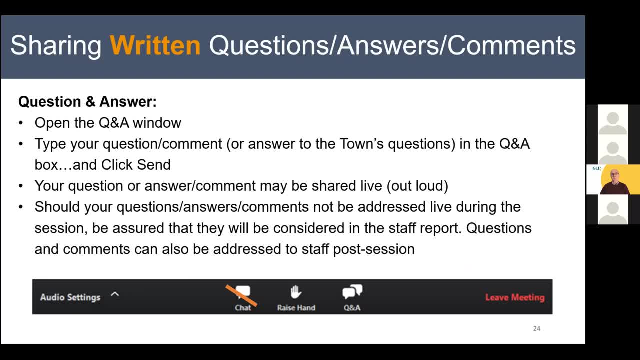 If you use your cursor and hover over the bottom of your Zoom screen, you should see it there So you can. once you've opened the window, you can type in your question or your comment about the material. Or again, you can type in your answer to our questions. You will see those. 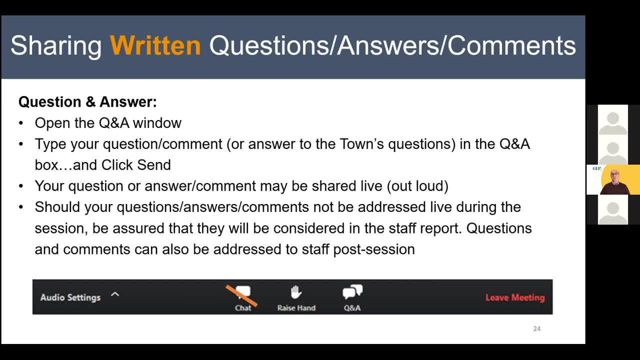 questions in a moment. I would encourage you to just reference your answer. So, for example, if the question is question B, when you put an answer you could just say QB and then put in whatever your answer is, And then our community planner from the town of Collingwood will be. 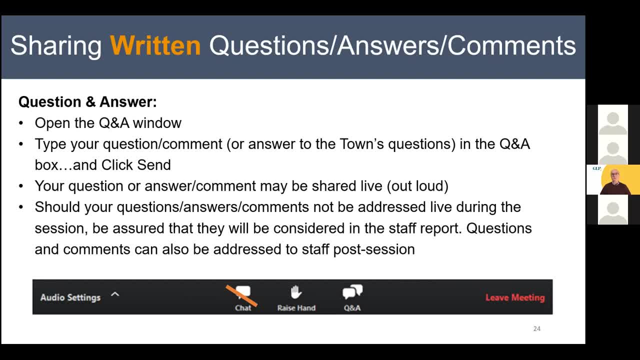 clearer About what it is that you're responding to. So, again, you can use the question and answer, written question and answer box or protocol to share your comments, to share your answers to the questions I'll be posing in a few minutes and to ask any questions that you might have. 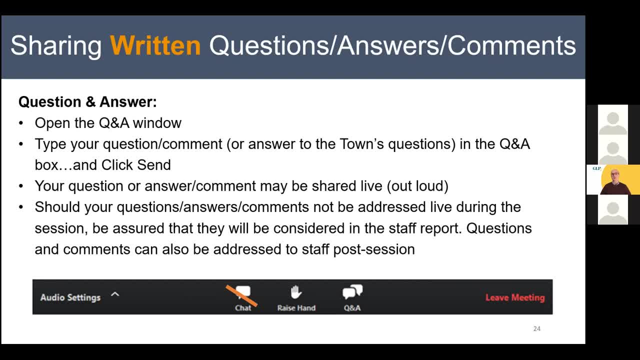 And some of those may be read out or shared live today. So just to give you a forewarning of that And also I wanted to note that if we don't get to all of the, the questions and things that have been sent through the Q and A box- which is likely because 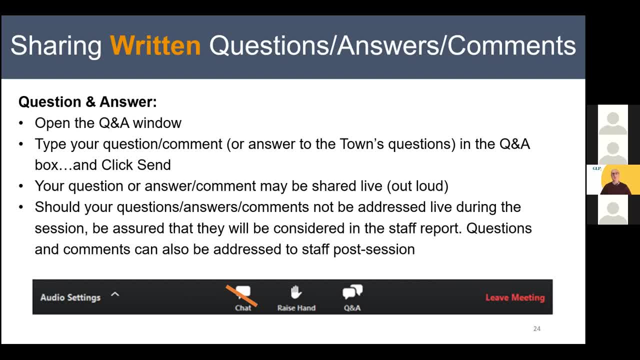 there's about 70 of you who were in this meeting, by the way, So we may not get to all of them. Do be assured that they will be included in the staff report, or at least or considered in the staff report, And that questions and comments can also be addressed to staff post-session And we'll talk. 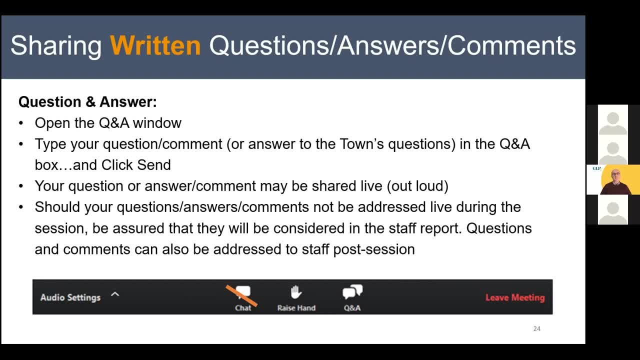 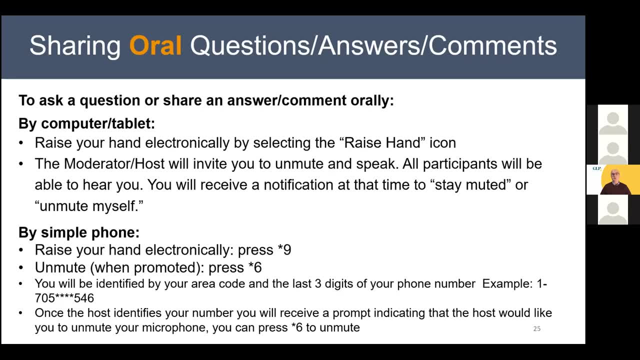 a little bit about that later as well. Now, if you'd like to share your questions, you can do so- your thoughts- orally, so not in writing, And the slide is up on screen now. So in other words, to have the opportunity to speak about the various things I've been talking about again. 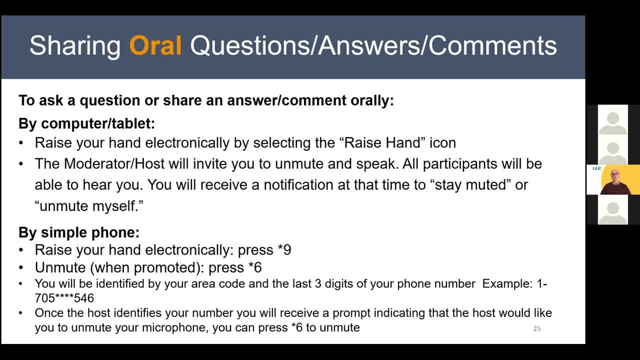 answering the questions, sharing your comments, sharing your questions. If you've joined by a computer or a tablet or a smartphone with screen capability, you can simply raise your hand electronically by clicking the raise hand button that is typically found at the bottom of the screen, And you can also raise your hand electronically by clicking the raise hand button. 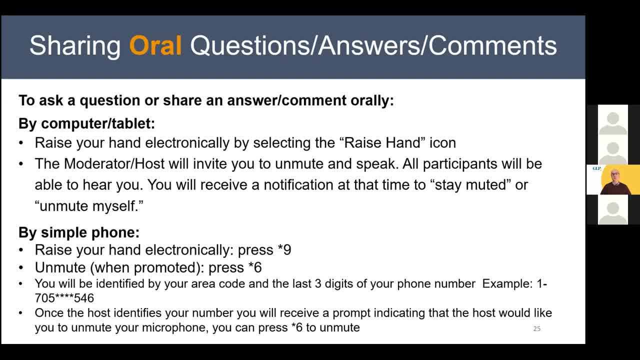 at the bottom of your screen. Some of you have already done that, So I know that you are able to execute that, Though this may vary depending on the device and whether you've accessed the meeting using the full Zoom program, the app or the browser. again, you should see the raise hand. 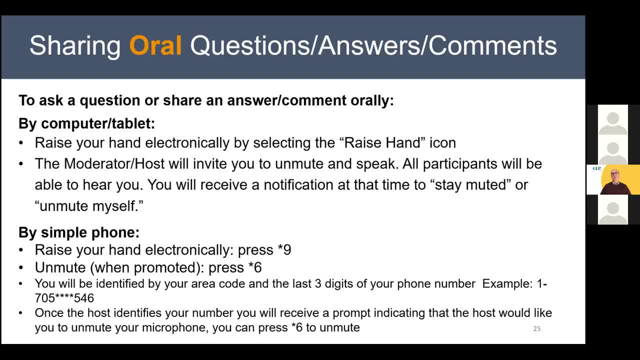 icon at the bottom of your screen And you can simply click on it and we'll get you into the queue to speak And, at the appropriate time, the technical manager will be able to answer your questions and we'll give you the permission to unmute and again to share your thoughts And 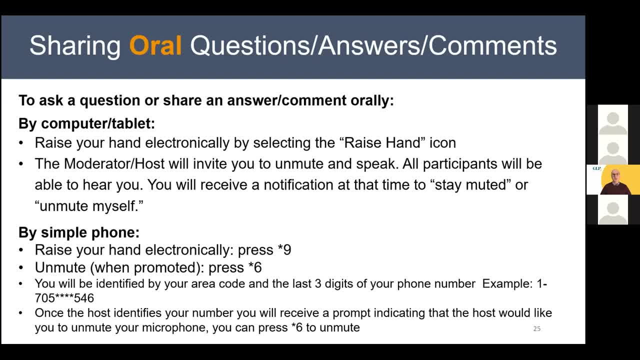 all participants, of course, will be able to hear you and you'll receive a notification at that time to stay muted or unmute yourself, and so forth, And if you've simply joined us today using a non-web-enabled telephone- so, an old-fashioned, simple phone- you can raise your hand. 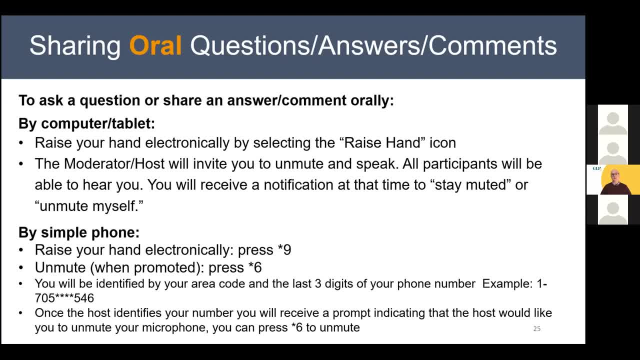 electronically by pressing star 9.. So again, star 9. if you're on the phone, or if you're on a phone that doesn't have screen capability, you can do it that way And you can mute and unmute your phone by pressing star 6.. If you're on the 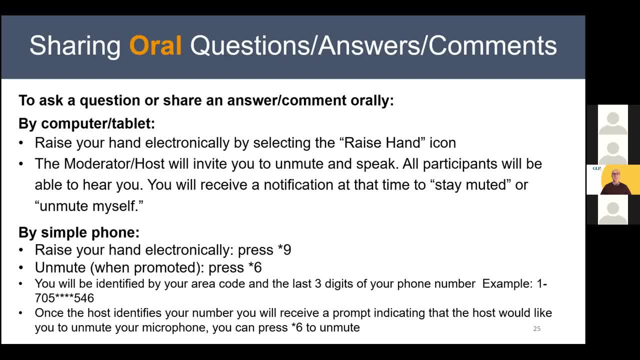 phone. we don't see your name or a screen name, We simply see a number. So we'll refer to the area code in the last three digits and that'll be your prompt to know that we're referring to you. And again, once you've been identified as someone to speak to, you can raise your hand and we'll. see that you're on the phone. So again, if you're on the phone, we don't see your name or a screen name. We simply see a number. So we'll refer to the area code in the last three digits and that'll be your prompt to know that we're referring to you. 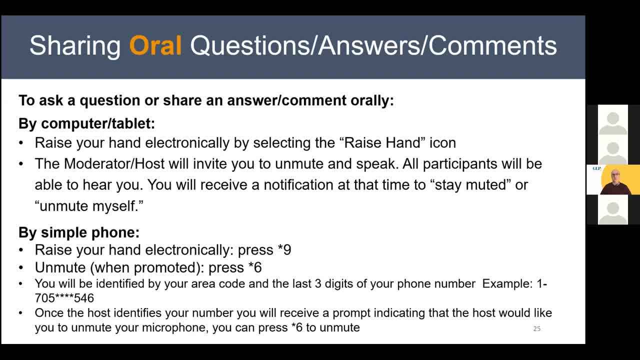 Please make sure that you unmute yourself, which, again, you can do by pressing star 6.. Okay, a couple of other things really quickly. If you are selected to speak- please be sure this is critical- please be sure that your own microphone is enabled- And that's different than muting- and 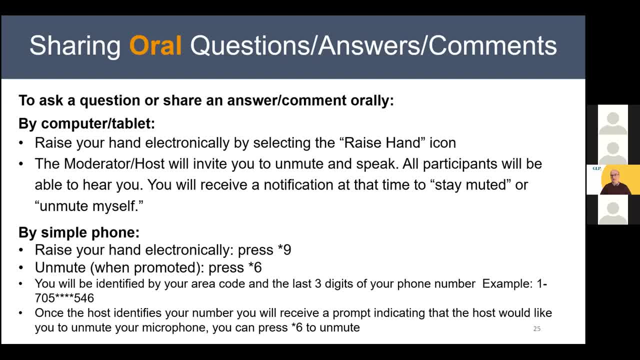 unmuting, You need to have enabled, through your device settings, your microphone to be used, So keep that in mind as well. And again, depending on how many people want to speak, we may randomly select people, but we'll more likely just take them. 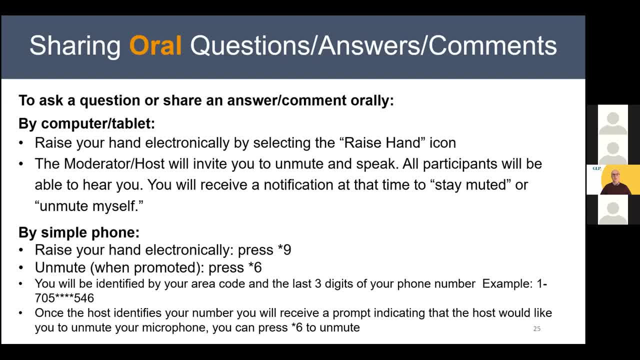 in the order that we see them. Once you've shared your thoughts, you'll be re-muted by the technical team and you'll return to being a meeting attendee so that you can continue to be a part of the session. And, of course, please lower your hand once you've asked your question or shared. 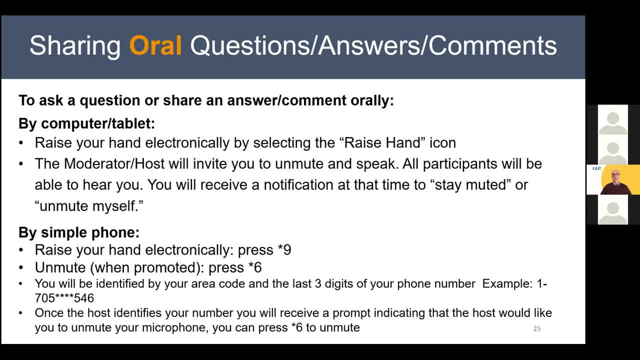 your comment And I'll ask everybody to limit themselves to just a few thoughts or questions, because we want to fit in as many people as possible. If, for some reason, we are unable to hear you or if we lose the connection, we will need to move to the next participant and we invite you to reconnect using 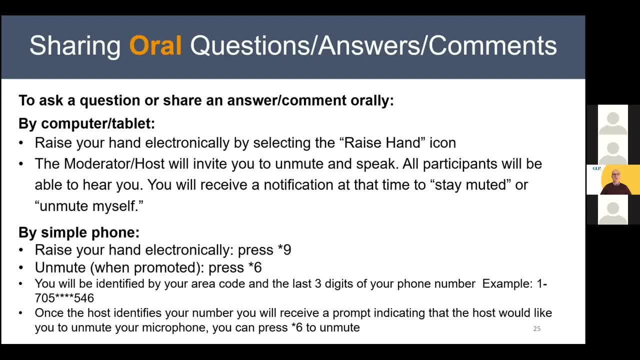 the Zoom link and or the telephone number provided, And again, we may not get to everyone this afternoon. Please remember that you can submit questions and comments through other means, So let's put some of the questions that the town is interested in getting your thoughts on on screen right now. So if we could put that slide up please. 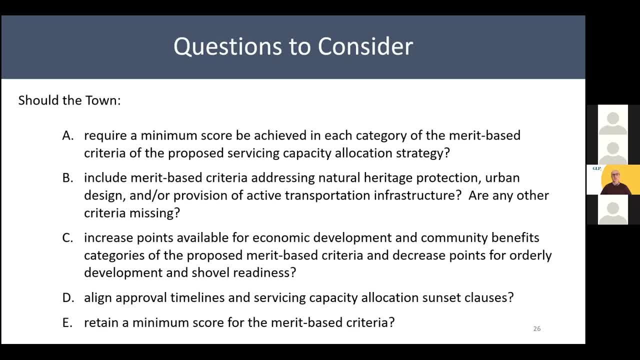 So you'll see that there are five of them, which have been labeled A to E. I won't read them all out, I'll just do a sample or two. For example, the town is interested in knowing should the town require a minimum score be achieved in each category of the merit-based criteria of the 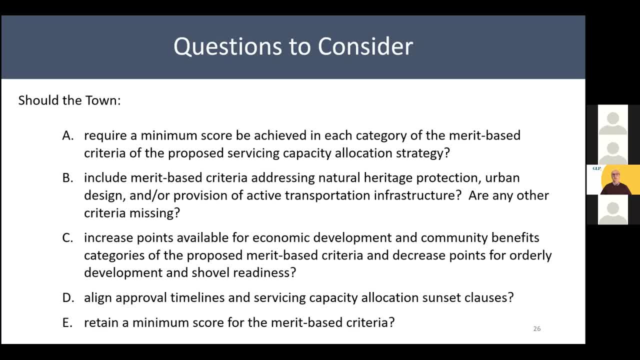 proposed service and capacity allocation strategy. I think there was a pretty strong response on that in the polls, but if you'd like to add some vocal commentary, the team would welcome it. And again, you see the other four questions. For those who are on the phone, I actually better read them all out. 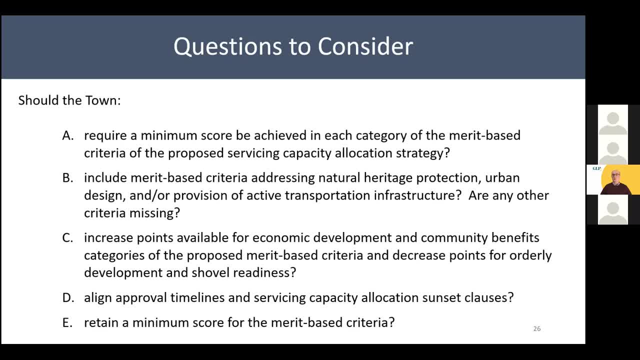 It just occurs to me, because you will not be able to see them if you don't have screen access. So question B is: should the town include merit-based criteria addressing natural heritage protection, urban design and or provision of active transportation infrastructure, And are there any other criteria missing? 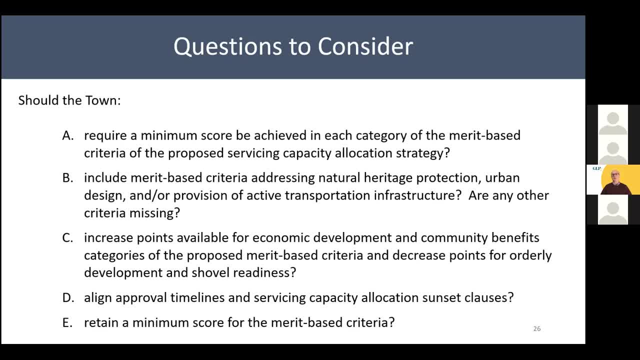 Question C and of course these are posed as sort of yes, no. but we're looking for more than your binary response. We're looking for your commentary on these. Question C: should the town increase the points available For economic development and community benefits? categories of the proposed merit-based criteria. 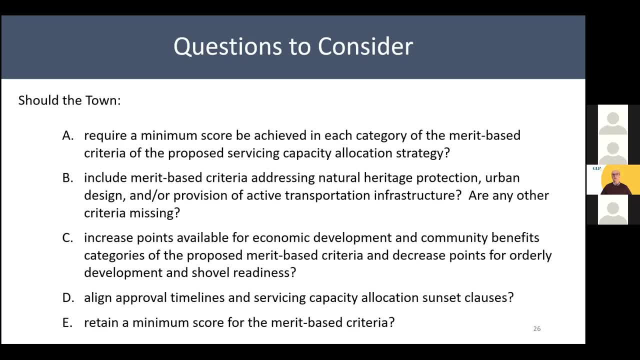 And should the town decrease points for orderly development and shovel readiness, Or perhaps other categories that you'd like to comment on? Should the town- this is question D- align approval timelines and servicing capacity allocation, sunset clauses And question E: should the town retain a minimum score? 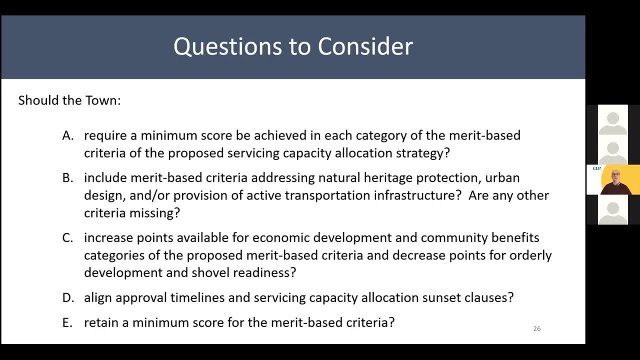 Or for the merit-based criteria. So let's move to hearing from some of those who have raised their hands or who have sent comments through the written Q&A box. Again, I'll ask each speaker to be as concise as possible. We want to hear from as many people as possible in the next 35 minutes or so. 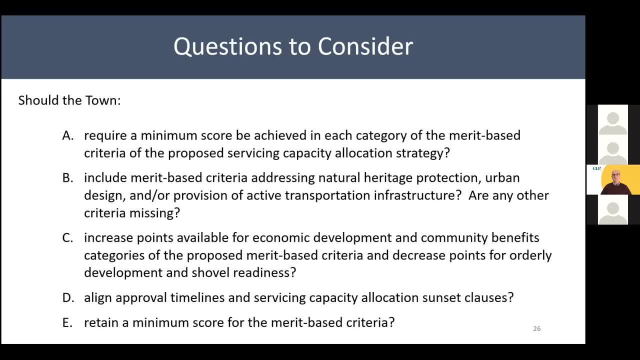 I'll invite each speaker to just quickly introduce themselves and perhaps let us know their location if they're so willing to offer that. So let's move to hearing from our first speaker now. The first person whose hand I saw go up was John Welton. 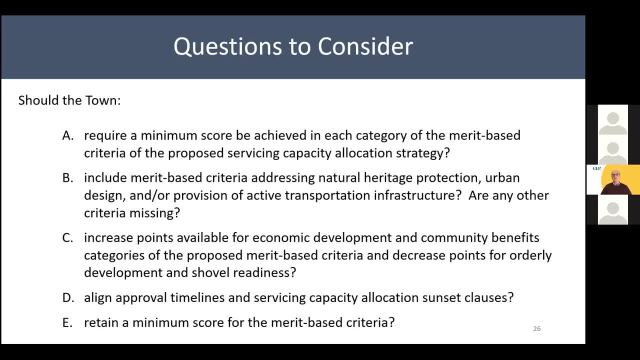 So, John, we will invite you to speak. Our technical manager will do that for you. If you would kindly unmute, go ahead whenever you are ready, John. Okay, I'm a little disappointed to know that there's 70 people and you're going to give us 30 minutes to provide input. 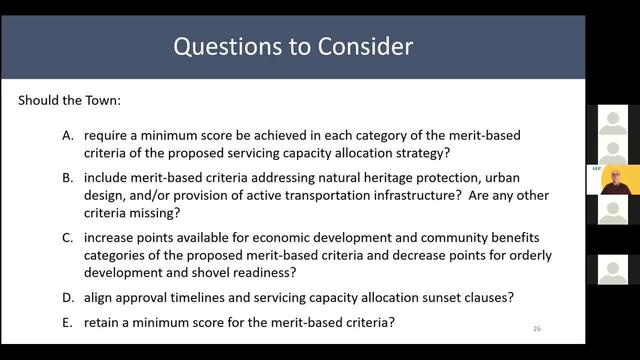 Because I have quite a few things that I need to put in. I'm very alarmed by this point system and that feels very threatening. We have a site that's just been through an LPAT hearing, that's fully zoned And we, like everyone else probably, tried to put in what we thought our development would score on the point system. 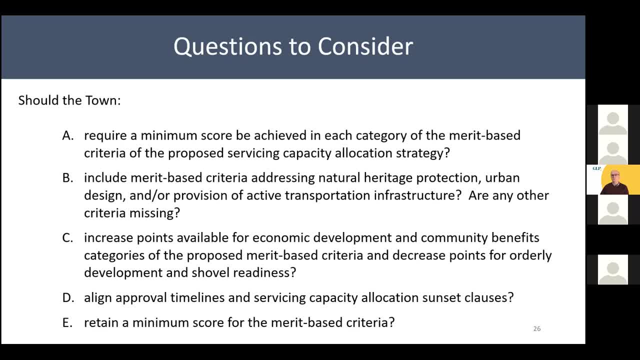 So we're shut out of a few categories in terms of infrastructure. Sorry. economic development is 10 points. I'm not sure how a completion of our 90-unit townhouse project can work on that. We can qualify for a portion of attainable housing, but our zoning doesn't permit some of the mixes that will give us more points. 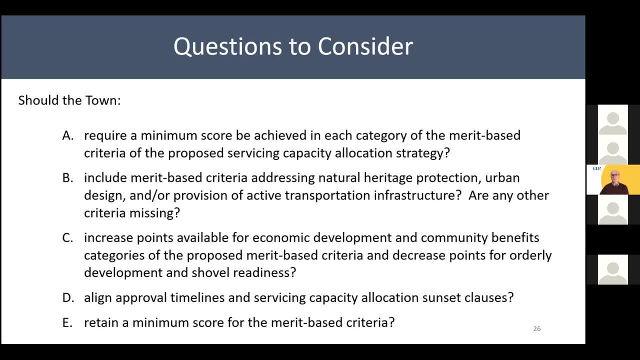 We don't have an opportunity for community impacts and benefits where we are. So we're concerned that the threshold of 75 points for approval is something that we can't meet, But we don't know who's. it's very subjective, these points. 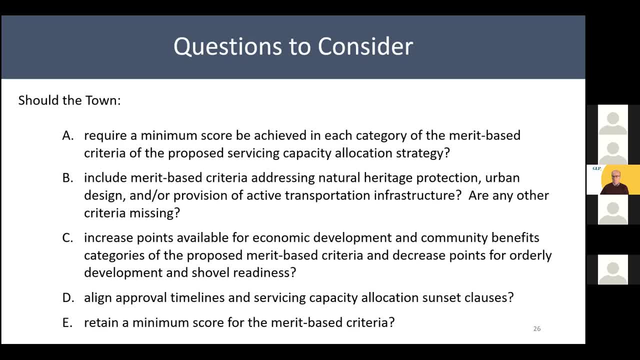 And we're wondering: is this a process where we sit down with someone from the town and go over these points totals together? Perhaps we might take some comfort to know that we're getting more points than we think we are. John, let's start with that. 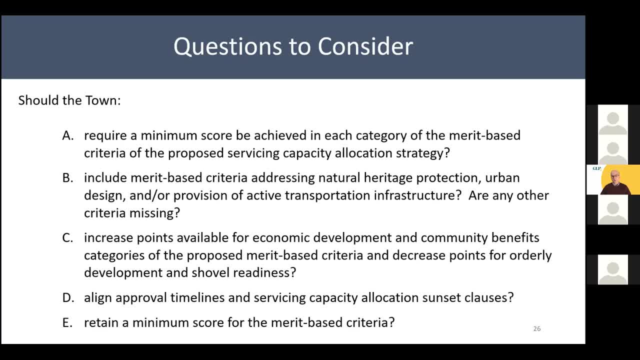 And then I'll come back to you in a moment. So John is putting on the table a concern about whether the 75-point threshold is attainable, And also about the manner in which the points allocation is made and the degree to which a developer or their representatives would be part of that process. 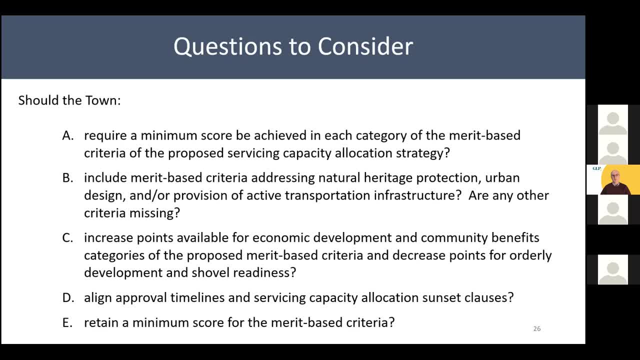 So, Nick or Summer, would either of you like to speak to John's initial comments And then I will go back to him And, by the way, everybody, we may extend this a little beyond 4.30.. We'll see how we're doing time-wise. 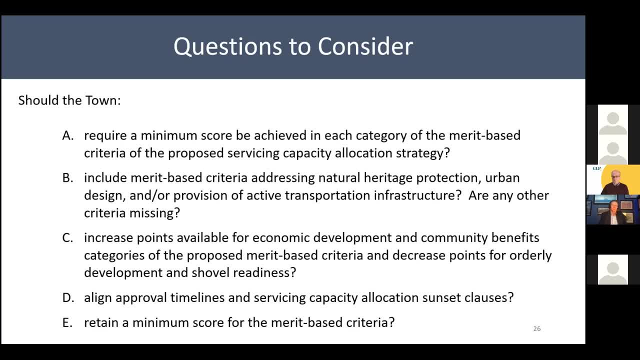 But go ahead, Nick. Thanks a lot, Glenn, And great question, And those are exactly the kinds of comments that we're looking to receive, And I certainly stressed at the outset that these are draft criteria. The merit-based approach is something I think the town needs to consider. 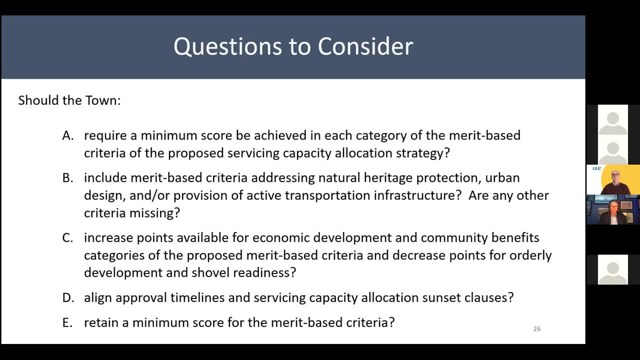 How it does. that is really what we're having this conversation for, So we're certainly interested in hearing that perspective. There may be other ways to get at the merit. There may be other ways to get at the merit-based approach that don't involve achieving a minimum score and do take into account some of the factors that you mentioned in your in your question and comments. 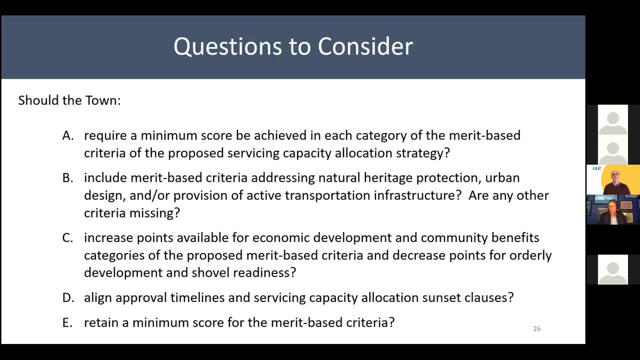 So thanks for that. We'll certainly be looking at that in some detail. And, Nick, what about John's point about the degree to which the developer would be involved in working with you to determine the points allocation Summer? did you want to add something? 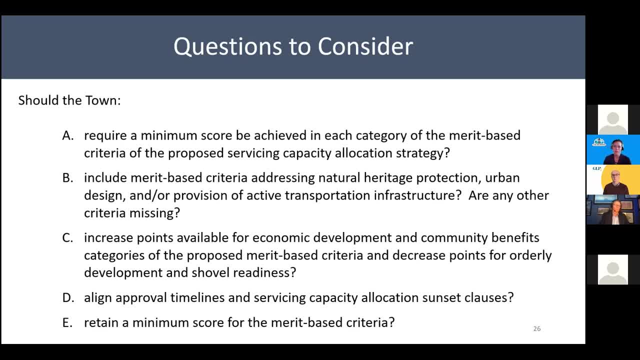 Go ahead, please. Thank you, Glenn, And to the individual who asked the question. I appreciate the comments and certainly, as Nick mentioned through his presentation, depending on where we land with what the policy looks like, we'll have to have subsequent discussions about how it's implemented. 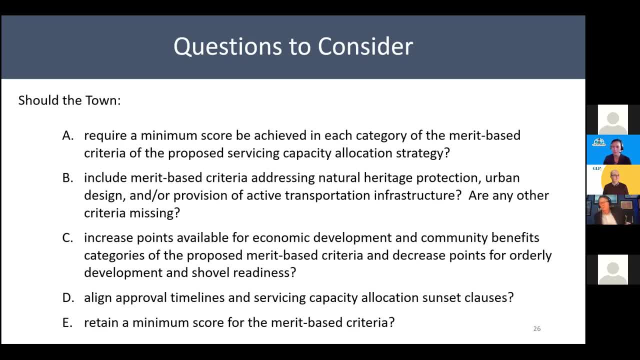 But with anything related to land use planning in the town, there's certainly a partnership and an open discussion between the applicant and staff, and as well as the decision makers around the council table, So I don't expect this process to be any different than that. 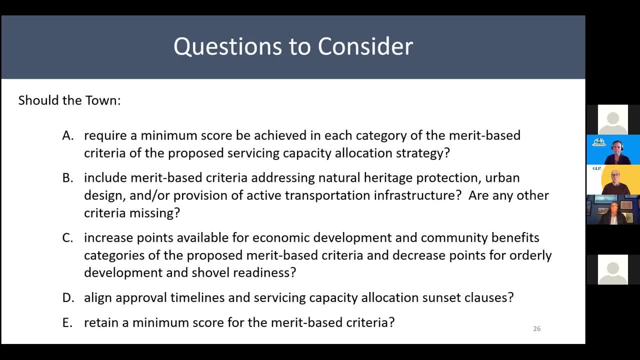 Okay, John, Back to you. You had one or two more things before we go to someone else. Yeah, So I mean, we're being asked to consider that this is being fair and transparent, And until we get the answers that I've been looking for, I'm not sure how I understand it to be fair and transparent if it appears that your project can't make the points total. 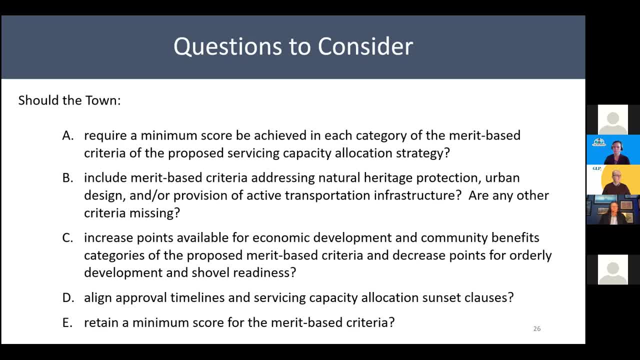 And so, and why would we support it if we couldn't? I would like to know what your definition of a brownfield site describes. I would like to know what your definition of a brownfield site describes. I would like to know what your definition of a brownfield site describes. 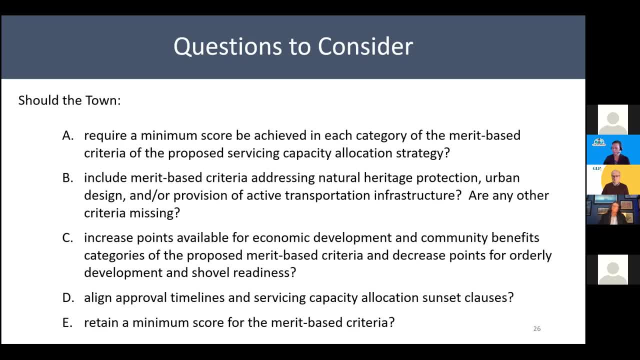 Right Definition is because my understanding would be that it would be cleaning up something that was previously built, perhaps something industrial, commercial, because that's somewhere where we don't have the opportunity to gain any points. What is what do you consider a brownfield? 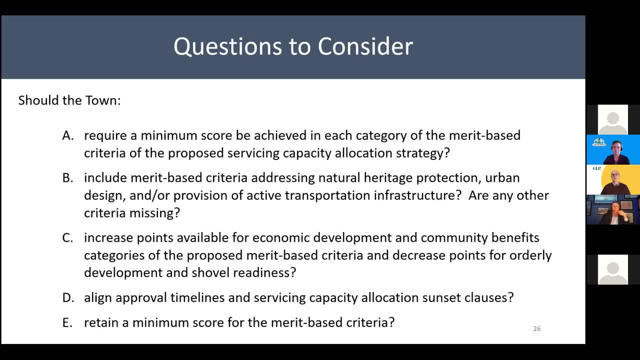 So Nick Summer, who would like to kick us off on that one? Thanks, Thanks, John, And by the way, James Orr, you will be up next. You're on deck. Go ahead, John. I guess an answer to your question. 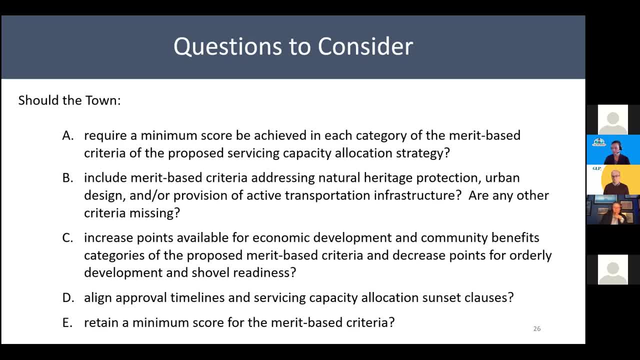 I don't have a clear answer for you. I know that certain funding is available for sites if they meet certain criteria and are considered to be a brownfields. whether that's what we want to apply here or not is a discussion item. perhaps a broader definition of what is brownfield may make sense. 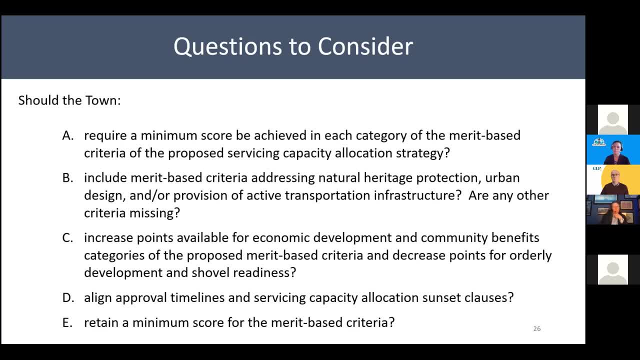 in the Collingwood context, and we're certainly open to that. Okay, the last item that I'd like to ask would be what's considered economic development, because when we look at the 10 points that are offered there, we don't see an opportunity to earn any points for developments. 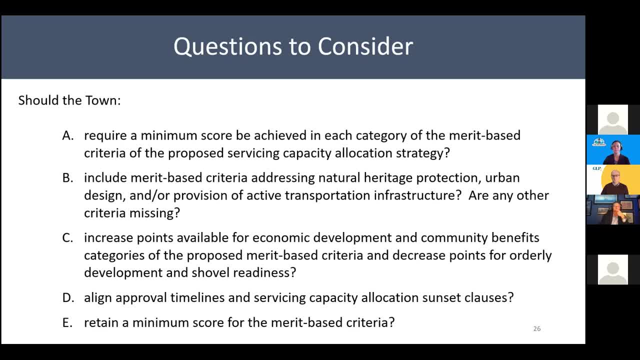 that add a significant number of new jobs to the local economy or enhance the downtown. I mean something downtown can get up to 10 points on that, Okay, so who can speak to that? what's included in the economic development category? thank you, John, for the questions much. 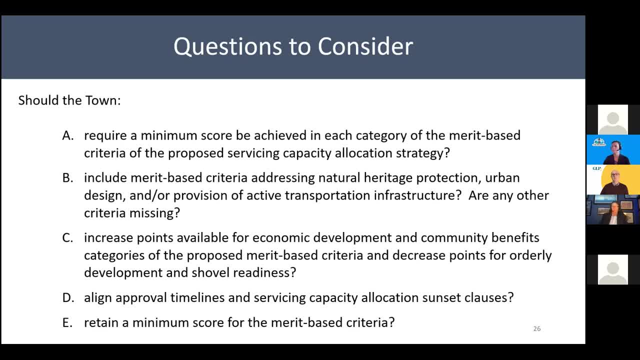 appreciated. Yeah, so the two, the two criteria you met are the two criteria we have in that bucket at the moment. certainly, job creation is always important and is something that we've reflected in here, and if a development is downtown or on a main street, we've also reflected that here as well. 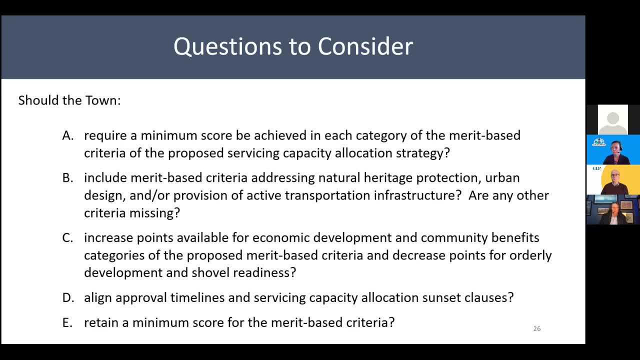 it reflects the broader focus the town has on encouraging job creation, of course, but encouraging development in in key areas like the downtown. There may be other economic factors to consider and we're certainly open to any suggestions, but those are the two that we've come up with at this point. 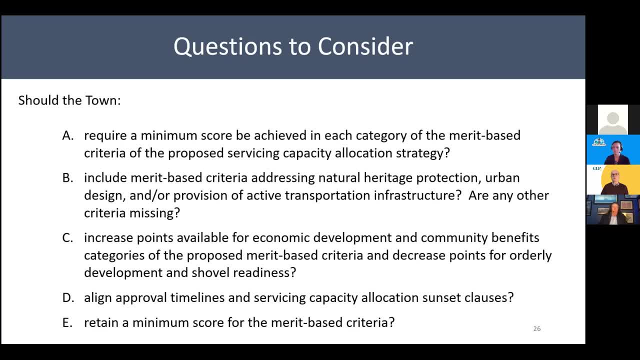 Okay, thank you, Nick, and again thank you to John for his question. so James Orr is next. again, I'm going by screen name, so James will invite you to unmute and please share your comments and or questions or answers to the town's questions. whenever you're ready, James, go ahead please. 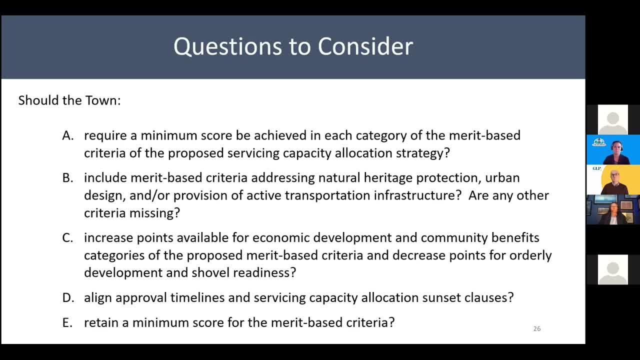 Thank you, Glenn Summer and Nick, for your content presentation so far. In reviewing the draft policy, I'm finding that there is no specific language or clauses, particularly in section A3, that address a change in tenancy or building use or repurposing that does have associated increases in water or sewage demands but does not trigger a planning act application. 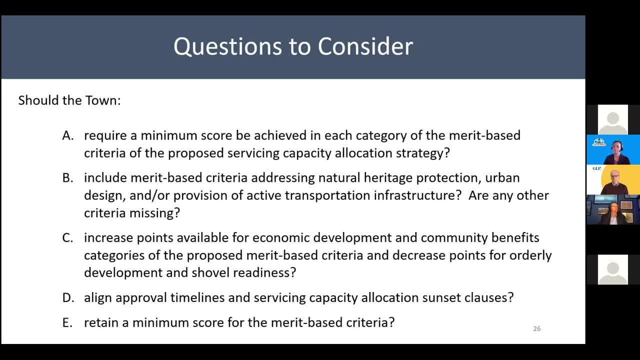 So that's a good question. Okay, thank you. So IEA permitted use under the current OP and zoning by-law and within the town's engineering standards. So from my read, this is left up to the CBO's discretion at building permit stage. 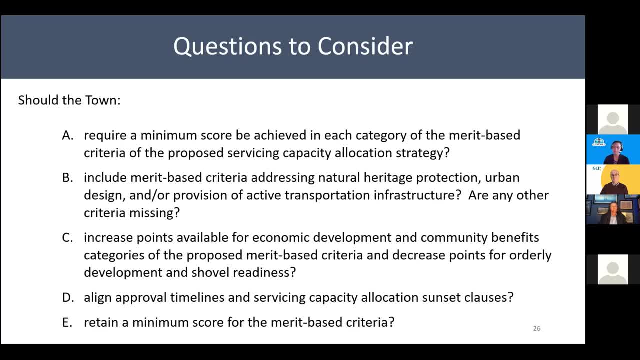 per the proposed zoning by-law amendment that's been discussed. So in this instance, if reserve capacity is available at the time of the application, would a repurposed or a retended thing essentially be competing with other applications for new development? subject to review. 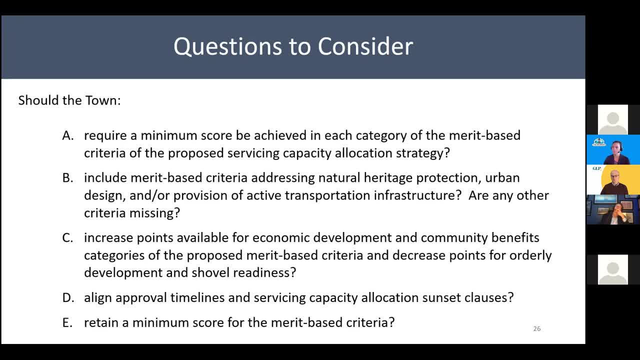 under the Planning Act, which doesn't seem to be an apples to oranges comparison and would be concerning to me, Thank you. Thank you, James. Yeah, these are very purposeful and on-point questions. Thank you for them. So, Nick, how would you deal with a change in building use? 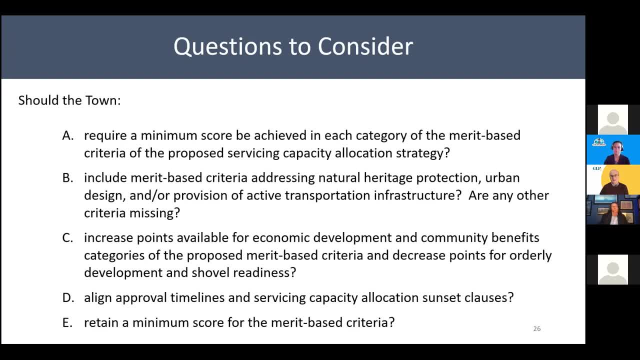 a repurposing. How do you reconcile all of the things James just mentioned? That's a very fair comment And I guess, as a general principle, our thinking is that anything that increases water usage or sewage flows would be the subject of the policy. 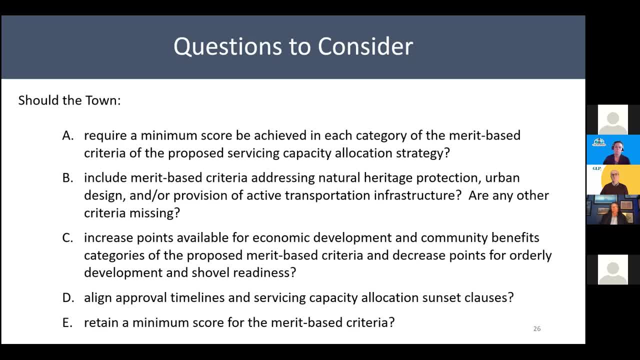 unless it's specifically exempt. That's the way it's set up now, But perhaps we could consider other types of exemptions, such as what you're proposing, which is a repurposing of an existing building. At the end of the day, 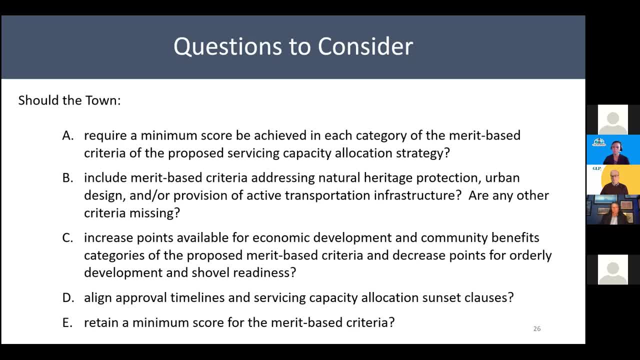 when the by-law is amended as recommended, it will give the chief building official the ability to make decisions on whether a permit can be issued, And we do know we need to do some thinking on that internally in terms of how exactly that is to be determined. 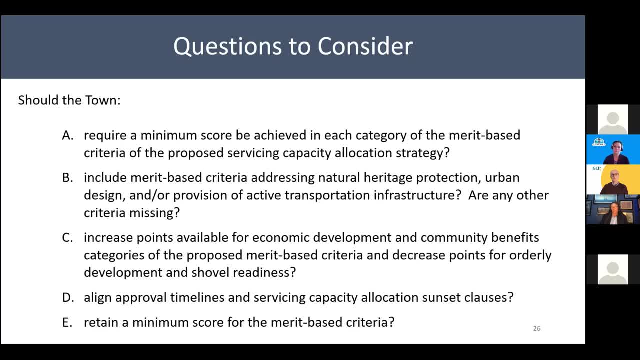 by a chief building official through this process. But thanks for that comment. Really appreciate it. Thank you, James. So Don Reed is next. Again, we will invite you, Don, to unmute yourself And whenever you're ready, please go ahead with your question, your comment. 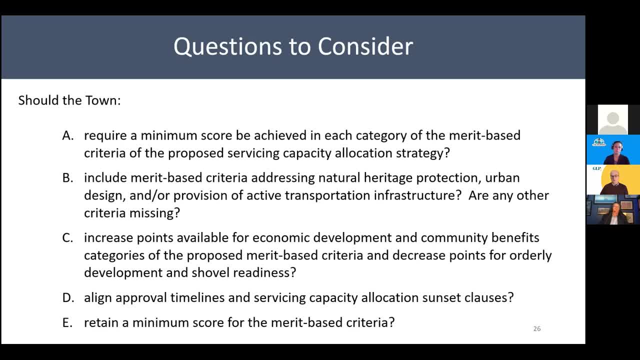 or again, perhaps an answer to the questions that the town has put on the table. Don, go ahead whenever you're ready. Okay, thank you very much, Don Reed, from Niagara Street. We fall into the category of lot addition, where land is taken from one lot and added. 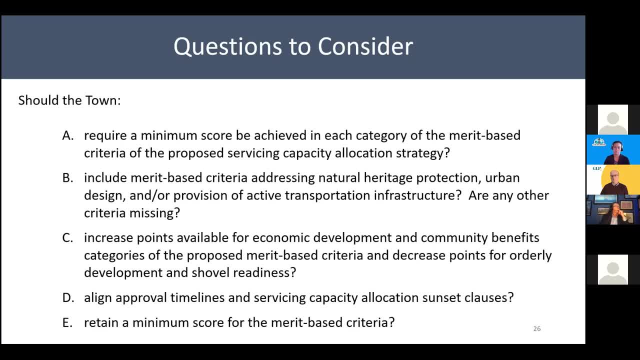 So basically we're severing a lot right now. We got hung up by the ICBL last March and just got through the Committee of Adjustment on October And now we have a year to complete the conditions, to complete the severance. I've spoken with water and services. and they won't be able to do their services until the spring of 2022, at which time we'll be at the beginning of the summer and when we can finalize our severance, which could theoretically delay our ability to build until 2023. 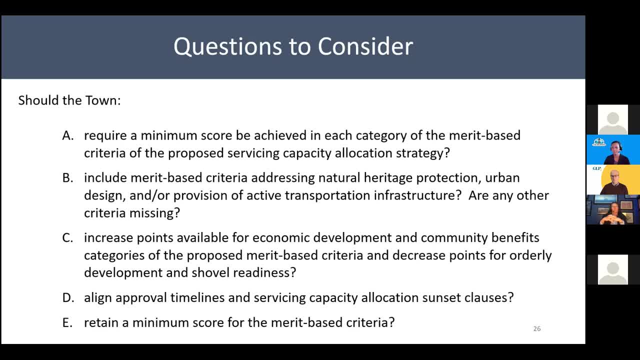 We currently hold an ICBL exemption. So I'm concerned about the phrase and the phraseology of shovel ready in terms of the natural progression of our development. We're just residents, we're not developers. What will happen to us? our ICBL will expire while we're just in. 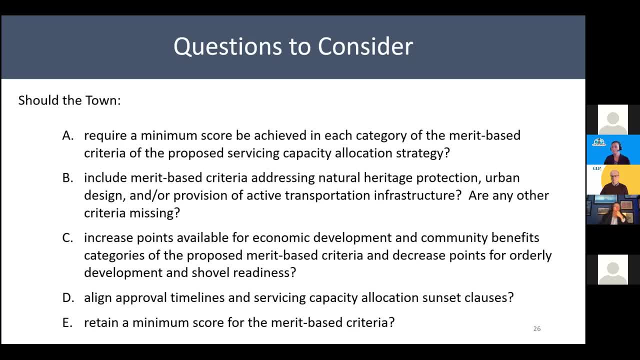 still in the process of trying to build, So we're concerned about that. Like we want to be able to continue on with this, So I'm just wondering what your comments might be about that. Yeah, so thank you. Let's invite Nick or Summer in. 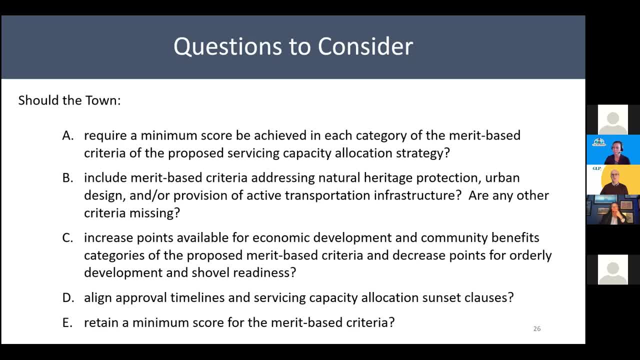 So the concern about shovel ready and what it might mean to somebody who's in Don's situation And Don do you mind muting? We're getting a little bit of feedback, Thank you. Okay, Where is that? Or we can mute you on this end as well. 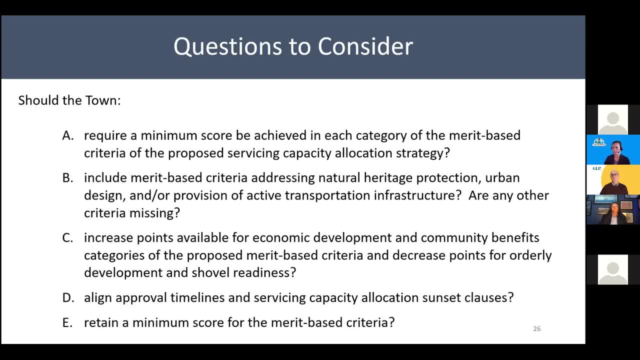 Thanks, Don. So go ahead. Thanks, Don. Yeah, great question, Don, And I'm not going to be able to give you an answer. It is very specific to your circumstance And I would suggest you reach out to Summer, after this meeting, to have that more detailed conversation. 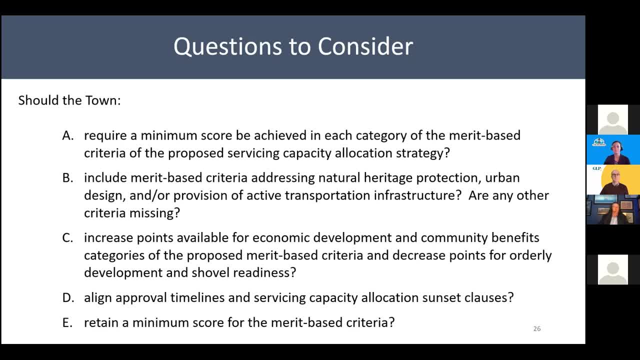 But you do raise a good point, because I did make it clear in the presentation that the policy would apply to anyone who got an exemption but didn't proceed to building permits. So that's what we're proposing, and certainly feedback on whether that makes sense or not is what we're looking for. 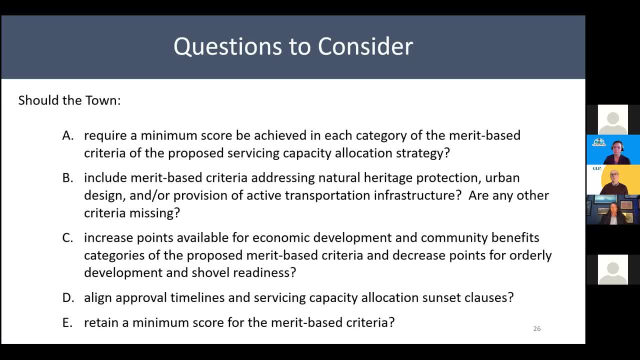 Thank you again to Don for the question. So I'm going to go to Leo Longo in a moment, but we also have, I understand, a couple of questions. I understand a number of people who are sending comments and questions through the written Q&A. 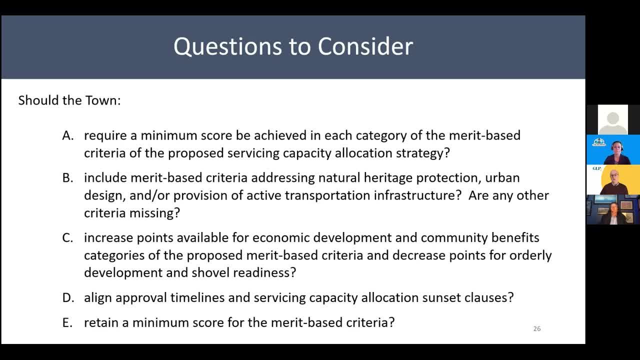 which, of course, I invited you to do. So what I'm going to do now is actually ask the community planner with the town of Collingwood, who is Nathan Wukash, And Nathan, I would say, let's just share questions at this point. 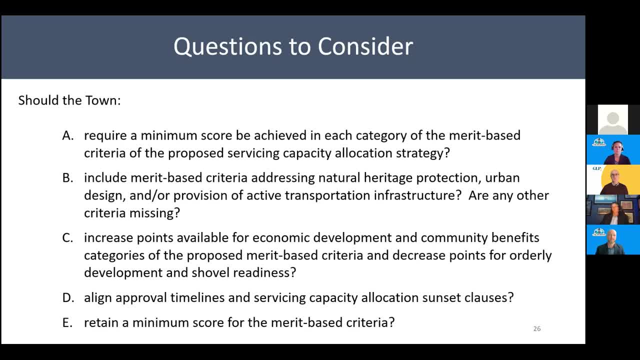 because we you know the comments and the answers to our questions. we can collect and review afterwards, But let's focus on the kinds of questions that are coming in, So why don't you share? There are a couple that have come through the written Q&A. 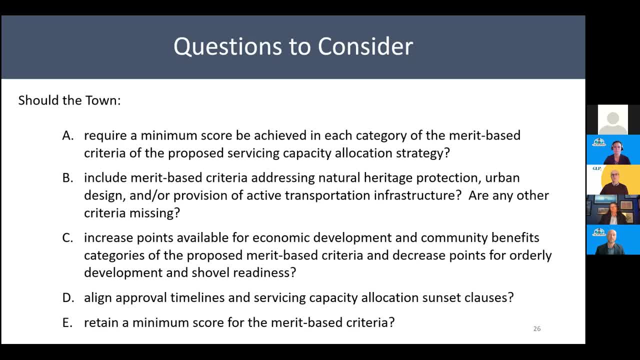 and then we'll go back to Leo Longo afterwards. Go ahead, Nathan. Thank you, Glenn. Yeah, the first question we have is from Mark Epplett, And the question is: how long will it be until the need for allocation criteria would not be required? 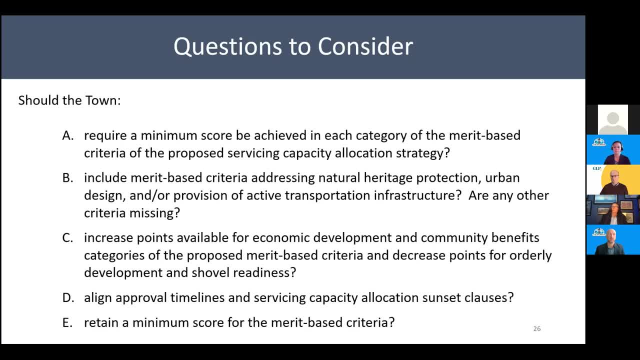 And when will the upgraded system be ready and what will be the new capacity? So that's probably a question that Director Slama could participate in, and also maybe Summer as well. Director of Planning. And for those of you who don't know her, that's Peggy Slama. 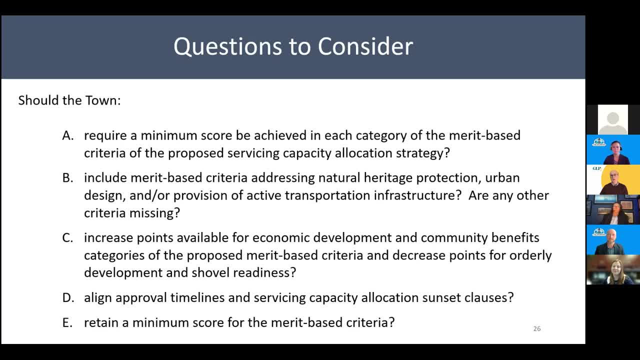 who's the Director of Public Works and Engineering? And again, Summer Valentine. you heard from earlier, But, Peggy, do you want to kick us off on that one? Yeah, sure Thanks, Glenn. Yeah, I can answer the question with respect to the water treatment. 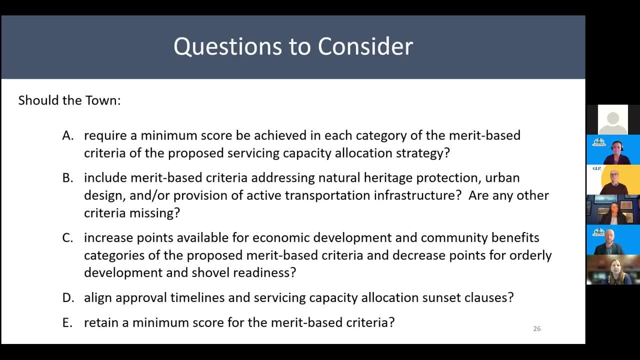 plant and expansion and looking at additional capacity at the water treatment plant. So Staff have been working diligently this year to advance our water treatment plant expansion And in the last few months we have we are working through the first step, which is, as approved by Council, to look. 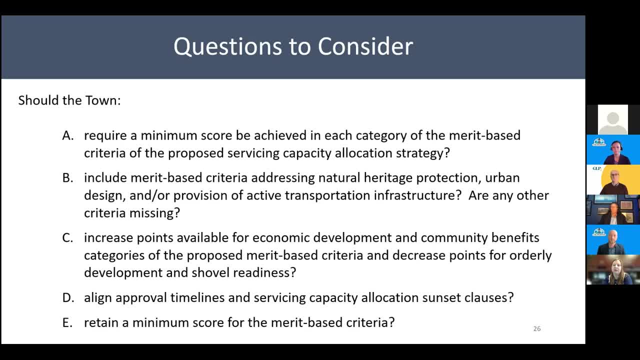 at the installation of additional disinfection so that we have we're restoring our rail, our Our available winter capacity at our current water treatment plant And we are on schedule for that installation to be installed be in place in 2022.. 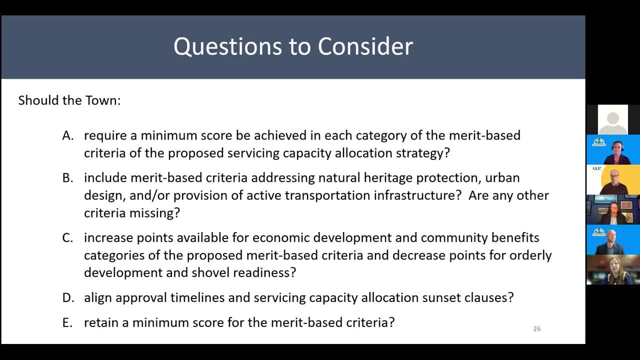 And it should relieve our winter restrictions in winter 22, 23.. With respect to the water treatment plant expansion, we remain on schedule to have you know additional capacity available before December 2025, at this time. So the way we are considering the construction, 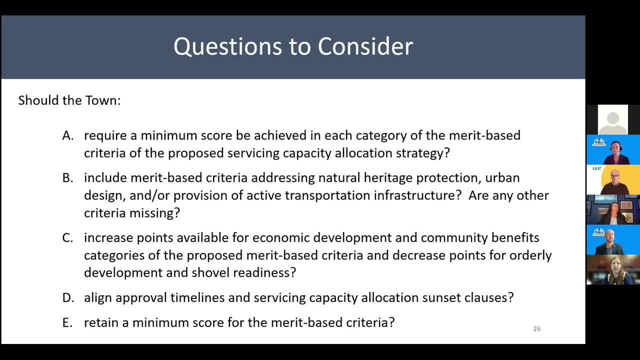 of the water treatment plant expansion is that we're looking. we're trying to facilitate additional capacity being available before the end of 2025. But the actual plant expansion won't be complete until summer 2026.. But the key thing is having small companies that are available and 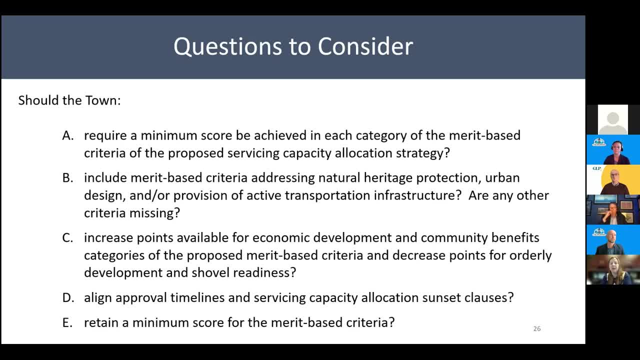 asking for Whose participation having that additional capacity online before the end of 2025.. We had indicated previously that the water treatment expansion would bring us from 31 megalitres a day- our plant capacity today- to 52 megalitres a day. 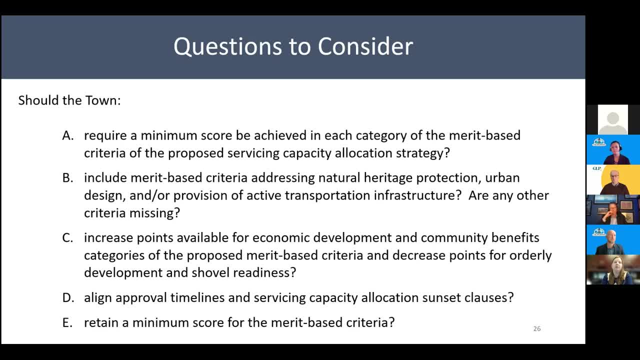 And in working with our consultant and refining our requirements for the types of treatment that we're looking at with the facility. we're hoping that the phase one expansion will be 58 megalitres a day, So that would be 58 megalitres a day before the end of 2025. 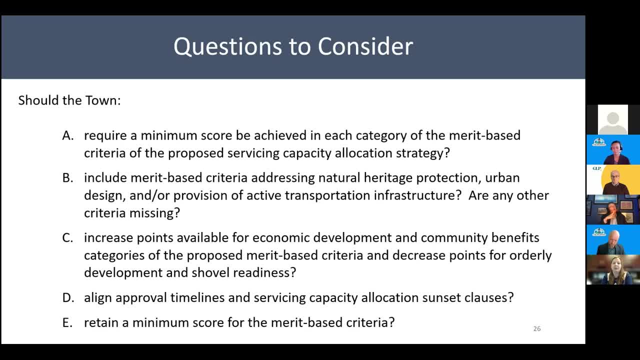 It's an aggressive schedule. so I will qualify that And we are, as I said, our staff and the consultants are working diligently to meet that. but I will say it remains an aggressive schedule. I'll let Summer, if you want to answer the question about you, know. 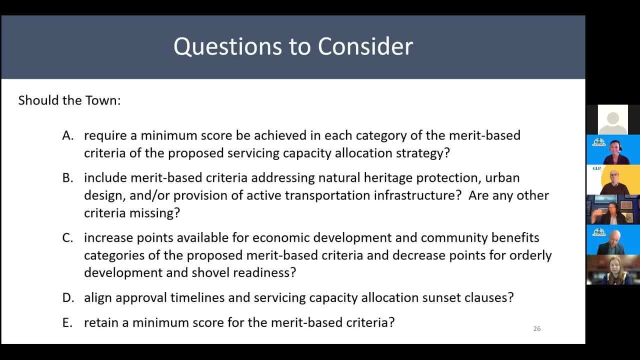 when the first question, which was Nathan, what? When? the allocation? yeah, okay, Yeah, when the framework wouldn't be required anymore. Go ahead, Summer. Yeah, thank you, And I'll be as brief as possible, recognizing that I think we still have eight people. 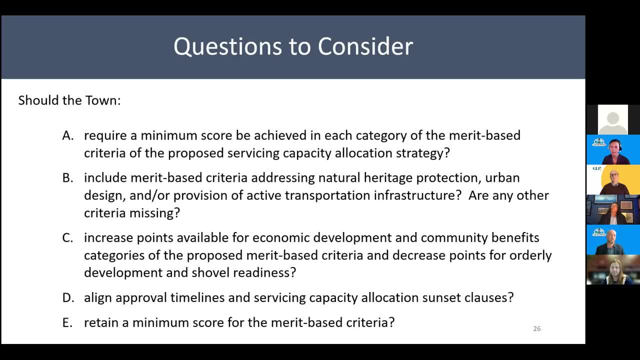 with their hands up that we need to get to. So the policy, as it's currently written, allows some merit-based criteria to be applied in two cases. One, when there's limited capacity, So in the timeframe that Peggy was speaking about, where the plant is being upgraded. 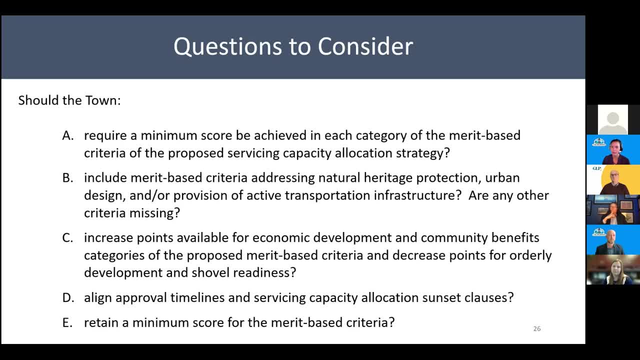 once the plant is upgraded, that limited capacity criteria wouldn't be met. And second is when there are competing proposals. So even in a case where the plants are fully functional and capacity is not limited, there may be some reason that within the system. 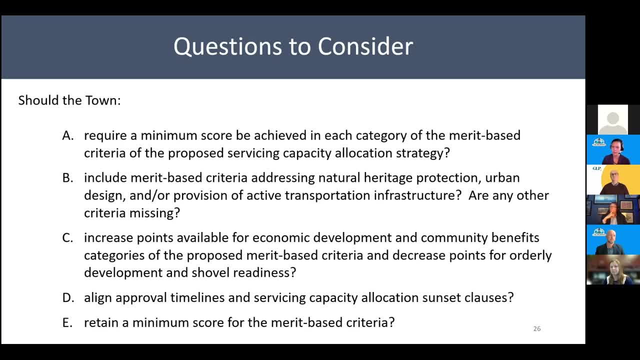 say, a part of the infrastructure that's serviced by a pumping station. beyond that pumping station there's only a certain amount of capacity available and there's competing projects for that area of town, then the merit-based criteria could be used. So I think it's important to think about that as well. 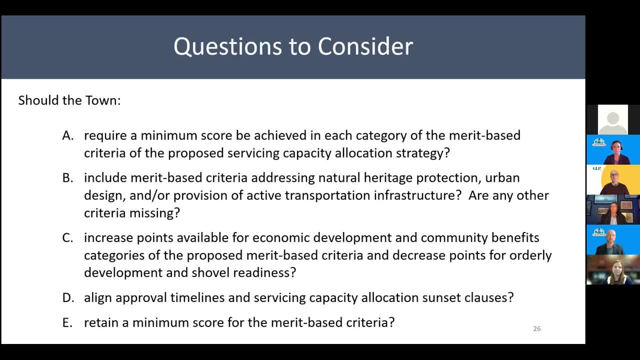 And I think that's what we need to be thinking about in those circumstances. Okay, thank you. So let me go back to Nathan. We'll take one more question from the written Q&A and then we'll go back to Leo Longo. 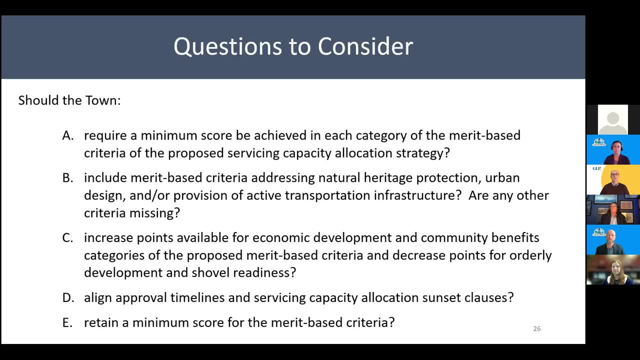 who I know has been waiting patiently. Go ahead, Nathan, And I'll ask all our responders: please be as brief and concise in answering as possible, so that we can maximize how many voices we hear from. Go ahead, Nathan. Thank you, Glenn. 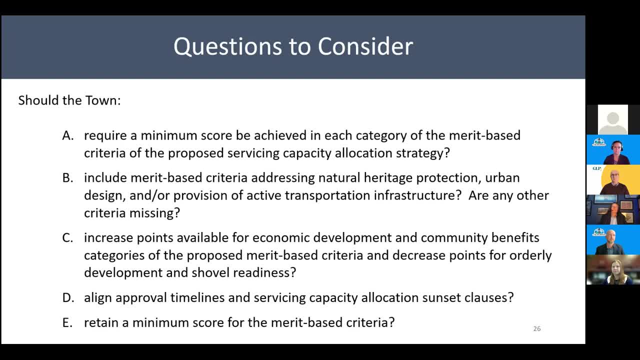 The next question we've got is from Fred Seraferro and it is part comment, part question, But the question part is: do you think it's a good idea to have more people in the community who are more likely to be affected by COVID-19?? 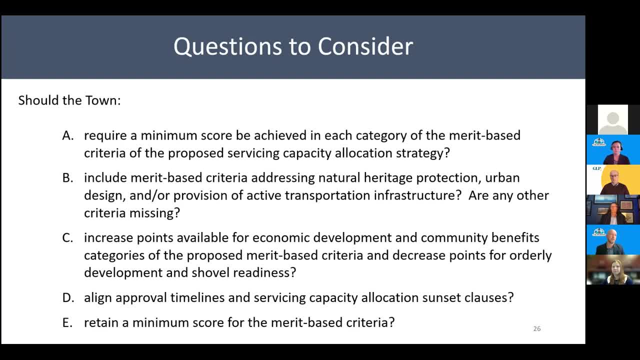 The next question we've got is from Fred Seraferro and it is part comment, part question. But the question part is the threshold for 75% scoring is quite high given the proposed categories. How is the scoring going to be conducted? 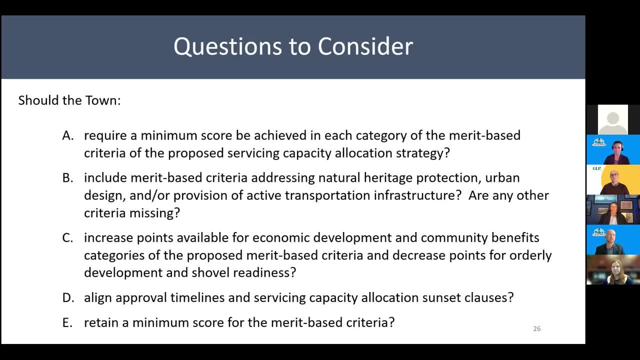 Okay, so Nick Valentine, or Summer rather Valentine, how will you conduct the scoring? Yeah, I think Summer gave a partial answer already in that, if this approach is accepted, the town would be working with the developer on a case-by-case basis. 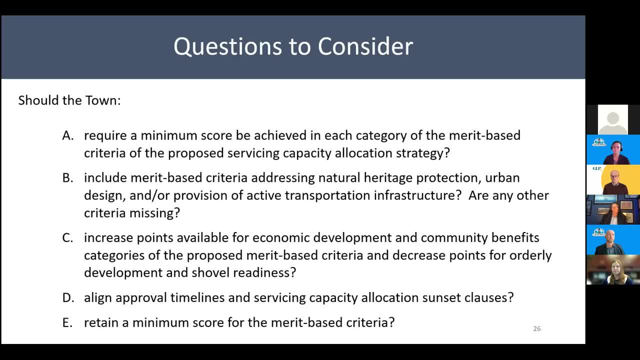 to determine how the points would be assigned and scored. I certainly do see a finessing of the wording as it currently sits to provide additional clarity. But, as Ms Valentine indicated, the town works closely with developers to achieve common goals and that's what I think will happen here. 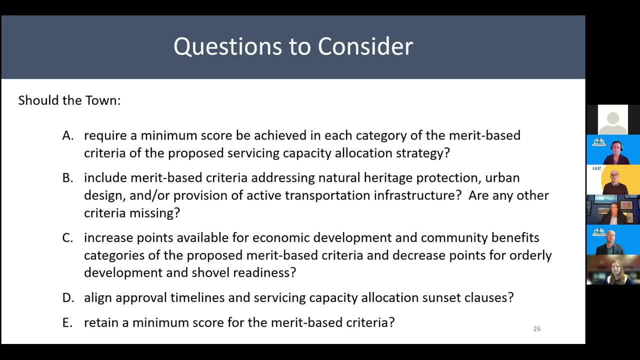 Okay, thanks, Nick. So let's go to Leo Longo. Again, I'll invite our technical manager to invite Leo into the conversation. And, Leo, if you would kindly unmute and go ahead whenever you're ready? Thank you very much, Glenn. 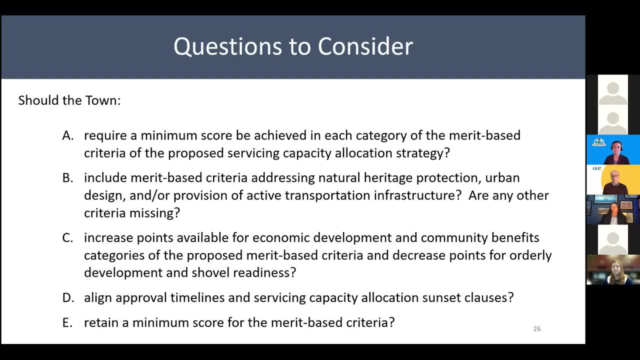 Just based on that question and answer that we just dealt with. my question did deal with implementation. should a criteria system be established? The first question would be: would there be an expectation that the landowner, development developer, would themselves, self-assess, assign a number? 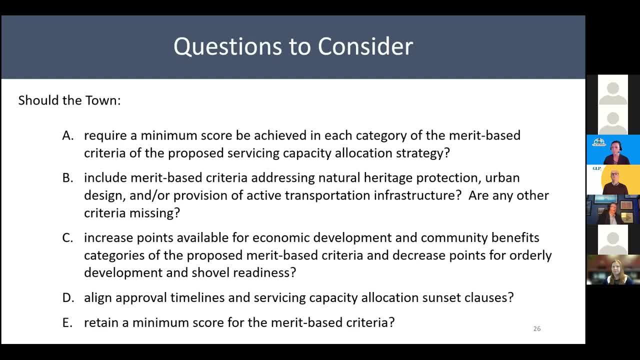 and then present that to staff. Second question is who on staff is going to be the one reviewing that and or assigning numbers? Third question would be: if the assignment by staff is lower than whatever the minimum criteria is, will there be an opportunity? 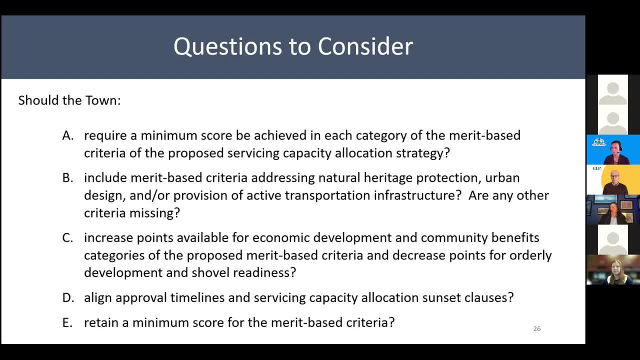 to advise the applicant to sharpen their pencil and maybe go back to staff. And then, finally, who makes the final decision as to what the score is? Is it a staff person? Is it town council? Those are some of the implementation questions I had. 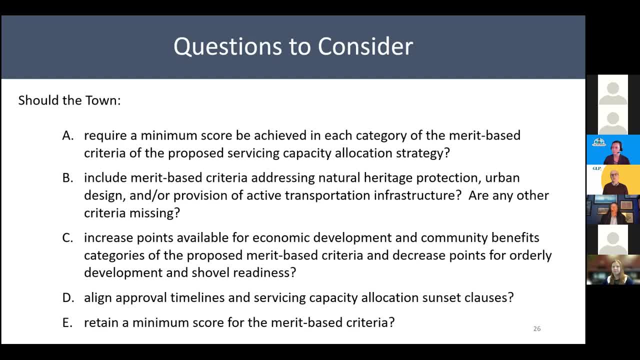 Thank you. Okay, thank you. So let's break those down and see if our response panelists can address them. So, first of all, is there an expectation that the developer or their representatives would do their own self-assessment and submit that? 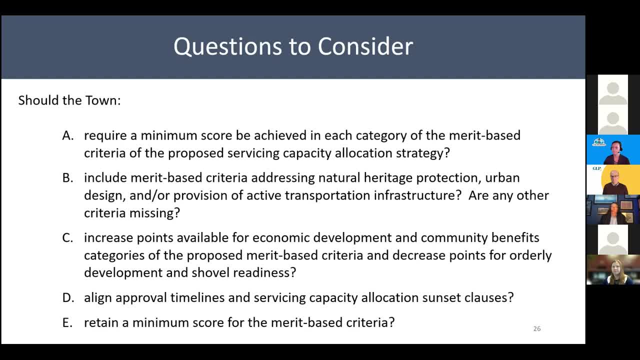 I think the simple answer is: I expect them to do it. Whether we expect them not to do it, it'll happen. We know how the development industry works and they will do everything they can to do that, So I anticipate that that will be part of the process for sure. 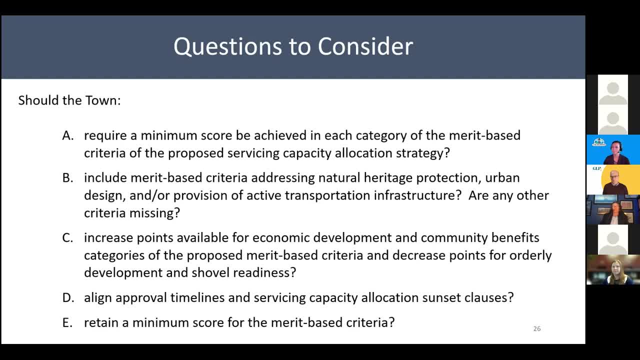 Okay, so if they do that, then I think Leo's next question was: who will review what they've done and actually make the determination as to whether, from the town, they agree with the developer's assessment and what if there is disagreement? So for those three questions, 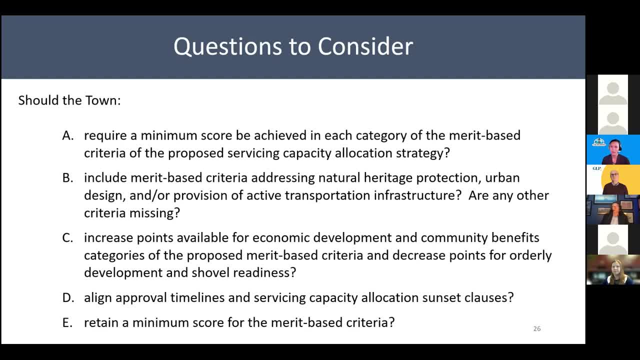 I'm going to hand them over to Ms Valentine to answer. Okay, thank you, And I imagine on staff it will be somewhat of a team effort. Some of the questions are more related to planning, Some are more related to infrastructure. 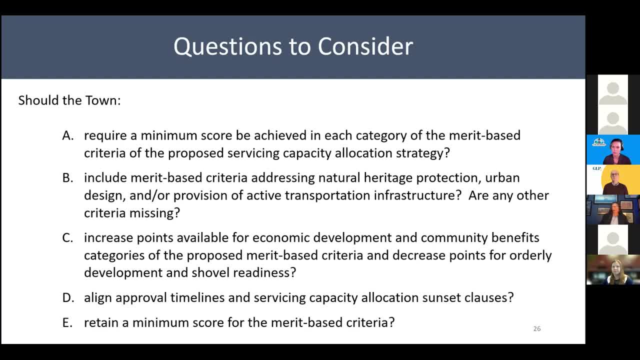 So we would have representatives from the engineering group and the planning group looking collectively at the scoring. Just looking at- I tried to make note of all your questions, Leo. And would there be an opportunity for staff to go back to the developer and ask them to sharpen their pencils? 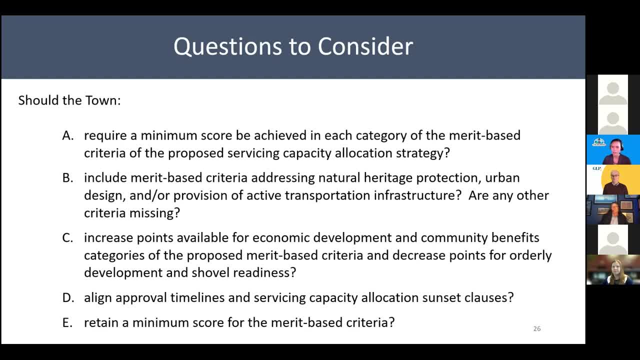 I think that this is part of the normal sort of discussion that would happen through the pre-consultation or application phase, So I expect that that opportunity would be available And to who makes the final decision Ultimately for a Planning Act application. 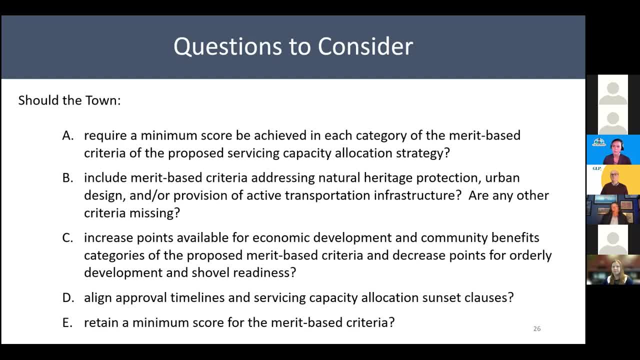 those would be going forward to Council. So in the case of a disagreement between staff and the developer on what the project should score ultimately, the staff report would reflect that And the developer would also be provided with an opportunity to address committee and Council through that process. 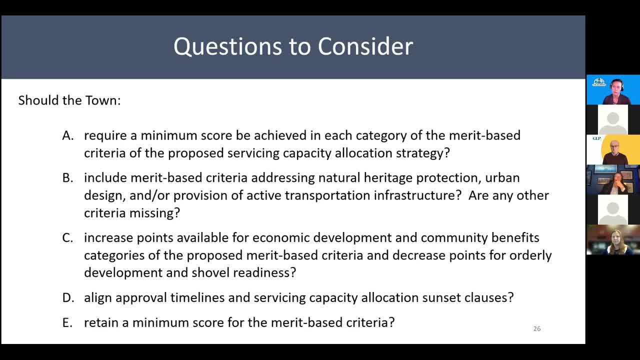 And ultimately Council would be the final decision in the case of a Planning Act application. Okay, thank you, And thank you again to Leo for the four or five questions. So, Chris Mattson, you are next. I'll invite our technical manager. 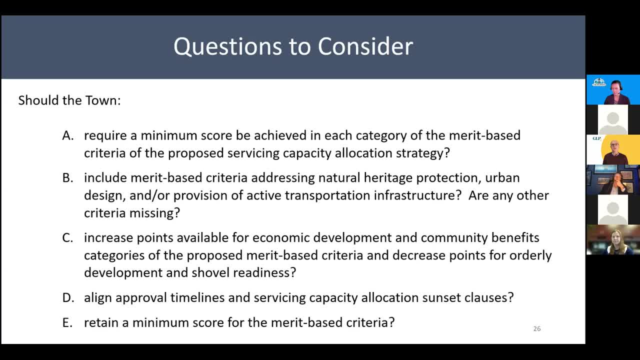 to enable you to unmute And, if you'd kindly do so, go ahead whenever you're ready. And, Shelley Kaufman, you are on decks just so you can prepare. But, Chris, go ahead when you are ready. Chris, we are seeing that you are still muted. 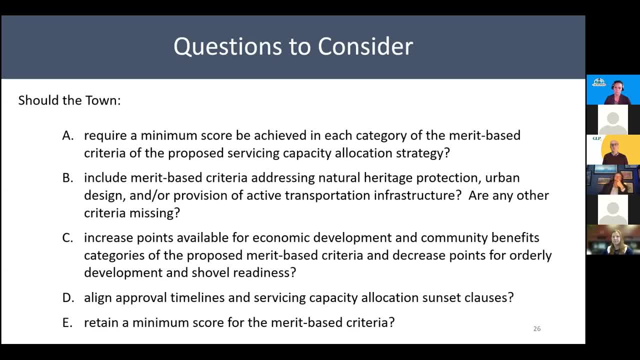 You will need to unmute on your end. Sorry, got it Good afternoon, Good afternoon, Thank you. I'll pile on on an earlier comment, then I'll provide a couple of comments, new comments. you haven't heard yet. So I strongly agree with what John Welton said. 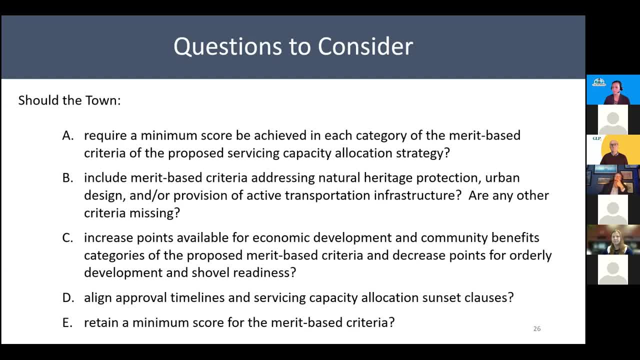 to open up the questions. The merit-based system has many pitfalls. There are a lot of items that are not applicable. There are a lot of items that we aren't even thinking of today, that you've admitted in this presentation and we may not think of by the time you do the policy. 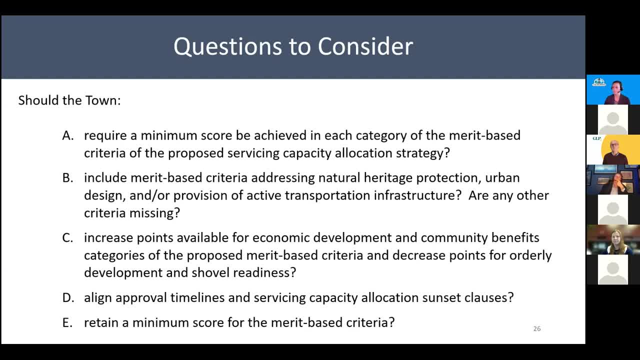 So that's a very slippery slope to go down. And some very specific comments on the program. maxing out at 100 units per phase I think is too small. I do agree with some type of a maximum If I have a thousand lot subdivision. I shouldn't hold up a thousand SDU because I can't build them all on day one. But when I have a large subdivision you need a certain critical mass for financing and to get the ball rolling with your marketing program. So probably something closer to the 200 units per phase. 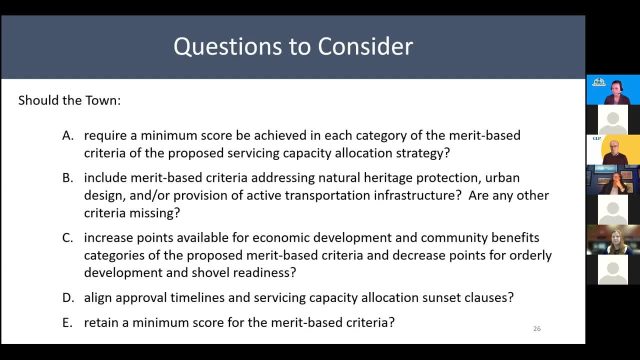 And I think that's the most important thing. And I think that's the most important thing, And I think that the most important thing is that the units that are closer to 200 and 250 units should be considered, And I really think you should use the words generally. because you don't want to box yourself in, Because if it's 200 units and I have 204 units or 210 units, you don't want to make me go back for a 10-unit subdivision And also you don't want me to go back. 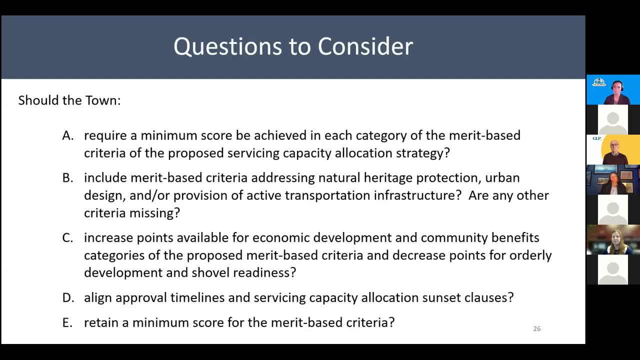 and build four houses or 10 houses in the middle of a completed community. So I think you should strongly consider that You must register within 24 months of draft plan approval. Again, I agree on timing, but that's too tight- Once your draft plan approved. it takes at least a year to do your engineering design and get your engineering approval- a minimum of a year- And then you probably again- I'm thinking larger scale subdivisions. you probably have a year of earthworks and then a year of servicing. 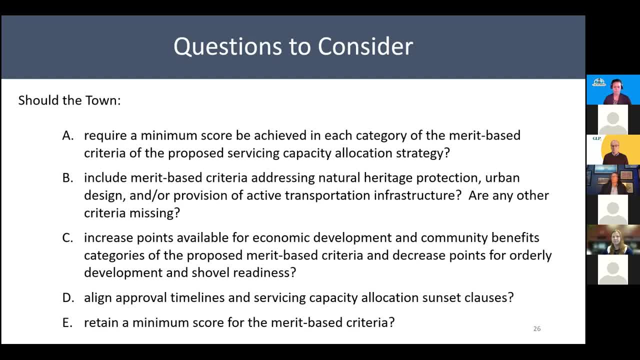 So there's three years right there. So you really need to reconsider that, because those are reconsidered And I think that's one of the realities that we face today. And my last comment would be: when you're doing your report and analyzing existing exemptions, 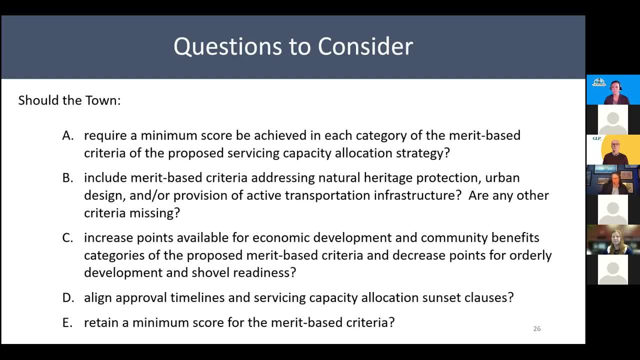 or new criteria. one thing that I did not see in there- and I believe Summit View, the one I represent, is the only one: a plan that is fully zoned, fully registered, full subdivision agreement, fully serviced and stopped mid-track. 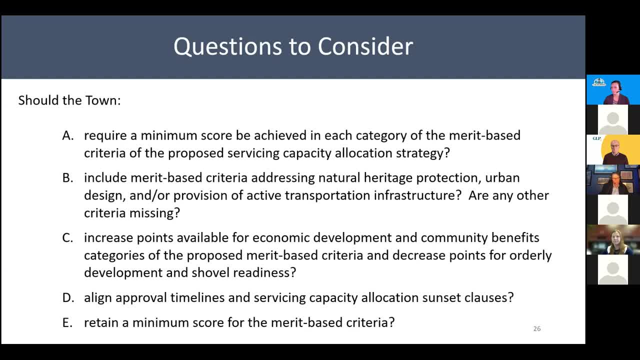 I think you have to clean up some of those issues before you get on to new criteria. So thank you very much. Thank you, Chris, for the comments. Nick Summer, any response to the idea of raising it to 250 units? 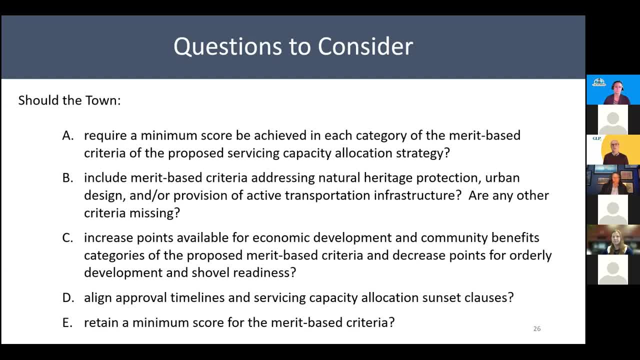 the comments on the registration timelines and so forth. Not at this point We're not going to react on the fly, but those are good suggestions and we'll certainly take all suggestions into account as we update it. But thanks for those, Okay. 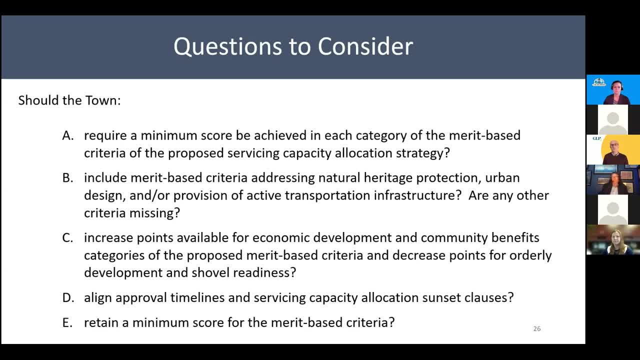 So I know we're at 425.. If I can beg the indulgence of the group, if you're able to do so, we will extend the meeting so that we can hear from some more folks and also get to some more questions that are coming in through the written Q&A box. 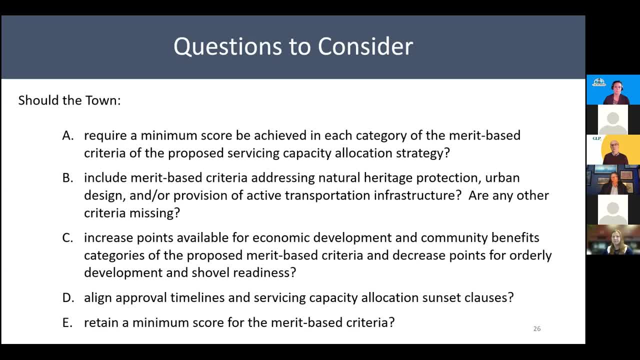 So again, if you're able to hang in there past 430, that would be terrific. But for those of you who may have to leave at that time again, remember there are other ways to share your questions and comments and observations post-meeting. 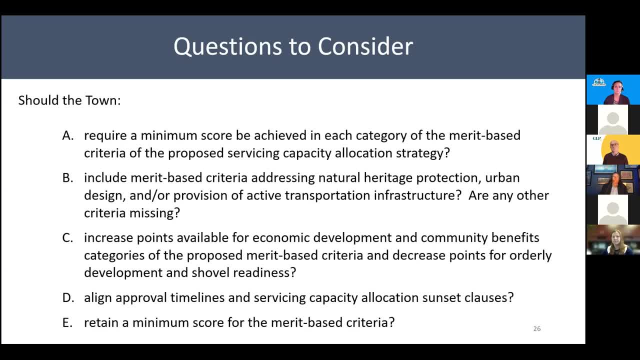 But I said Shelley Cox, Ms Rothman was next, So we will go to Shelley now. Our technical manager will invite you to unmute and go ahead, Shelley, whenever you're ready. Thank you, I'm here from Turkstra Mazza. 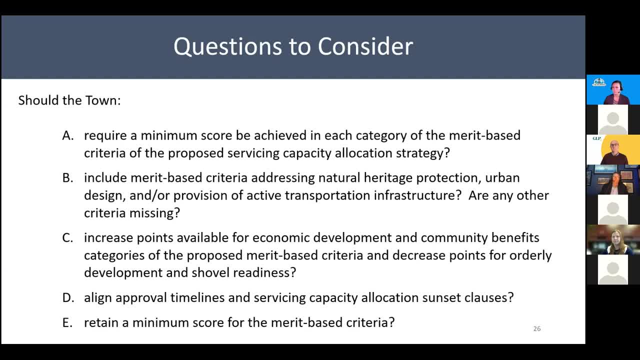 on behalf of a couple of landowners, including McPherson Builders, And there's a couple of things I wanted to raise, And one was about the competing proposals aspect. I know that Summer spoke a little bit to this in her presentation, but I wanted to clarify that even when there's 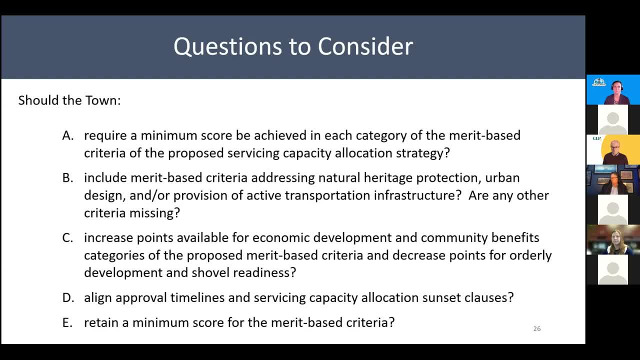 not a limited capacity that this would apply, and I guess the first comment would be that I think there needs to be some clarification as to what that criteria would be, because if there's capacity, it should be clear why this would be an allocation policy would be applied. 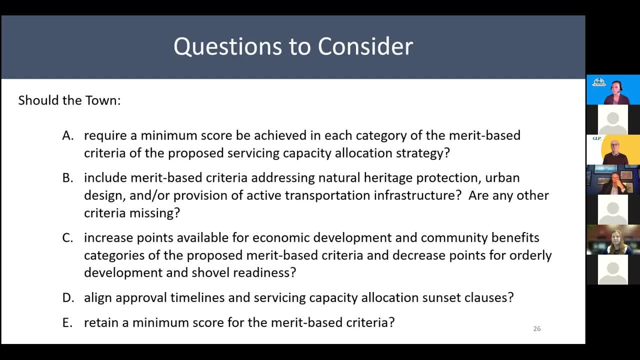 And then even within the competing proposals, what that means. So like, is this just luck of the draw that you have a competing proposal, or would it be kind of time-based? A couple of times a year you'll assess the applications. 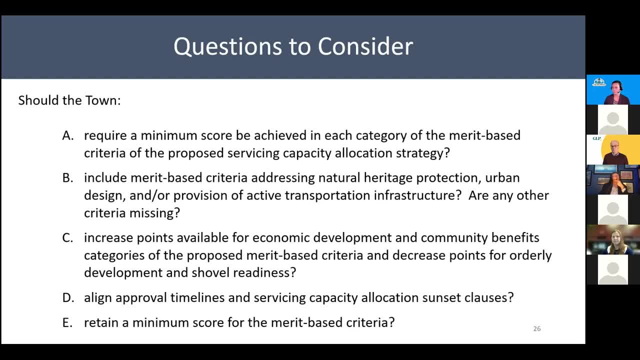 And the additional item is because the town's saying they're going to go through existing approval and look if they're competing. It's just there's a lot of questions about what that all means and how it applies. So I don't know if you can speak to some of that right now. 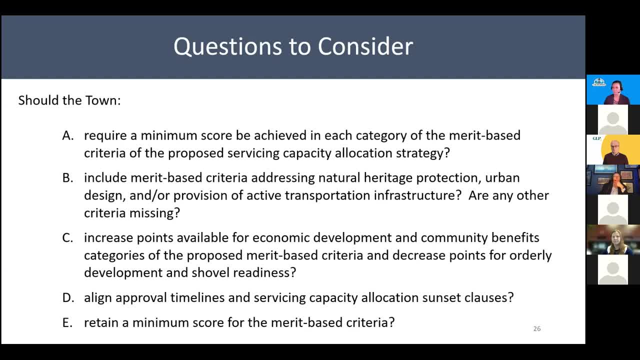 but that is one of the issues that I would raise. Okay, Well, thank you, Shelley. So yeah, let me invite Nick and or Summer. Can you provide a little more process clarity to address some of the points that Shelley has made? 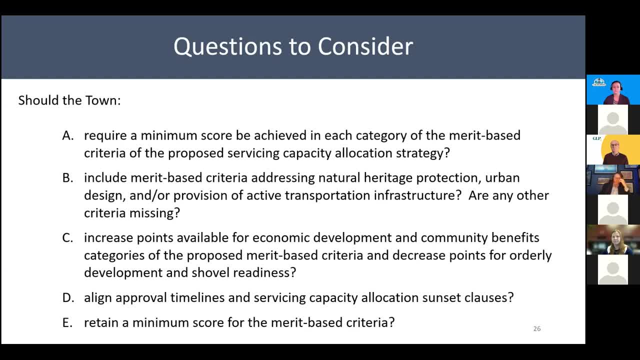 Nick, go ahead, please. I think I'll ask Summer to respond to that one. Thank you, As mentioned before, the competing proposals piece is in there only for the circumstance in the future where there's additional capacity available and the plant has been expanded. 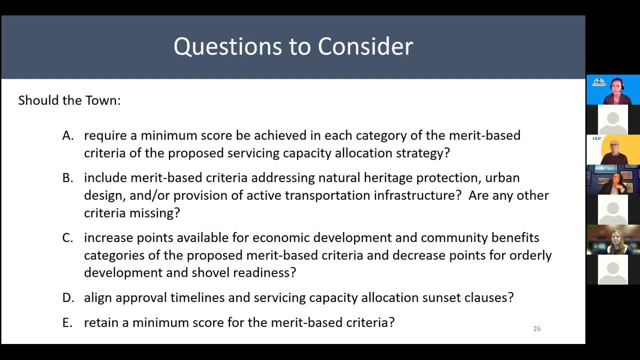 We wanted to cover off any unforeseen circumstances that somewhere in the system- and my example was sort of past- an existing pumping station which may have a capacity limitation, that's separate from the plant, And two proposals that rely on that pumping station were moving forward and competing. 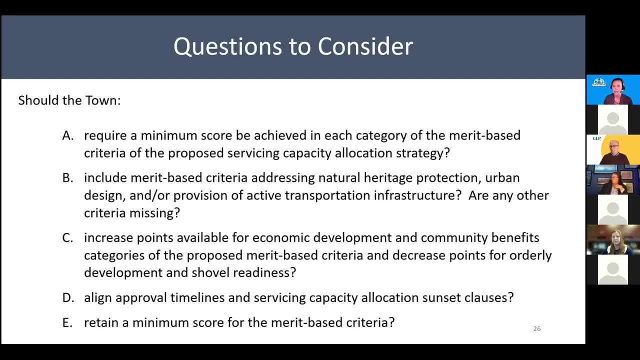 at the same time for that capacity. We wanted to have a way to trigger the merit-based criteria in those cases. So the competing proposals piece would only come into play after the plant has been upgraded. So hopefully that does provide some clarity. but we can look at the language as well. 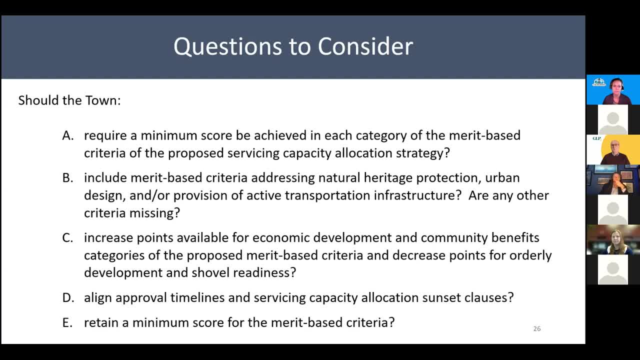 to ensure that the policy is reflective of that. Thanks, Summer, And thank you as well to Shelley for sharing those questions. So next up is Corey Chisholm. Corey, I'll invite you to unmute and speak. Our technical manager will make that option available for you. 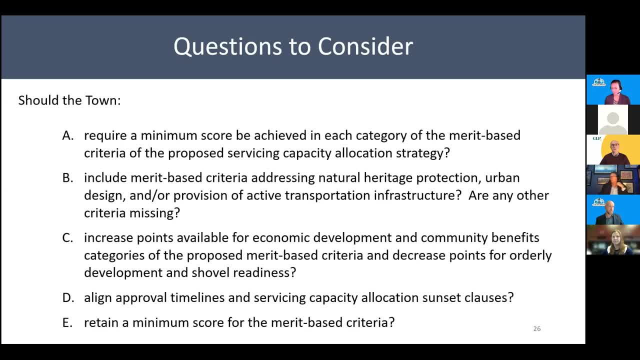 And on deck is Greg Jones. So, Greg, you can get ready. But in between Corey and Greg, I am going to go back to Nathan and we'll take a few questions that have come in through the written Q&A. But, Corey, you're up right now. 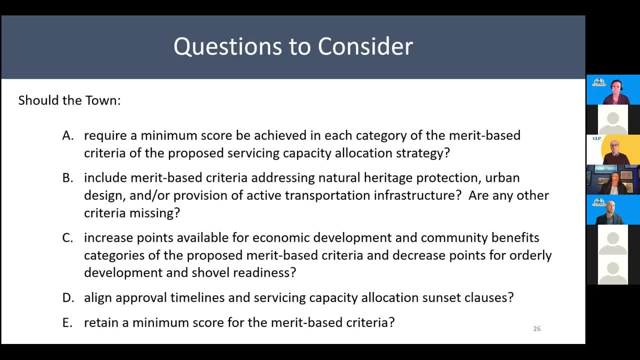 Go ahead, please. Thanks, Glenn. Can you hear me okay? Yes, I can Thank you, Corey Great. So my name's Corey Chisholm. I'm a partner with MHBC Planning in the Barrie office. 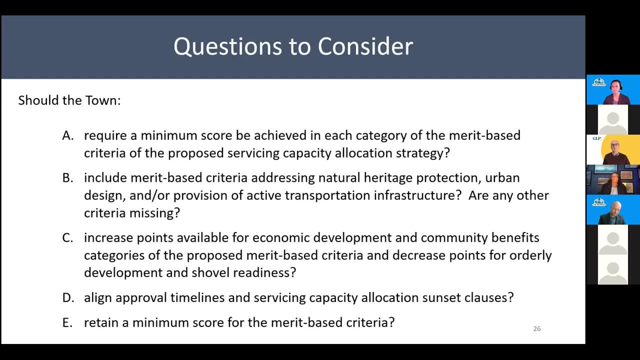 However, I'm here on behalf of the Washington Triangle Development Institute to provide comments on behalf of the development industry as a whole, And we will be submitting formal written comments that'll be a lot more detailed. However, I would like to share a couple brief comments. 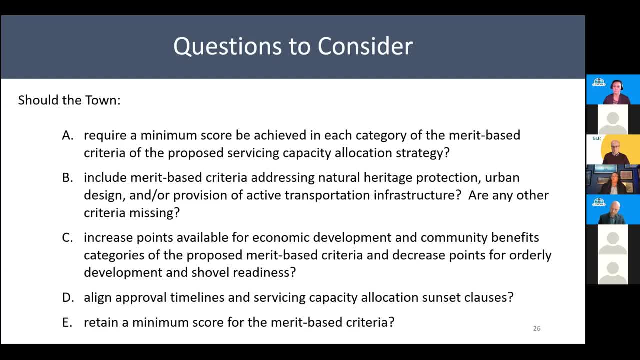 on the draft framework as it stands today, And certainly a lot of the clarification that was provided in today's presentation and discussion was helpful for framing both these comments and our future comments that we'll submit in writing. The first would just be to question 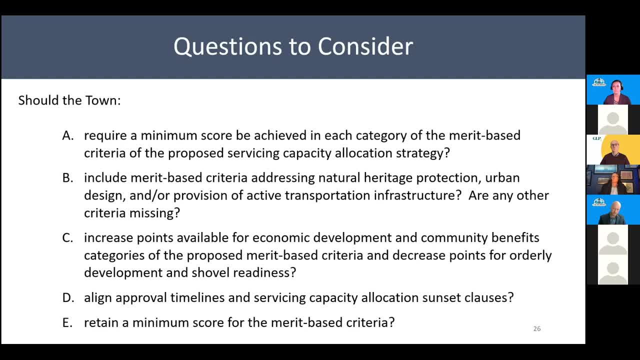 the notion of applying the merit system CARP launch, moving forward for the next four to five years until the full plant comes on. It's understood that today there's approximately 500 SDUs of capacity remaining and I believe it's expected that an additional. 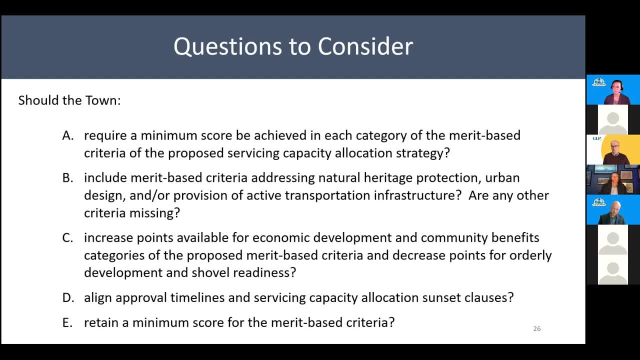 approximately 800 will be brought online in the next couple of years with the interim UV solution And just wondering if there's really the need to potentially prohibit a number of developments from proceeding within the next five years if they don't meet a minimum threshold. 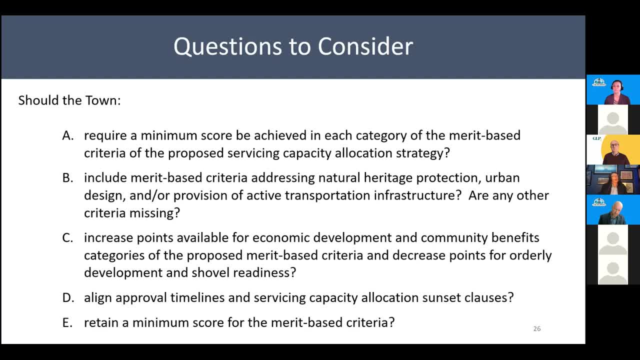 And maybe this could be retained to: really, if the town was down to a certain number of remaining capacity, if it was 100 units or 200 units left, how to then prioritize how that gets used up? So let me invite. I'll come back to you, Corey. 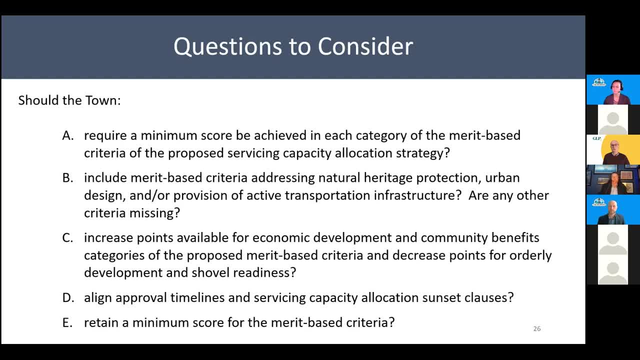 Any quick response from Summer and or Nick about what Corey has said so far? No, I think they're mainly comments that perhaps there should be a thrash, a specific SDU-based threshold where the merit-based criteria would come into effect. Okay, 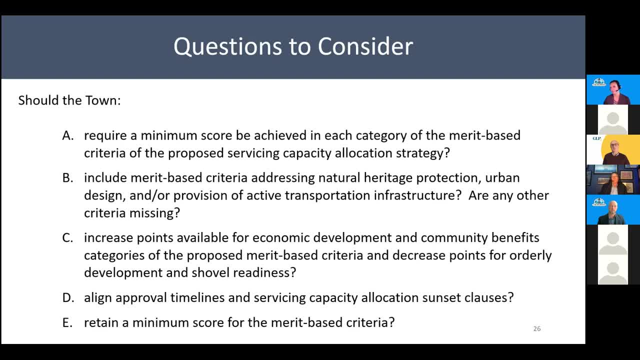 And that's something to take under consideration. Thank you, Keep going, Corey. Thanks, And just further to some of the previous comments and understand the point. system is in draft and there's a lot of moving factors at play, But through my discussions, 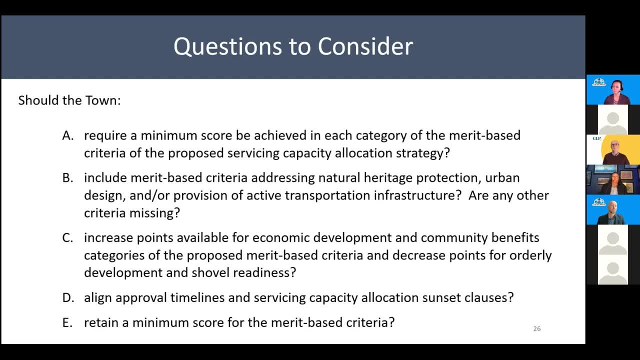 with various colleagues representing different types of developments. there are certainly concerns amongst the industry on the minimum requirement to score. I think at this point is drafted to be 75 points out of the 100.. Definitely, spoken to colleagues representing different developments that wouldn't even come close. 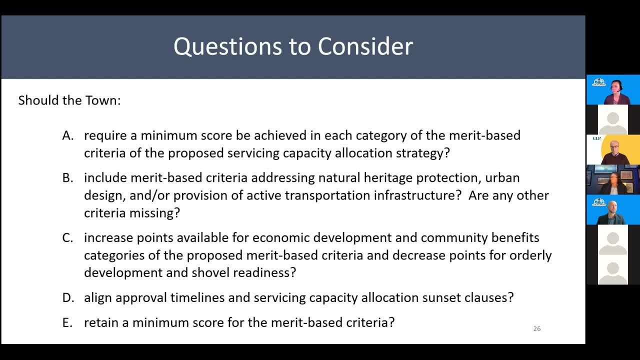 to being able to meet this as it currently stands, And a lot of that is just simply geographic in nature. A lot of greenfield developments are outside the built boundary, Don't have an opportunity to complement the main street, simply because they're not in anywhere close proximity to it. 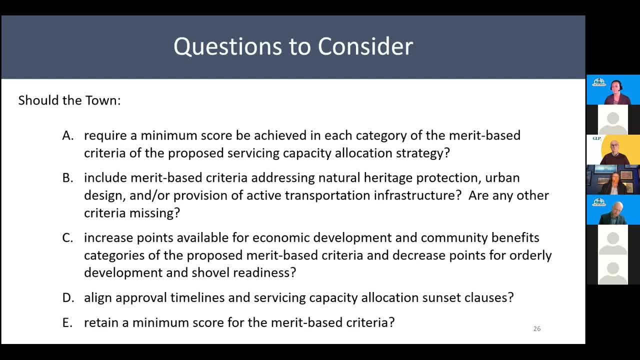 Aren't a brownfield site. If a site's a clean, you know, farm field site, it won't have the opportunity to dedicate any natural heritage lands to public. So there's a lot of these categories that simply certain sites can't qualify for due to their nature. 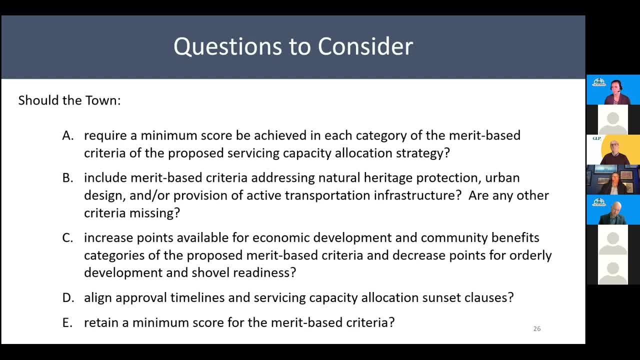 So if one suggestion would be to eliminate the minimum requirement, or certainly reduce it, or potentially you could look at a system where it's based on a percentage and if based on geographic nature- if you can't meet certain ones, then you're no longer tested against them. 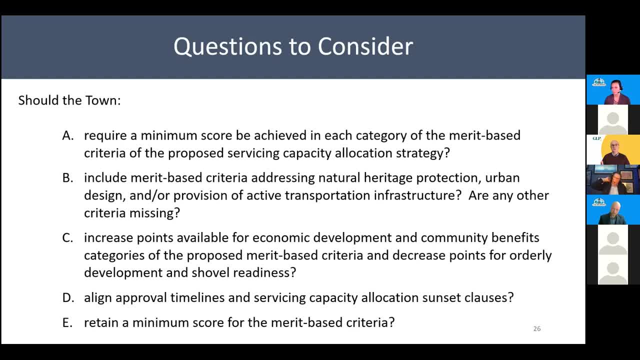 Thanks, Corey. Yeah, Nick, I know you were interested in hearing people's thoughts about the minimum and the points allocation. Go ahead, jump in. Yeah, I was just going to say very quickly, Corey, the whole point of the merit-based system. 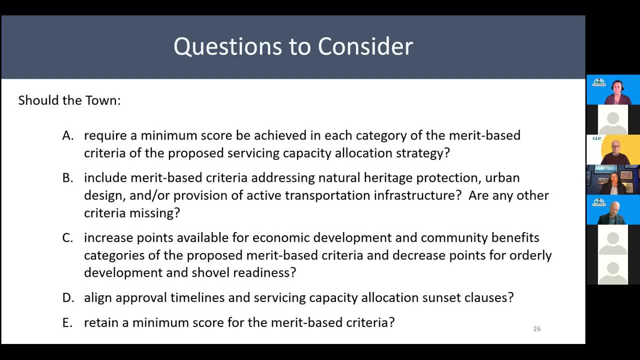 is to encourage development in the right places to occur. So there is a preference in the system for development within the built boundary and that's not unique to Collingwood. Other municipalities have done similar things in terms of how they dealt with their servicing. So there should be some benefit that someone gets for developing in places where the town wants development to occur, and that's what we're trying to get at. But we also get your point that to some extent greenfield development may be unduly affected. 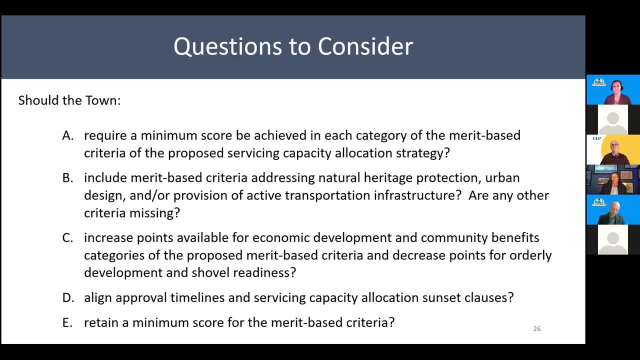 by not being able to achieve those higher scores because they're not in the built boundary, But maybe in the end that's what the town should be doing right. So that's part of the conversation we're having right now, and your comments are certainly well taken. 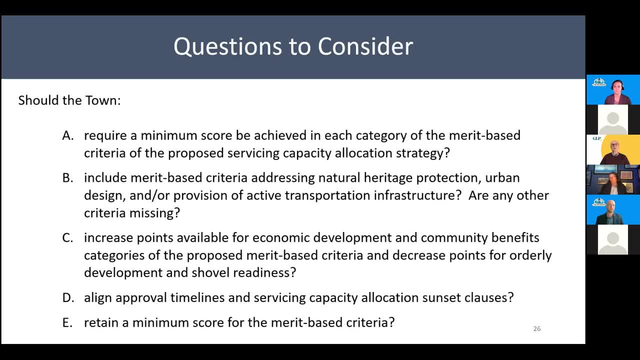 Okay, thank you, Nick. So everybody, just to take stock, we're at about 4.30, a couple of minutes past. We have three folks who have their hands raised electronically. I'm going to get all three of them in. 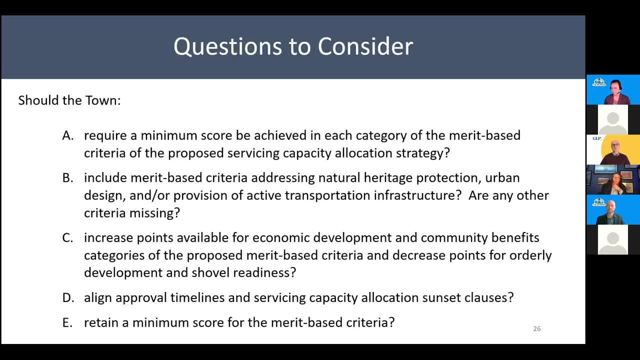 That's Greg Jones, Kenneth Hale and Vince Cicucci, if I'm pronouncing that correctly. Apologies if I'm not. We'll also take a few questions through Nathan, on behalf of those who have submitted them in writing. So we'll take those three. 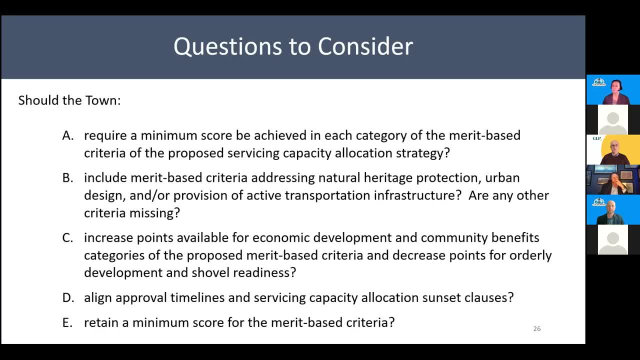 who have their hands raised electronically. Nobody else needs to raise their hand electronically anymore because we're only going to take those three And again we'll take some through the written Q&A. So I said we would go to Nathan. now Let's take one or two questions. 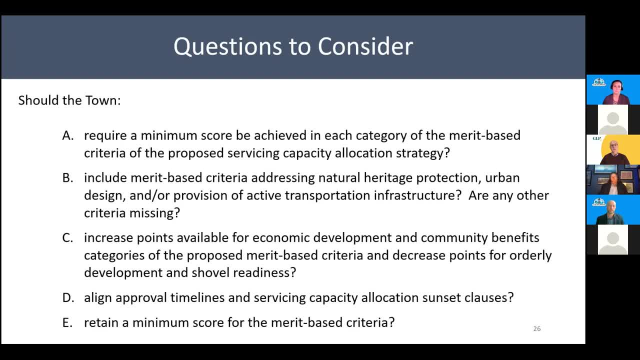 from him on behalf of those who have submitted them in writing, and then we will go to Greg Jones. after that, Nathan, what are you seeing? Thank you, Glen. Just wanted to thank everybody that's given feedback to the questions that we've posed. 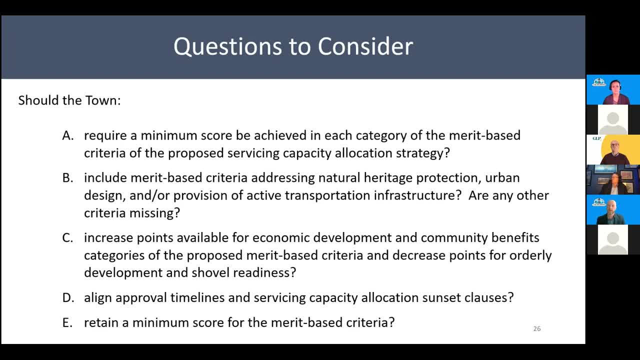 We've got a lot of answers here and we appreciate that. The next question is from Michelle Cutts, and the first thing is she notes the exemption for two additional residential units on a lot that has an existing residence. So that's a lot of residential use on it. 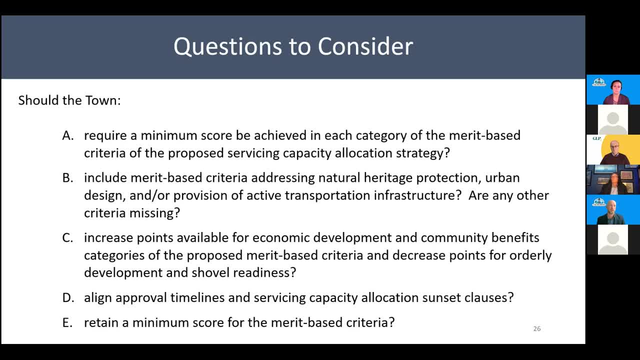 And her question is: does this also apply for the addition of a residential unit on a lot that is the site of an existing commercial use? Nick, go ahead. I think a quick answer would be: we hadn't considered it. to be frank about it. 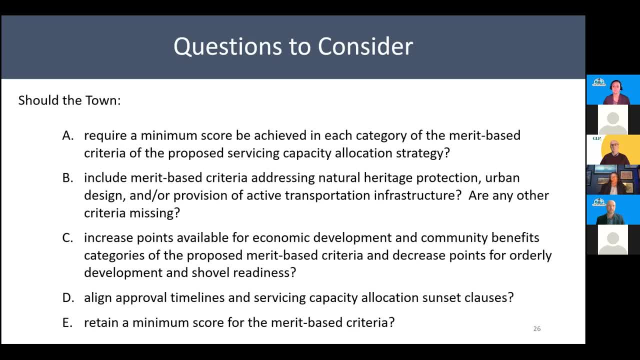 So that is something we could look at. I mean, there are benefits that accrue wherever a residential unit is added, So that's something to think about. Okay, And Nathan, what was the second question? Thank you, Nick. The next question is from David Finbow. 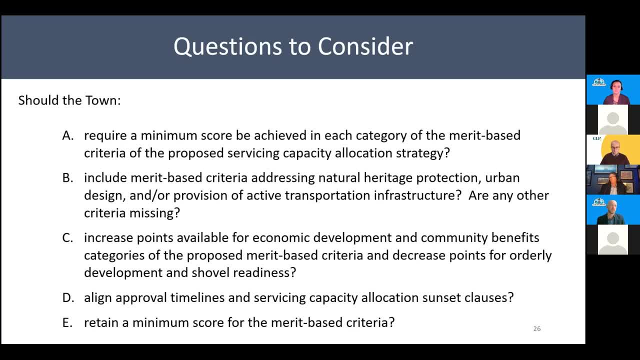 and his question is: has consideration been given to include a mixed-use column in the scorecard? Up until this point, no, But we have been thinking about how to deal with mixed uses because that is becoming more common and popular, So it's something we will look at. 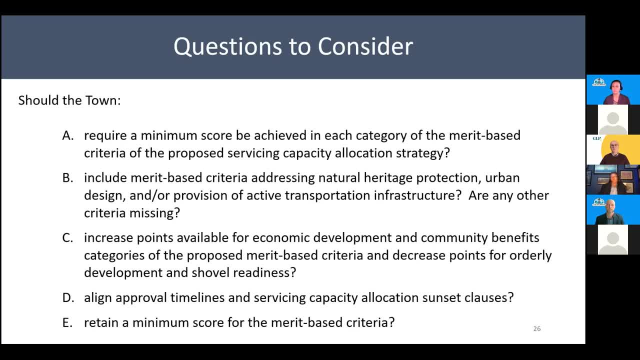 Okay, I'll come back to you at the end for one or two more, but let me go to the three folks who've had their hands up for quite a while now. Thank you, Nathan, for sharing those on behalf of the participants. 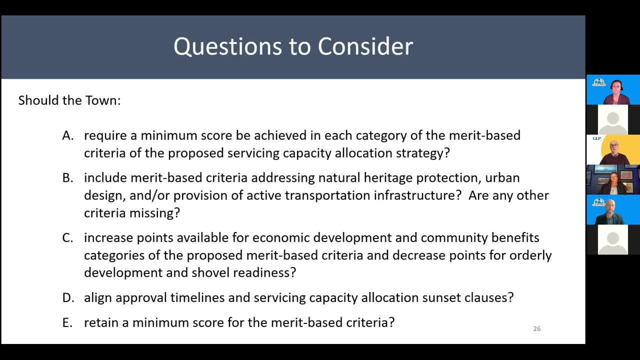 So, Greg Jones, you're up Whenever you're ready. please unmute and go ahead. Hi there, I'm Greg Jones. I'm with Skydav, part of the Skyline group of companies. We're rental housing developers, owners and managers. 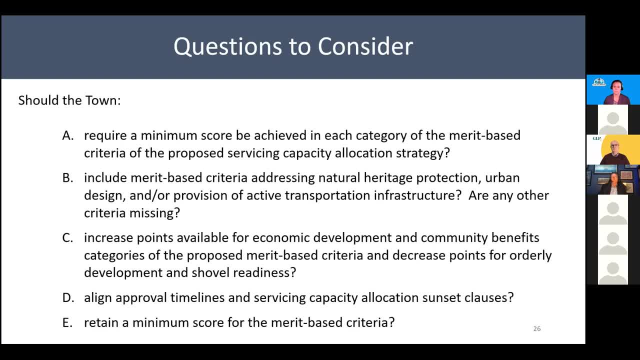 We have been on site plan for a couple of years now, trying to build new rental apartments in Collingwood. I just had a comment about the points-based system. I don't think it's fair to have criteria that are not possible. Example: you can have a clean property. 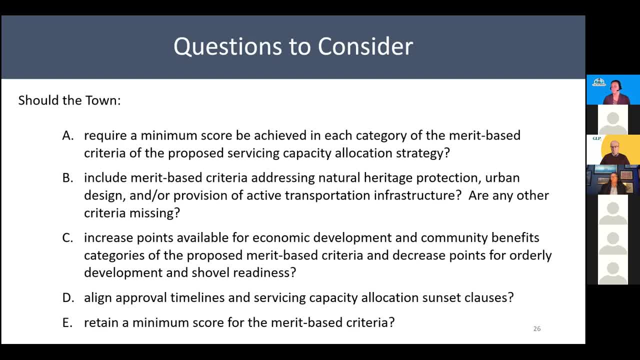 not downtown, without any kind of heritage attributes to land or heritage buildings and no land use conflicts, Automatically you do not meet the minimum points required, even if you score perfect for everything else. So there's criteria here that simply- I guess I'm just caught re-saying- 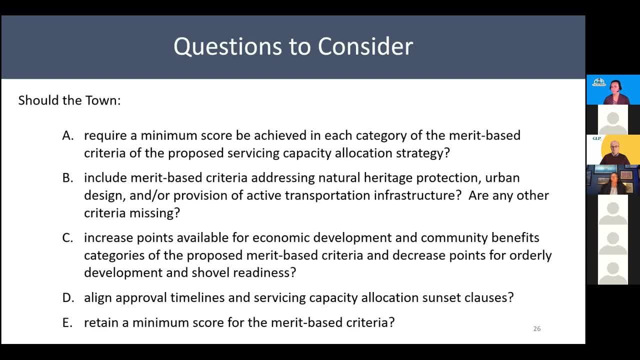 what Corey Chisholm said, but I think it should be based on criteria that developers can actually achieve. because we want to do good, We want to have those merits in our development to move forward- sustainable initiatives and water efficiency primarily- and have shovel-ready development. 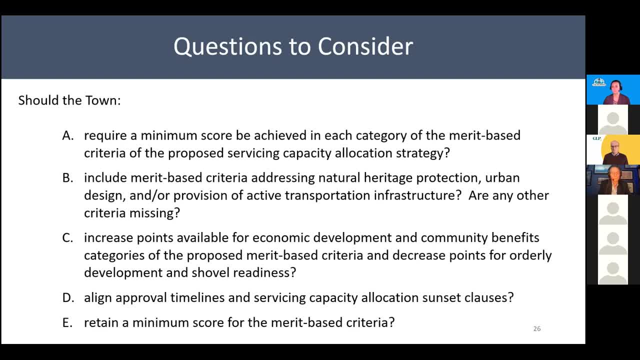 and move forward our development. I think if 75% of the available points is the target, it should be based on points that are actually available to people to achieve. That was my one and only point. Criteria should be either applicable or not applicable as part of the maximum. 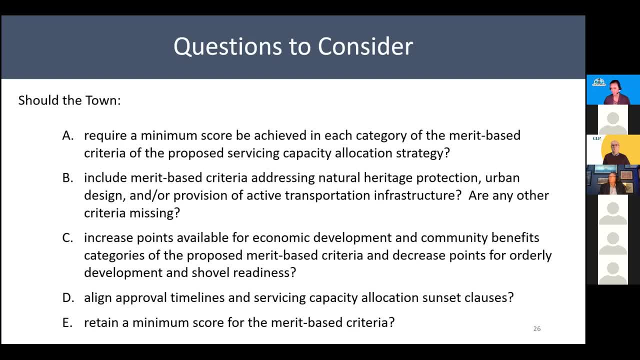 And I think it should be a percentage of that. If we're going down the road of having a points-based merit system, let developers actually give them the ability to actually sharpen their pencil and not have 25 points that are not available simply based on the location. 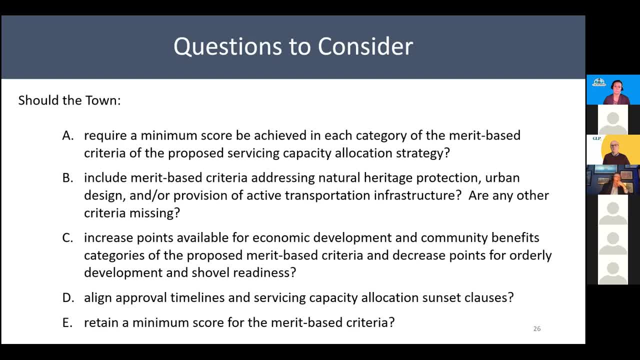 and cleanliness of a site. Okay, thank you, Greg. So, Nick and Summer- I know you're both hearing this now a number of times- There are obviously some concerns that people have about the attainability, the achievability, the practicality of the criteria. 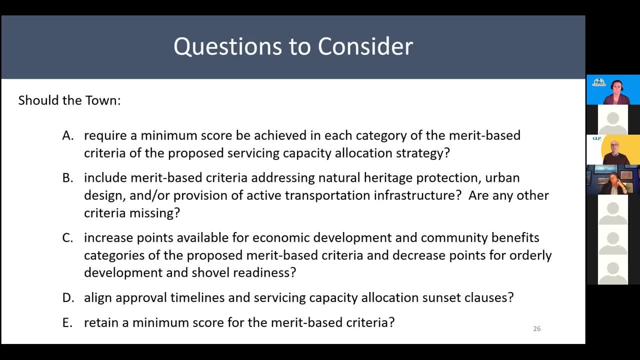 and hitting that minimum points threshold. So we won't dwell on that at the moment. but, Greg, thank you for reiterating the point. I'm going to go now to Kenneth Hale. Kenneth, we will invite you to unmute and please go ahead whenever you are ready. 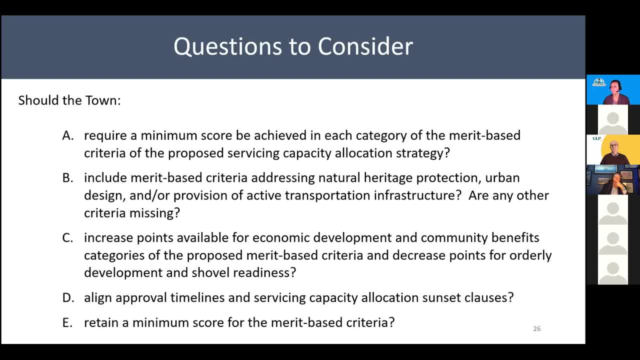 Thank you, Glenn. My name is Ken Hale. I am a developer with Dunn Capital. We own a number of properties throughout the town: industrial, commercial departments, Hotels. We have a significant amount of holdings within the town of Collingwood and have been doing business here. 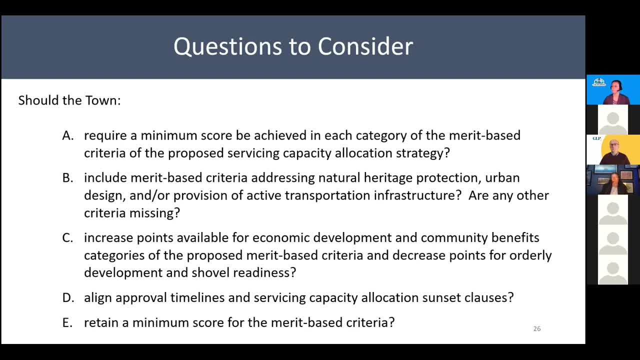 for just under 40 years. I want to say that I agree with John Walton and Greg, who was just on, and a few other developers with this point-based system, And what I would ask is: has the town in developing this point-based system? 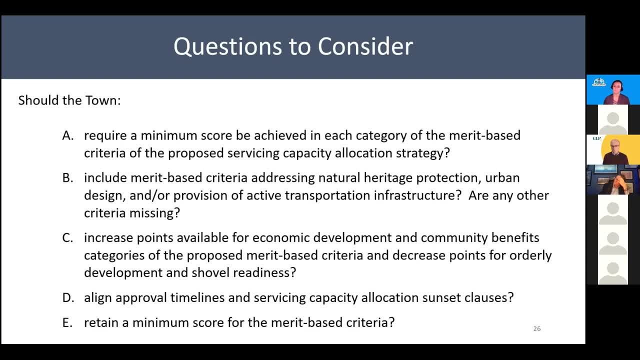 I guess my first question is- and I have a couple: has the town done an audit of the development that are on the books right now To see if any of those developments will actually achieve 75 points? Okay, So let's start with that one. 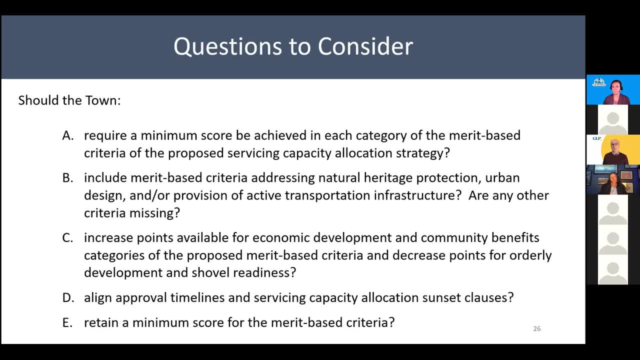 Has anyone done that kind of audit to see if current developments would achieve the point threshold? I can answer that And thank you for the question, Ken. Given the timelines associated with moving forward, we wanted to get this information out to the public as soon as possible to start to get comments. 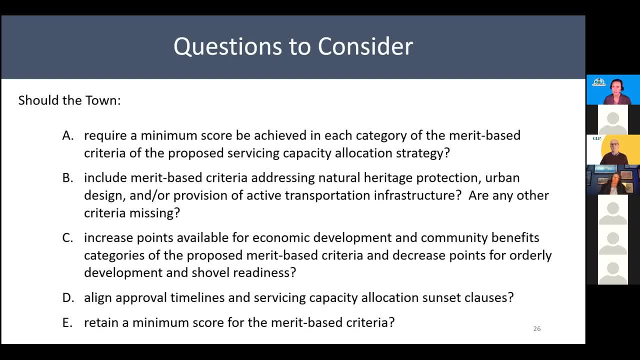 So staff are currently running through the scenarios of us- Not every development that's already on the books, but a sample of development which include commercial and industrial, residential, greenfield versus infill development and site plan and plans of subdivisions. So we're working through that exercise now. 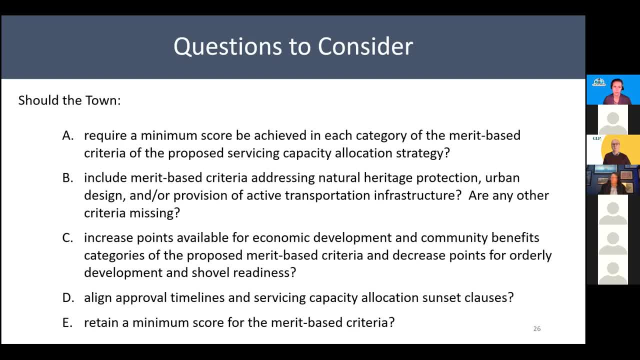 And some of the comments that we're hearing today are also some of the issues that we're running into as staff, especially for mixed use proposals. And Ken, back to you. You had a second one, I think. Yeah, I actually have a couple of points. 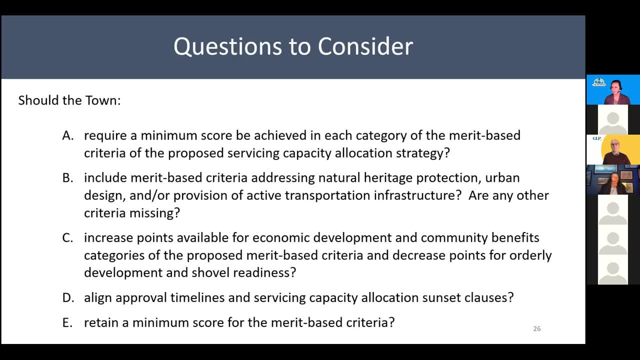 And just a couple more quick questions. And at the beginning of this Mr McDonald had indicated, and I agree, that right now water in the town is a finite resource in the short term But, as Director Slam had indicated, the plans are in 2026 to go to 58 megaliters. 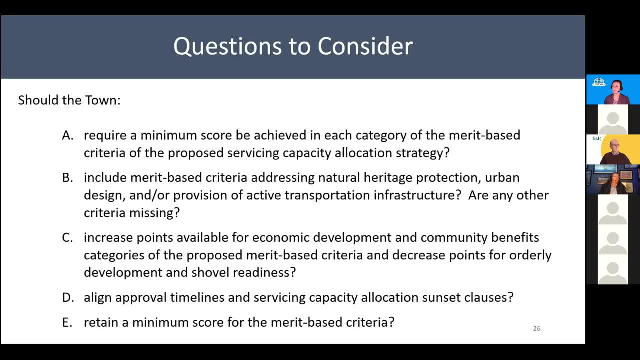 which is actually a quadrupling of what the town of Collingwood uses today, because half of our water actually goes down to new tech. So I'm just trying to understand why, after 2026, when we get to that- 58 megaliters. 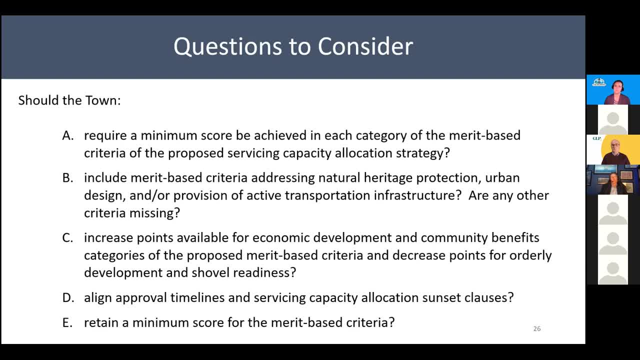 why we are still going to be looking at this merit-based system for water and wastewater. when I'm looking right now at infinite resource in the lake that we're sitting on and we are quadrupling our water intake, Why would we still need a merit-based system? 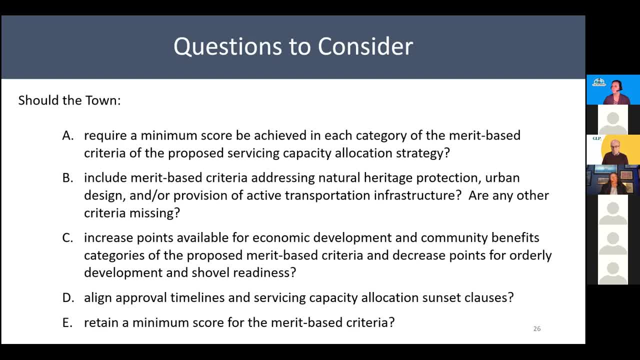 The second. the next question that I have is why is the planning policy that's being produced enshrining static numbers in terms of the amount of water SDUs are using, rather than referring to an engineer's report every year that says this is the plant capacity available? 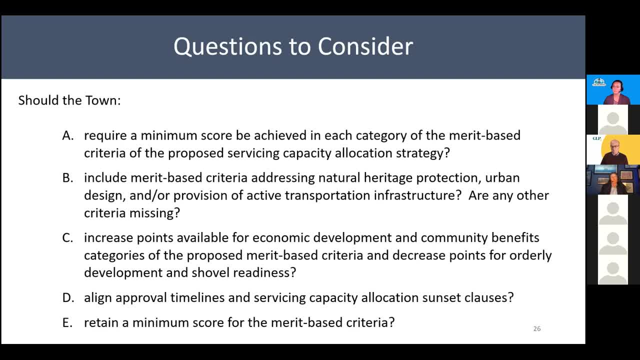 I'm unsure of any planning policy that actually enshrines engineering numbers within it and doesn't make reference to a town standard or some other report. And then my final question is: has the town looked at their statute, how they're going to meet their statutory requirements? 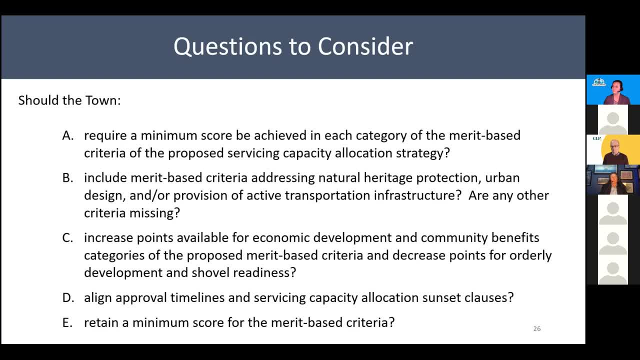 of the provincial policy statement under section 14.1, which reads- if you bear with me here a second, I'm trying not to take everybody's time here- that the planning authority shall at all times maintain, at all times new development is to occur. land with servicing capacity. 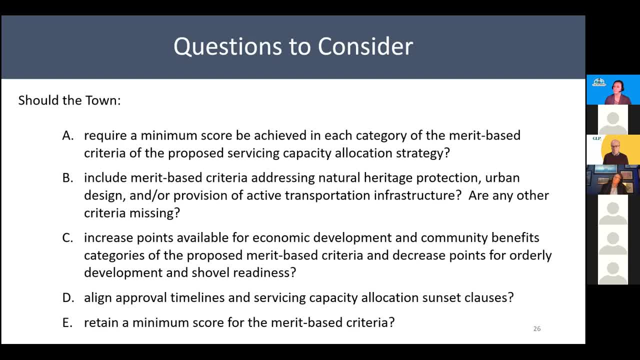 sufficient to provide at least a three-year supply of residential units available. So there are three questions there that I have Just to recap. why, after we are quadrupling our water in 2026, are we still using a merit-based system? 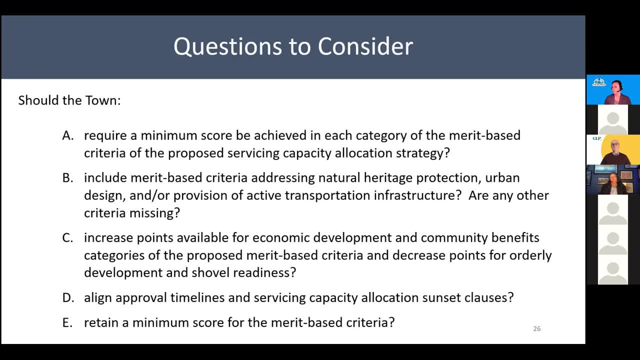 Why are we enshrining static numbers of how much SDUs are being water being by SDUs, And has the town considered how it's going to meet the provincial policy statement to having water available for its projected growth? Okay, thanks, Ken. 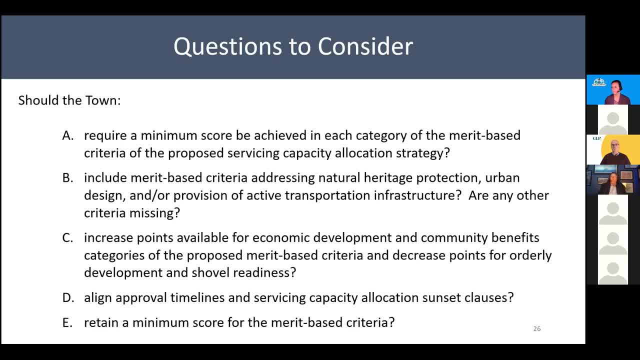 So let me ask, maybe Nick- I think is going to kick us off- Do you want to take that first question? Yes, so three quick answers. This is what we're suggesting in the end will be a council adopted and approved document. 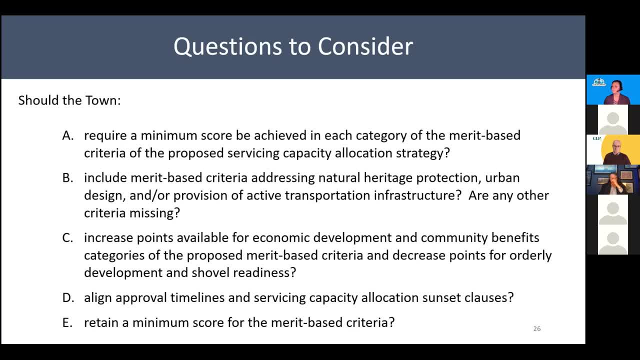 And council can certainly, at its pleasure, change that document when it sees fit, And I think the conversation about whether the merit-based approach should live or not is probably a 2025 discussion and not one for today. I'm just saying that at this point. 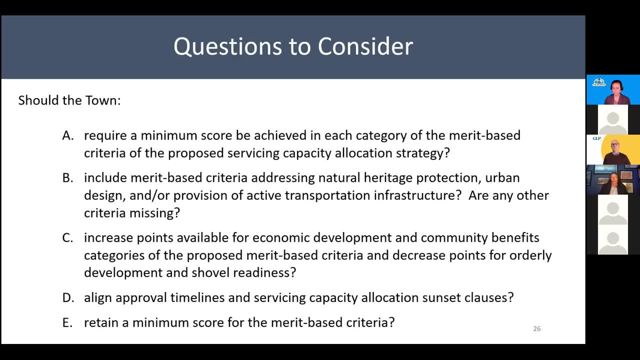 We've thought about that too Clearly. there is a finite resource right now that we're trying to deal with, So really the focus is on that. But in our review of how other municipalities do things, there is an element of merit considered even in municipalities that have tons of capacity. 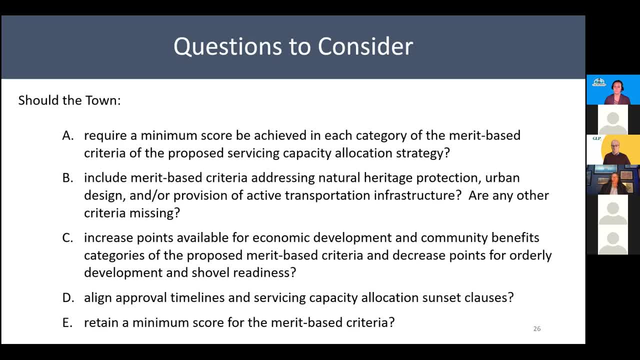 because choices still have to be made on where development should go, And those choices should be the right ones. in terms of checking off the right boxes, The merit-based system may look different in a circumstance like this, in a circumstance where there is a lot of capacity available. I agree. 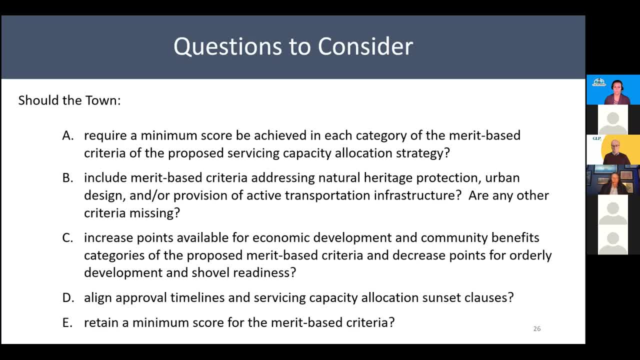 But it's pretty hard to figure that out today And I think that's probably a future thing. In terms of the SDUs, your point's well taken. I'm certainly aware every year there are recalibrations done and recalculations done on this. 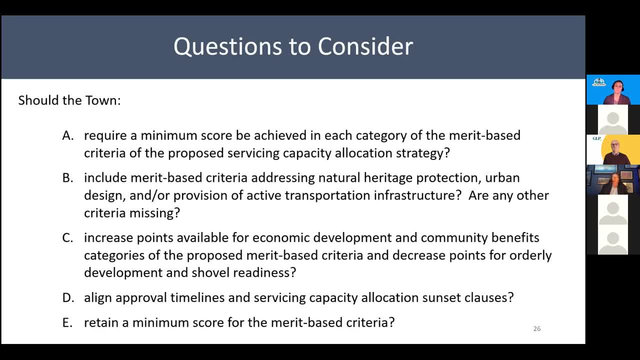 So I think there should be some recognition that that could occur in how this is all figured out. But in the end, with your last question, the town is working very hard to make sure that there is land available for development in accordance with the Provincial Policy Statement. 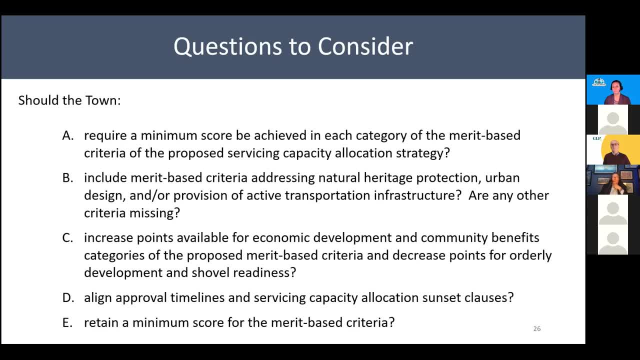 And it's going to cost a lot of money, And the town is certainly committed to going down that road and doing just that. And, Summer, did you have anything to add? Nothing further to add at this point, Glenn, Thank you. Okay, thank you. 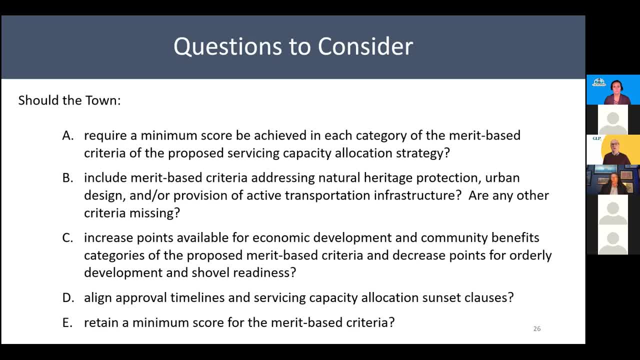 So let's go to Vince Cicucci And then, as I mentioned, we will go back to Nathan and just see if there's maybe one or two other questions or maybe, more importantly, a couple of key themes that seem to be emerging from people's responses. 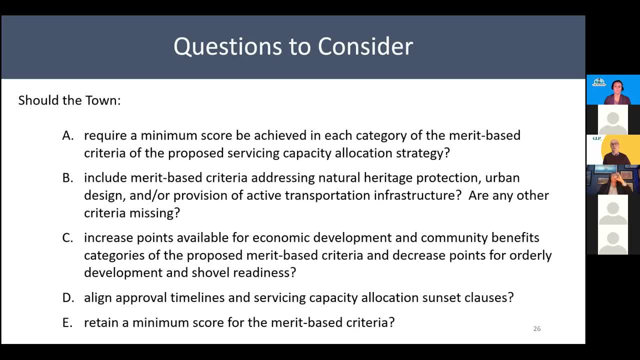 But we'll go to Nathan in a moment. But, Vince, please go ahead. I know you've waited patiently. We're happy to get you in. Thank you, Glenn, And for the record, you did pronounce the name right, So that's very good. 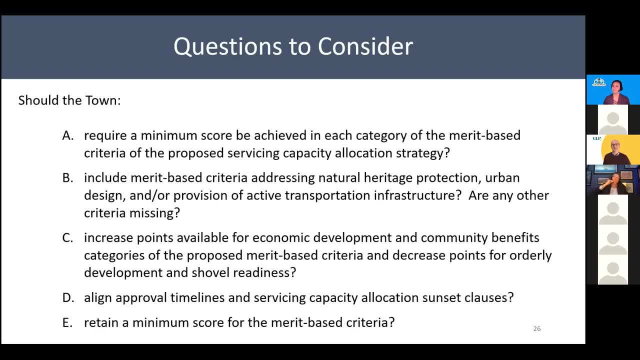 Good to hear, Thank you. I'm not a planner so I'm not sure if I'm directing this at planning And I'm with Newtac Holdings. We have several properties in Collingwood. What I'm curious about is when you, I guess as a filter, 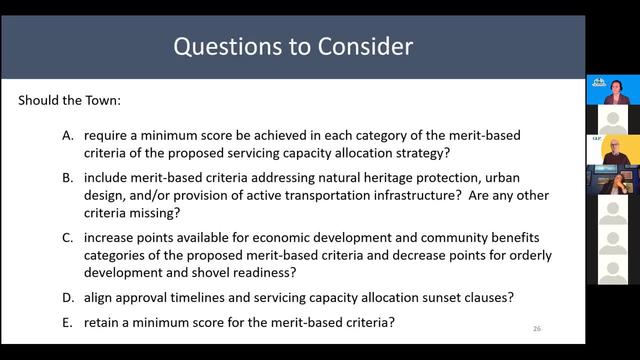 given that the criteria for seeking an exemption is really a series of filters, would it not be the sort of first filter, from a triage perspective, examining whether or not an application requires more water allocation And if a site doesn't require more water allocation? 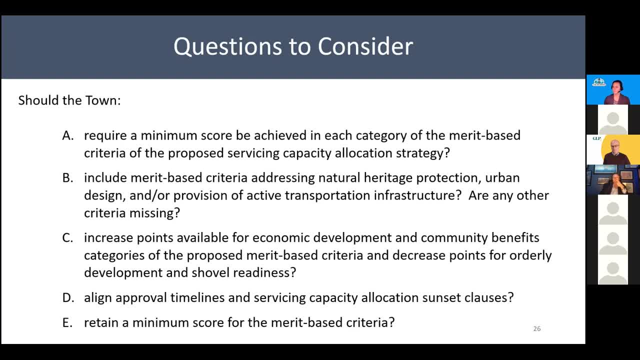 why should it seek an exemption? And how is the community or good planning compromised by that? In our specific example- because everybody obviously has a specific example- we're returning SDUs to the municipality with our proposed redevelopment, So we're giving water allocation back. 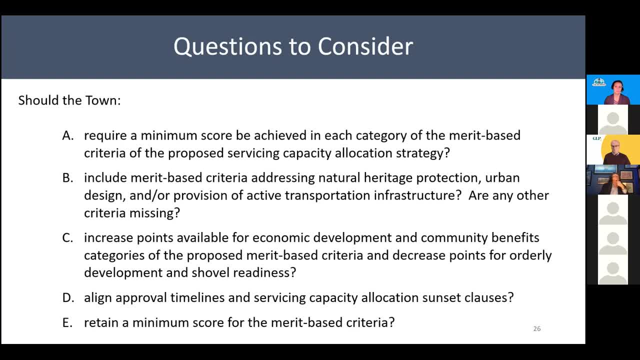 and yet we're required to seek these exemptions, which seems nonsensical. Not only does it place uncertainty for us, but it also creates a workload- an additional workload- on planning staff to have to do these kinds of reports that are unnecessary. So perhaps somebody could answer that. 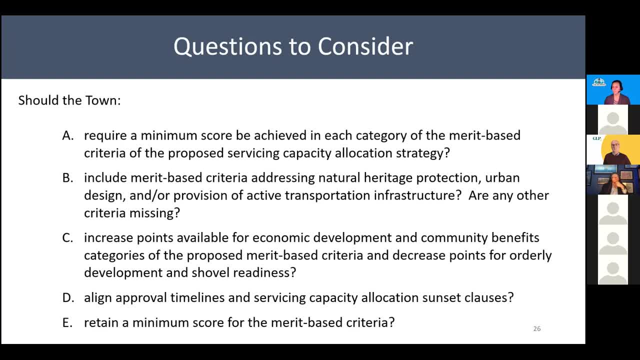 sort of first question And I have one other sort of additional question, unrelated. Okay, I'll come back to you, Vince. So, Nick, can you speak to this point about maybe using a triage filter that could be used initially and looking at cases where a development? 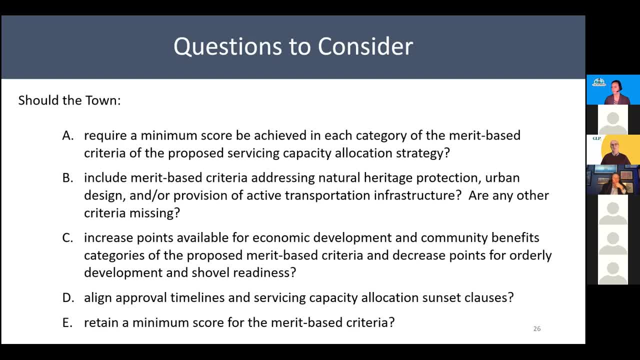 might actually be bringing units back to the town, so to speak. Go ahead, Nick. Yeah, so I guess there are two circumstances. One is which something is proposed and there is no increased servicing demand. They're automatically exempt, but somebody has to make a judgment call on that. 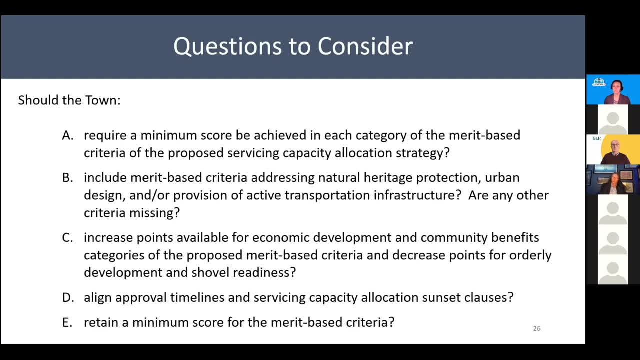 so that's something to work out through implementation. What you're suggesting, Vince in your example, is you're actually returning SDUs and putting it back in the bank, so to speak, and how does the town deal with that? That's a very good question. 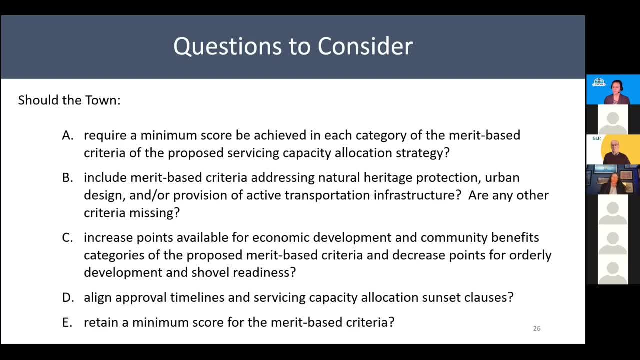 so I don't have an answer, But it's certainly interesting because certain developments may actually do that and maybe there should be some recognition for that somehow. I'm just not sure at this moment what that would look like, but it's an interesting proposition. 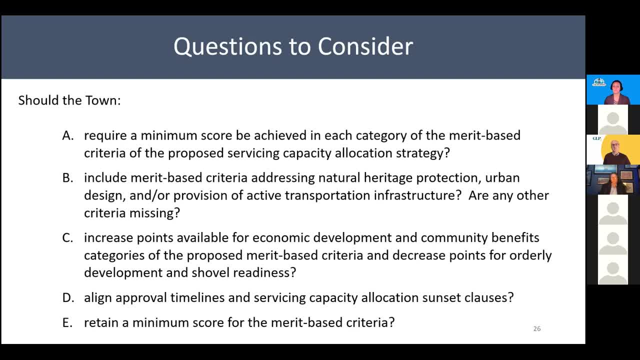 And let's go back to Vince. You said you had one other question. Go ahead, please. Yeah, I appreciate your comment, Nick, and I guess I would invite planning staff, as you bring this to Council, to consider. you know the specific example. 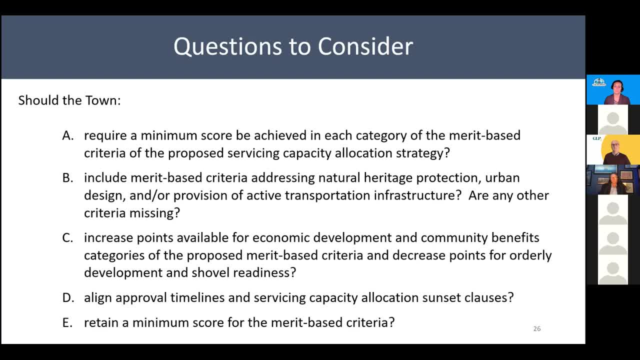 where it's demonstrable that by obviously a qualified engineer that you know, SDUs are required to return to the municipality, that they're just simply automatically exempt. You can't extend it as far as in my mind if you're not taking any more from the pie. 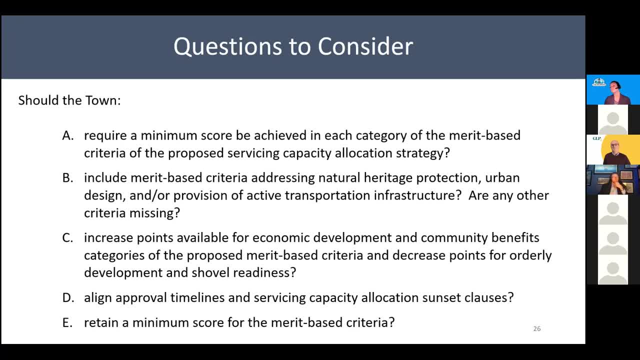 you know, why should you have to go through these hoops and then burden planning staff and create uncertainty? So I appreciate the comment. I would simply invite the planning staff to consider that in whatever they deliver to Council for consideration- The last one is unrelated. 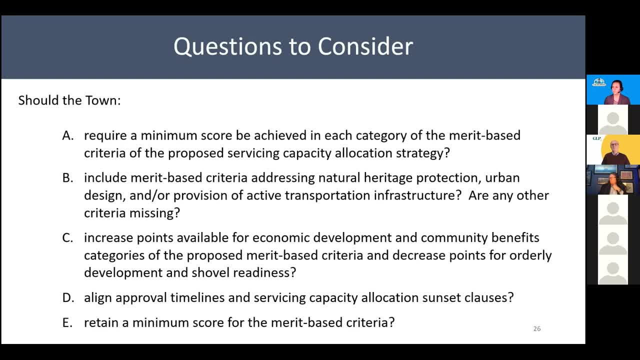 but I noticed or noted that land is placed in a holding provision And then, at the same time, there is- I think you referred to it- the notwithstanding clause that relates to the bylaw And it seems to me to be a bit of a belts. 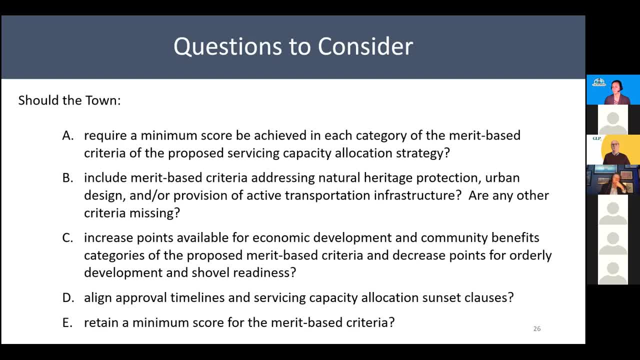 and suspenders kind of application, where you've got two elements that can actually hold it at the building permit stage, And I'm not sure why, but two hoops are required in that particular case. I can't differentiate between the two. No, that's a really good question. 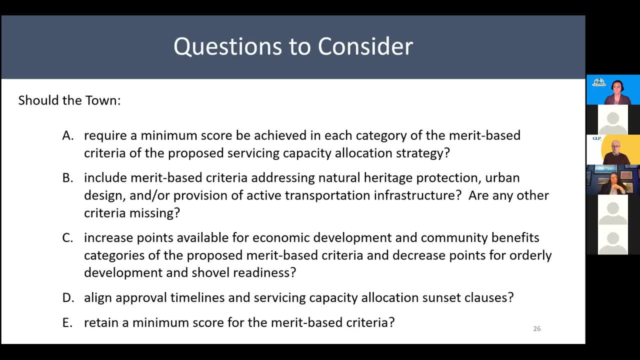 And you're right. both serve the same purpose and achieve the same objective. What we found, though, is by actually having a holding provision on a property, people are much more aware of the town, of a potential limitation to development on their property. 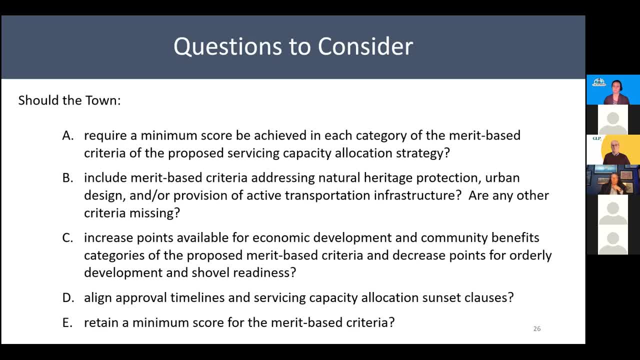 than they would be if they were looking through a bylaw. They're trying to figure it out on their own. So there's pros and cons, but there is an element of belts and suspenders here for sure. The town is trying to come up with a plan for moving forward. 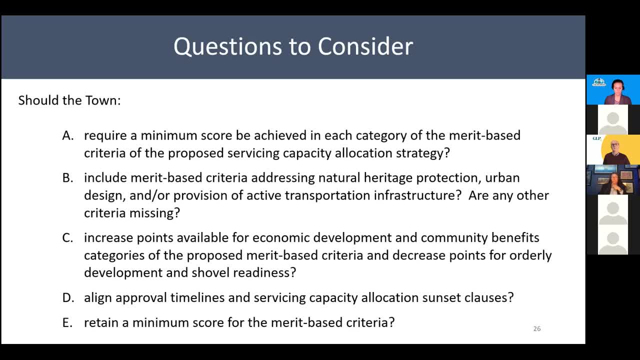 that covers them off and protects the overall public interest. So your point's well taken. Where the holding provision gets used is a discussion item. It's pretty typical. when subdivisions are draft approved and there are limitations on how much development can occur, It's pretty typical. 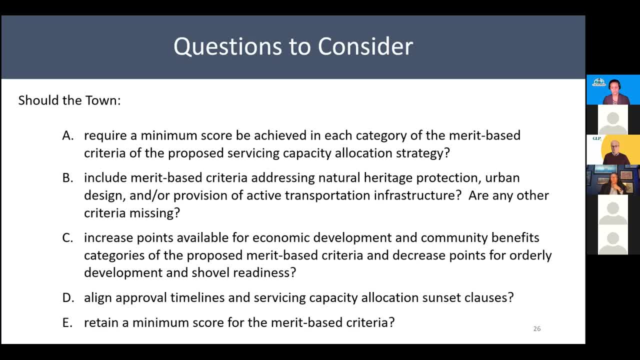 I wouldn't see holding provisions used across the town. I think it would really be only in those cases where developments are proceeding through some type of process, where some kind of phasing is required and things need to happen before you can go from one phase to another. 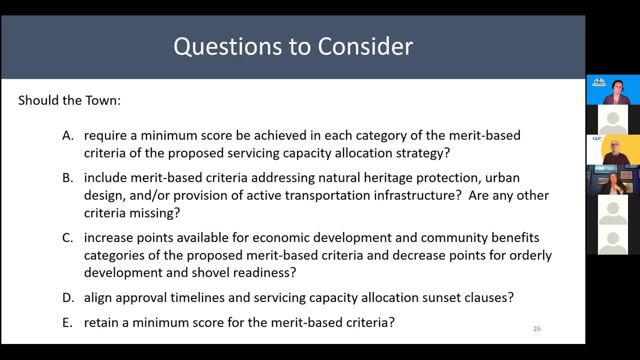 Having said that, we've seen circumstances where the entirety of an urban area is the subject of a holding provision because of servicing concerns. I don't think I'd recommend that, but I've seen that happen too Well, I just want to say thank you to Vince. 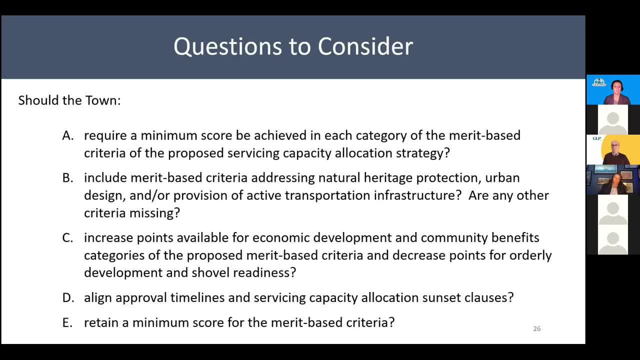 and really to all of the participants who shared questions and comments. We appreciate you sharing your views, your wisdom, your insight, your perspectives Just before Summer reiterates next steps and where things go from here. I promised we would go back to Nathan. 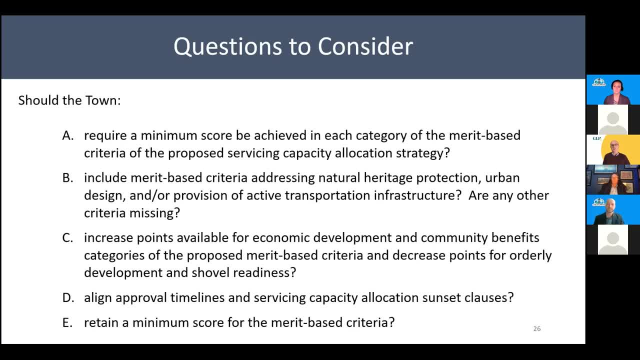 And Nathan. maybe we don't do any other questions at this point, but are you seeing sort of one or two big messages coming through the myriad of responses you've been getting to the town's questions? It sounds like we're hearing quite a bit about the point system. 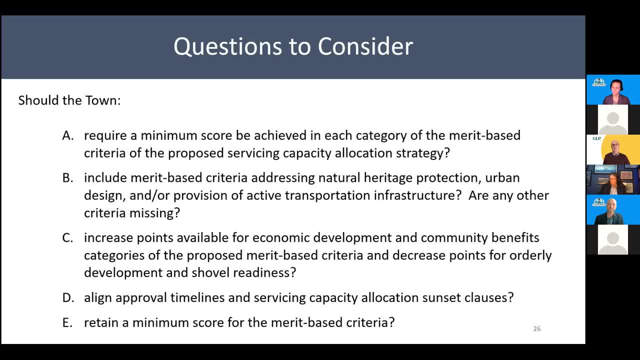 and whether it's attainable. But go ahead, Nathan. What are you seeing, at least as a preliminary look at the data? Yeah, thank you, Glenn. We've actually answered all of the questions we've received. So just to summarize some of the feedback that we've seen already through the Q&A forum: 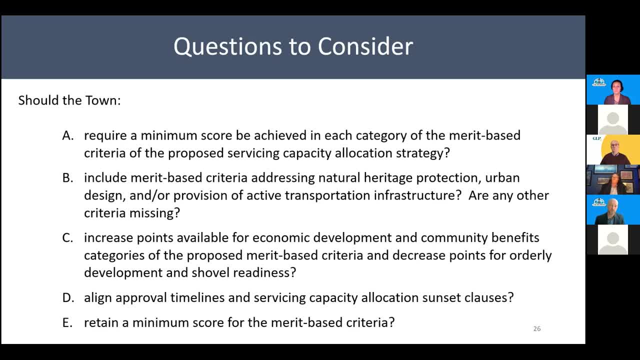 is that, yeah, it is difficult to meet the 75 points. We've had a few respondents, Yeah, We've had a few comments on that And there's a general feeling that I'm seeing here that no minimum scores should be applied as well for each category. 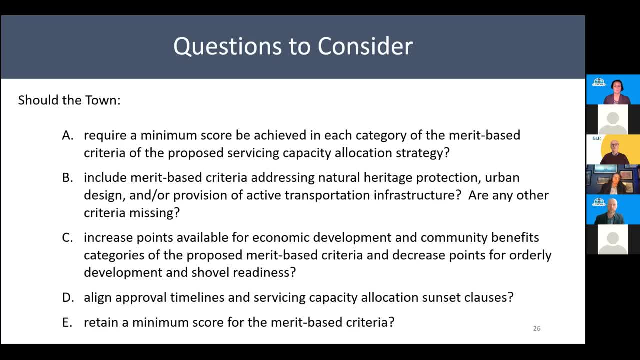 or for the whole project. And then there was one other theme that arose about job creation, and that was that the job creation category should be used for just the commercial, industrial and not residential, and really focus on permanent jobs rather than construction jobs. Okay, 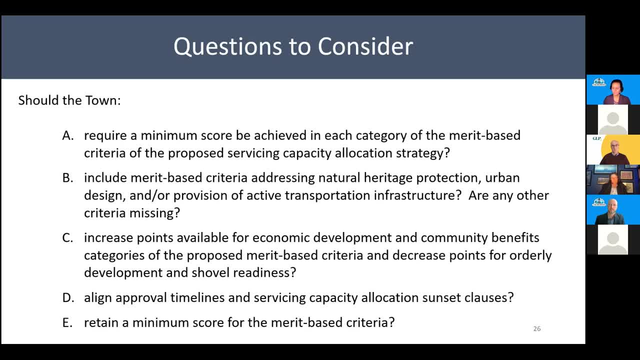 Thanks, Nathan, Appreciate that quick overview And I know there'll be much more. you know more rich findings as you sift through the comments in greater detail. So thank you everybody for giving us an extra 20 minutes. We'll wrap this up in the next three or four minutes. 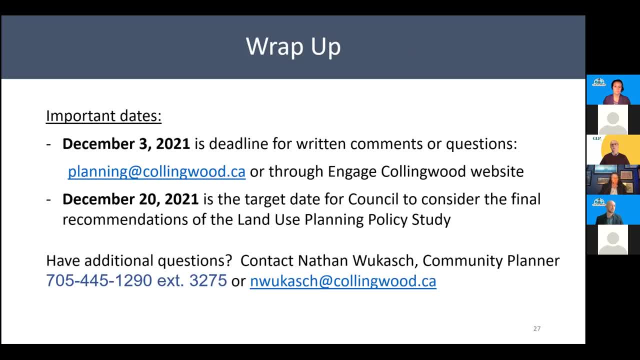 Just before I formally draw things to a close, I wanted to invite Summer Valentine again, the Town's Director of Planning, Building and Economic Development, to talk a little bit about next steps and share any summative observations she might have, And then I'll formally draw things to a close really quickly thereafter. 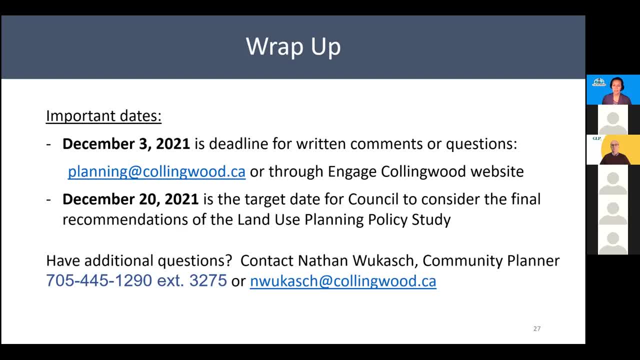 Summer go ahead, please. Thank you, Glen, And given the hour, I'll just focus on highlighting for the group some of the important dates. So we've got a written commenting period open for 10 days, until December 3rd. 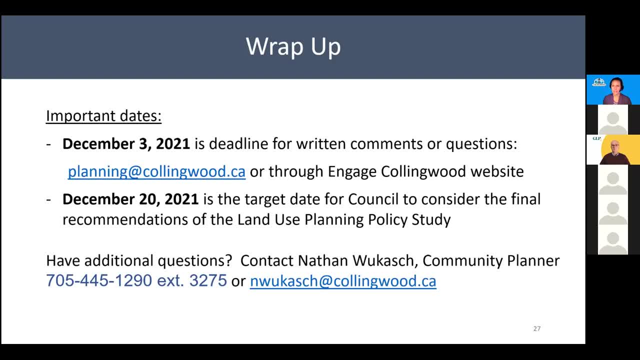 And you can do that either through planning at collingwoodca, by email or through the Engage Collingwood website. And another important date to remember is the target date to have the package returned back to Council for a final decision on the recommendations of the Land Use Planning Policy Study. 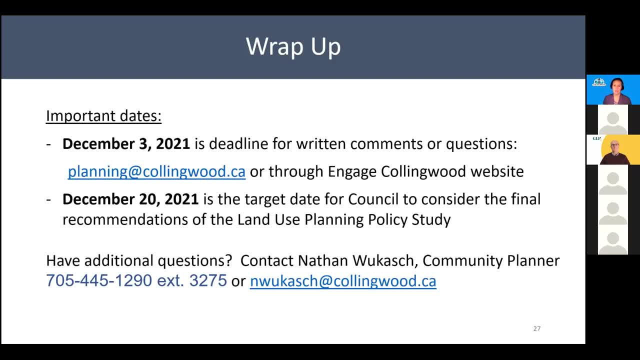 is currently December 20th. There might be some flexibility in that date depending how much feedback we receive and how much additional work there is to do to bring forward a product that we all feel comfortable recommending. And we do recognize that we might not have gotten to everyone. 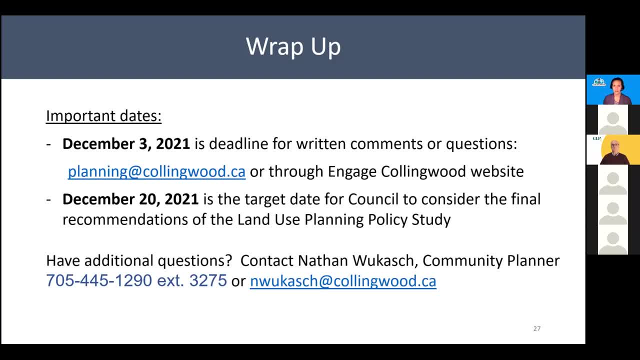 or people don't feel comfortable participating in this format or have site-specific questions. So if you do have additional questions, please do reach out to Community Planner Wukash, who is here with us today. His number and contact information is available on the slide. 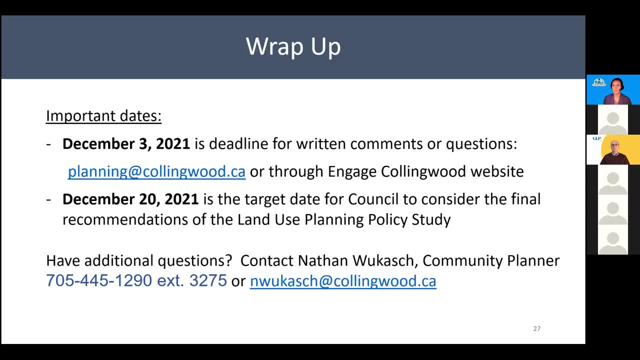 And I have confirmed as well with our communications group that this slide deck will be available on the Engage Collingwood website And therefore you'll be able to access this contact information easily through that platform as well. Just to add to add to what Glenn mentioned. 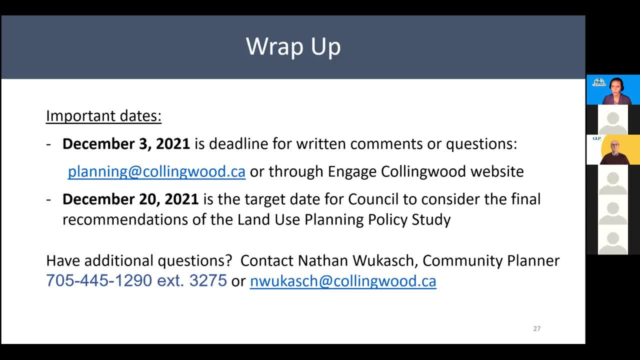 we are incredibly grateful that everyone was able to join us here today and share the comments and questions that they have, And we look forward to any further written correspondence or conversations that we may have on this topic. Thank you, Great Thanks, Summer. 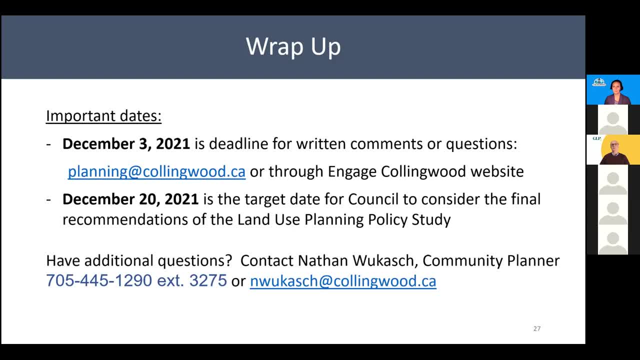 So just give me 30 seconds everybody. I want to thank you all again for participating. A special thank you to those who shared responses and comments and questions. I know this project invites you and invites a lot of interest and passion, And thank you for the very respectful dialogue. 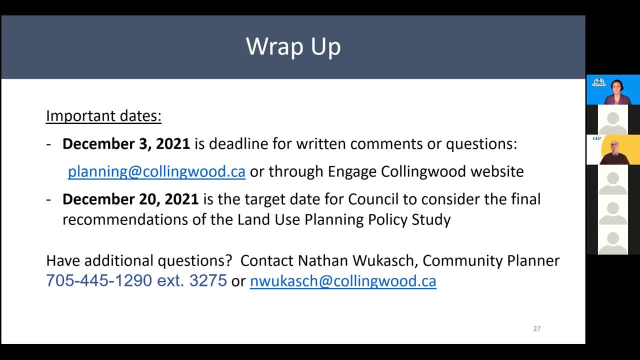 And thank you again for the insightful questions. I think you've given the town a lot to think about. I'd also like to thank any of our elected officials who joined us this afternoon, not only for their interest in this topic, but also for their ongoing valued contribution to the community. 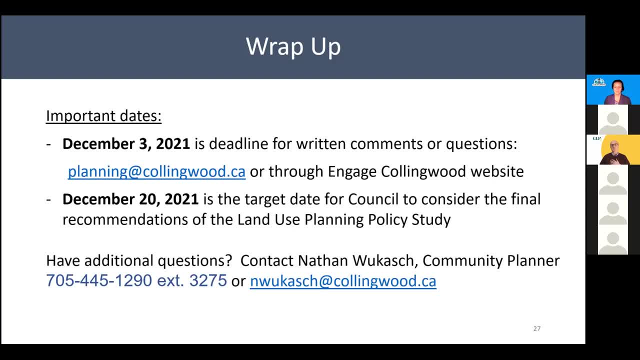 which is greatly appreciated, And, from my perspective, it's been a real pleasure working with all of you. Thank you for the privilege of serving as the independent facilitator for the session. I'll now formally adjourn the meeting And thank you to the various technical and other personnel. 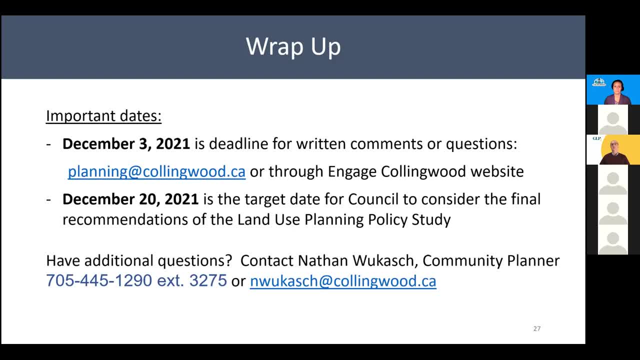 who made the session possible. Please enjoy the rest of your day, Take care, stay safe and goodbye for now. 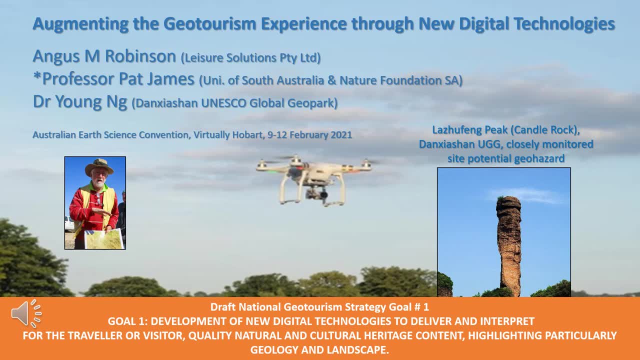 Hi, I'm Pat James. My co-authors and I have been involved since the Adelaide Convention in developing a range of new innovative technology applications to support geotourism interpretation. We had planned to show this at the 9th International Global Geoparks Network Conference in Korea. 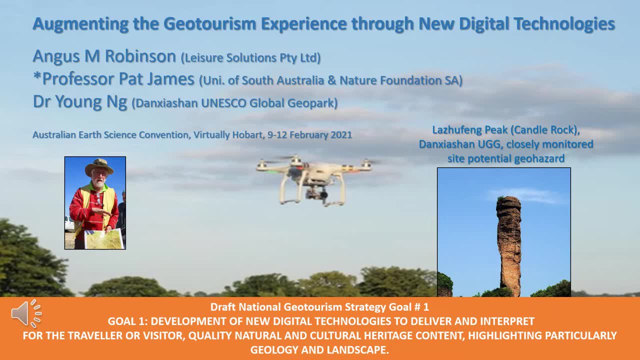 last September, but that was postponed to September 2021, so maybe we'll go there. We also plan to visit Dangxiaxian Geopark in China where Dr Yang is the principal geoscientist pioneering drone use in that geopark. We've also been members of the Australian 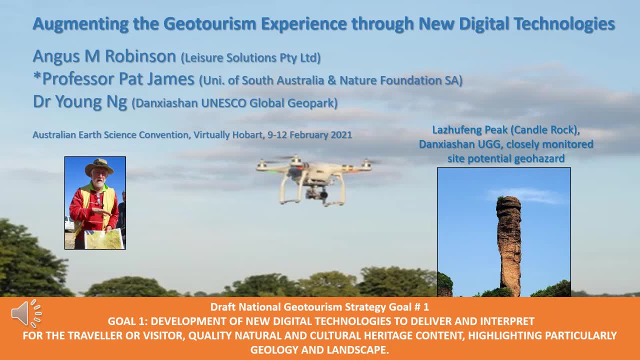 Geoscience Council's National Geotourism Strategy Reference Group, which is coordinated by Angus. This group's just completed its first draft with seven strategic goals, and goal number one is designed to foster the development of new digital technologies, as you can see at the bottom of the slide.